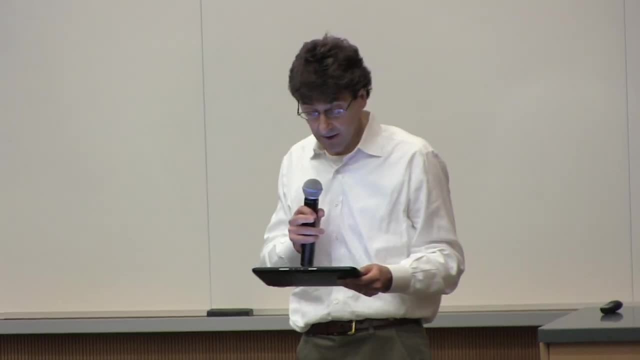 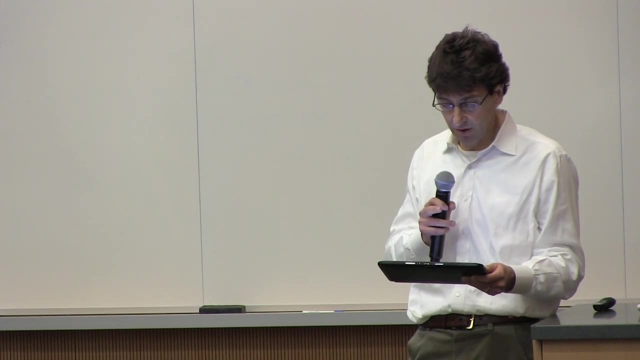 and he was then a postdoctoral fellow at Harvard with Elkham Blount. After that he spent a period of one or two years, I believe, here in Madison working at the Enzyme Institute in collaboration with Harry Lardy. 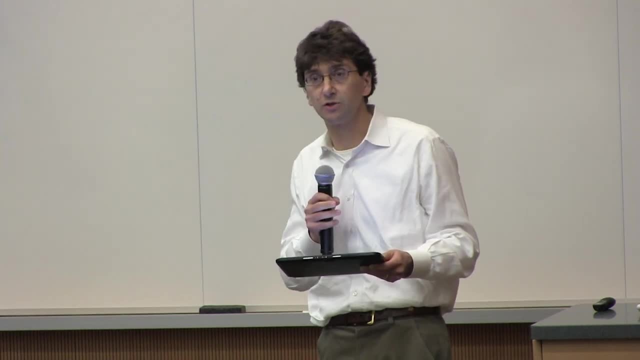 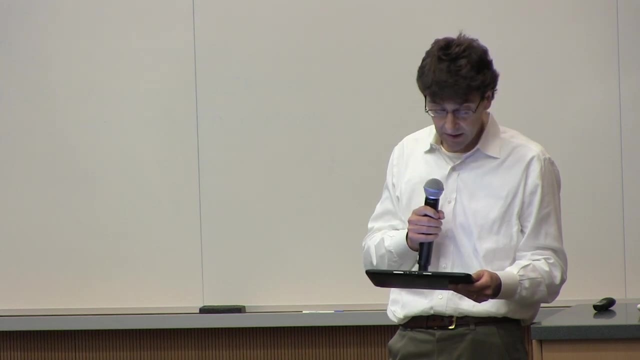 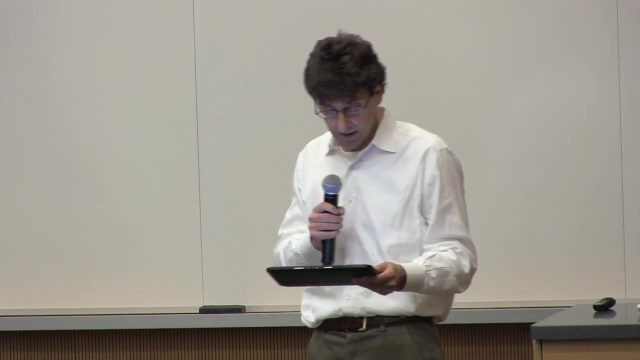 and then left to take his position as an assistant professor, then in Toronto. He has a long list of honors, awards and professional achievements. He has over 250 publications in international journals. He has been president of the American Peptide Society. He has been the editor-in-chief of Peptide Science and in the editorial board of many other journals. 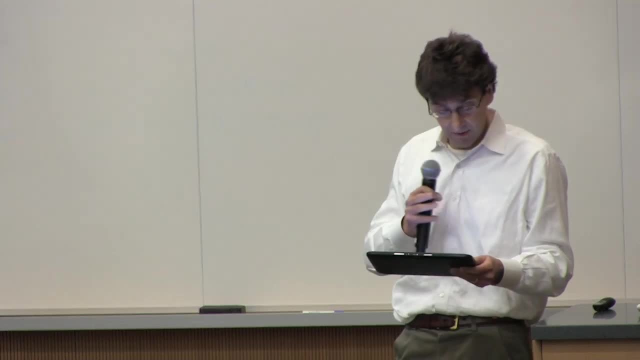 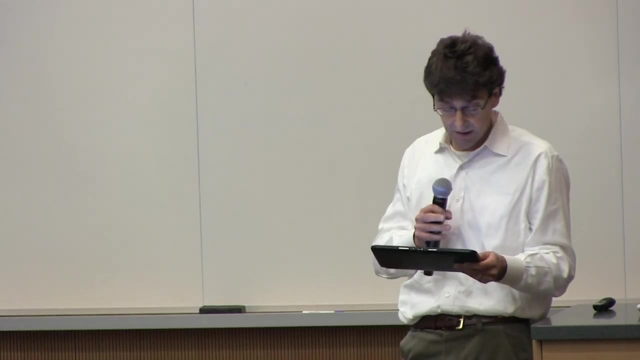 He's a friend of mine. He's a friend of mine. He's a friend of mine. He's a fellow of the Royal Society of Canada. He was awarded the Vincent Duvenger Award for Outstanding Achievement in Peptide Research by the American Peptide Society and the Murray Goldwyn Award for Scientific Excellence. 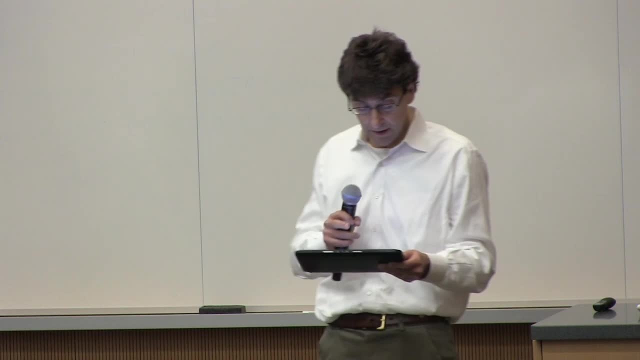 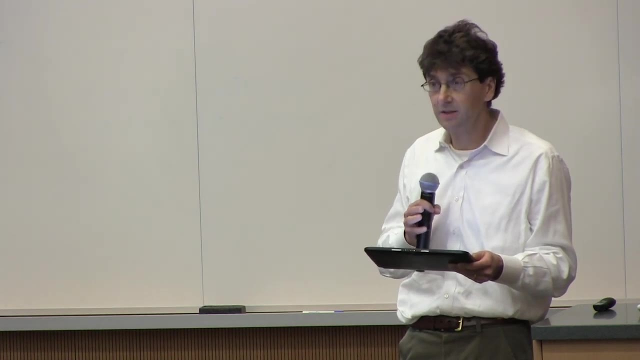 and Mentorship in Peptide Science, and I could go on If I had to define Dr Dieber in a nutshell for those that don't know him very well: he is an outstanding peptide chemist and he is somebody who applies this to understand. 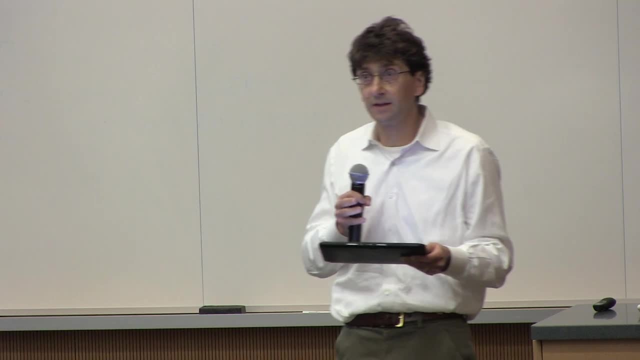 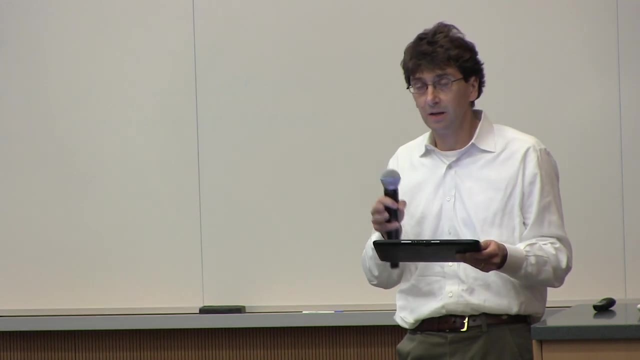 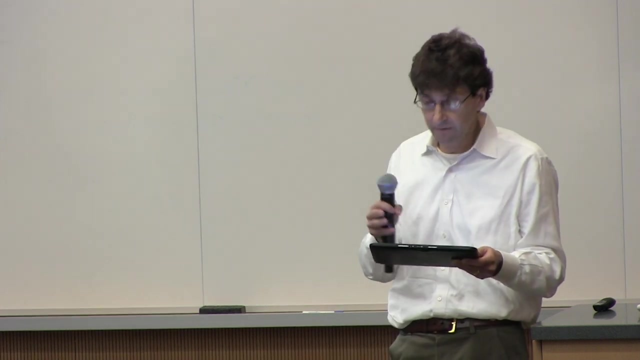 the folding and structure of membrane protein. I feel that he has pioneered. He has been studying factors that drive association and insertion of peptide in lipid, bilayer and detergent, and studying motifs and physical factors that drive this phenomenon, like van der Waals, hydrogen bonds, aromatics. 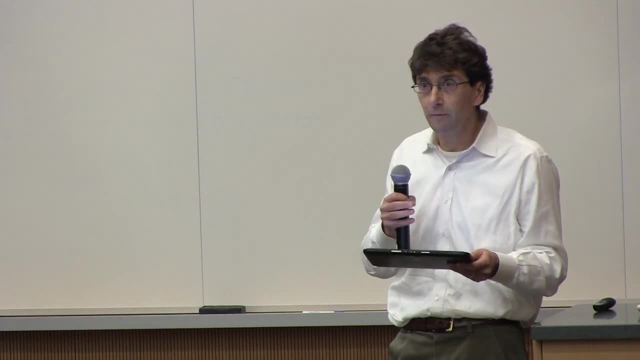 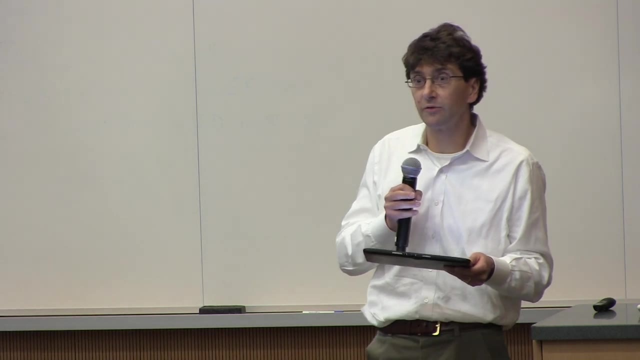 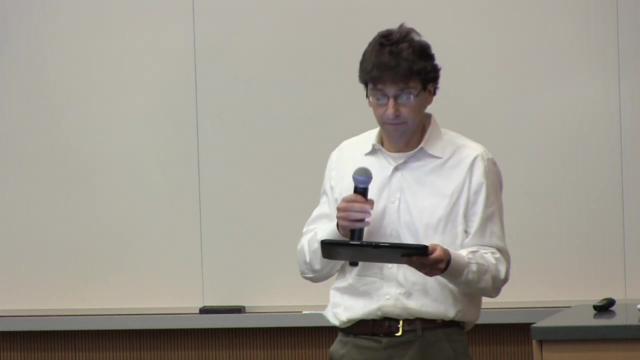 chitin and so on, laying very much a foundation for very much everything that we do in my lab. He has done most of these studies. He's primarily in the concept of biologically important molecules such as CFTIR, which is the chloride channel that causes mutations, cystic fibrosis or viral code proteins. 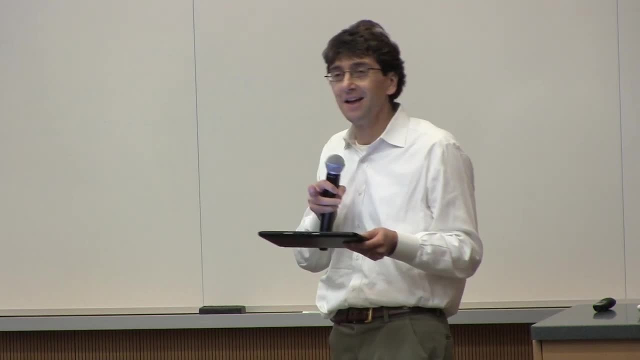 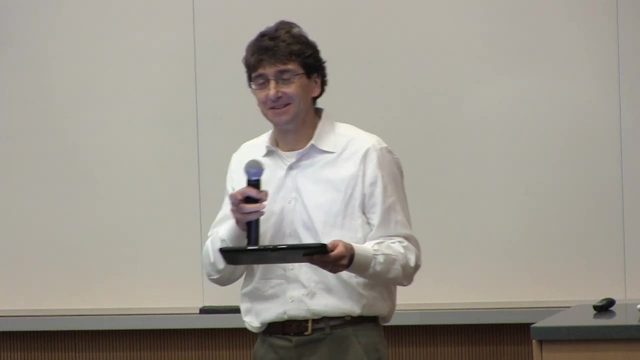 Another interesting fact that I learned from Dean is that he's a recurrent contributor to the New York Times crossword puzzle, which I found very interesting. I think he contributed a couple of years ago- one of the 50th anniversaries of the Beatles right. 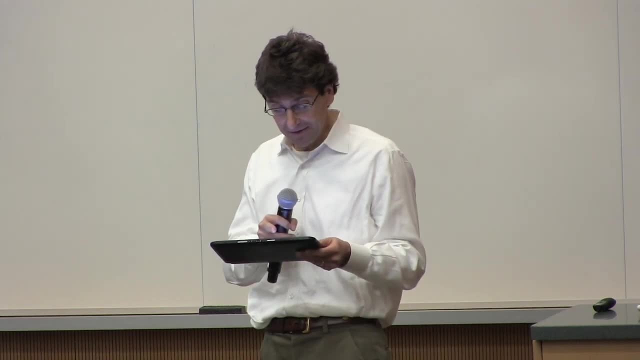 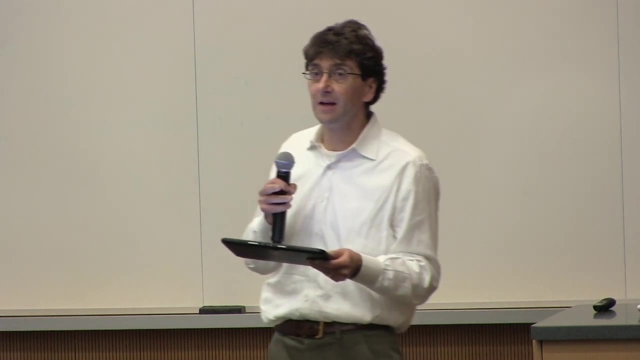 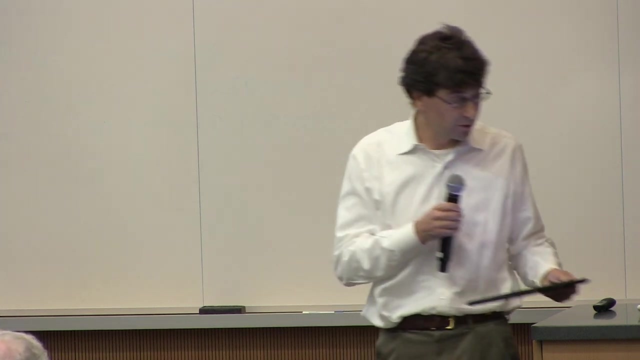 Yeah, recently, yeah, Okay, Today, Dr Lieber will present some work, recent work on a new class of peptide that have some very outstanding properties, especially in light of antibiotic resistance. Without taking more of his time, I would like you to join me to welcome him back to Madison. 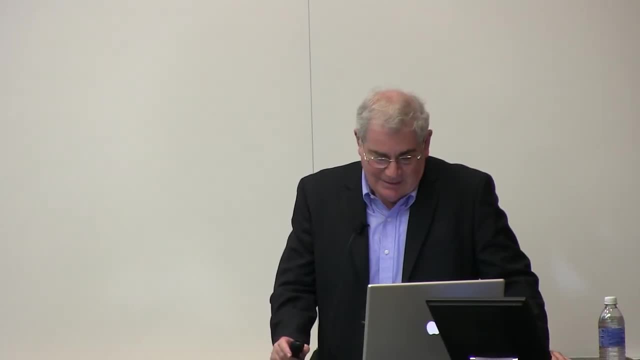 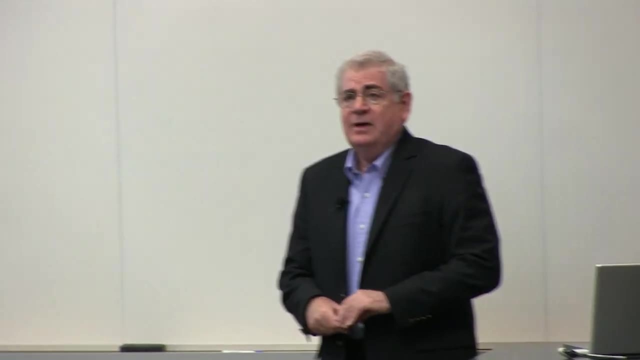 Thanks, Alessandro. That's a beautiful introduction And we'll try- I'm going to try- not to let my Brooklyn accent distract you too much. I'm going to tell you today about, as the title indicates, something about- antibiotic resistance. 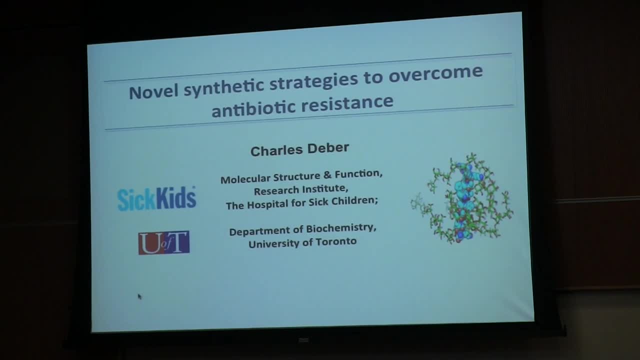 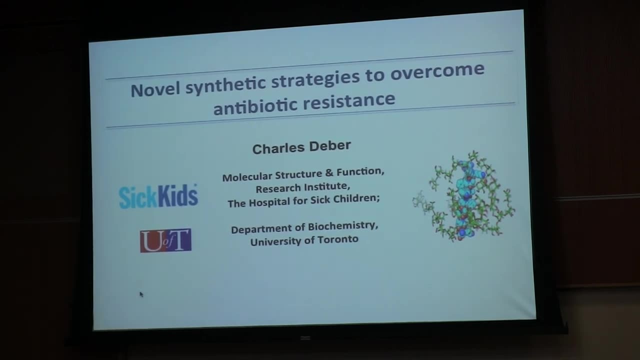 And it's a topic that really came out of all the transmembrane segments and all the peptides and membranes and so on. It's one of these things, curiosity driven. It isn't something like we started out to do, but you will see where it ended up. 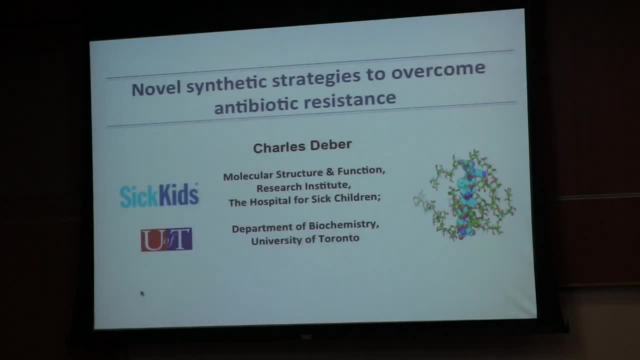 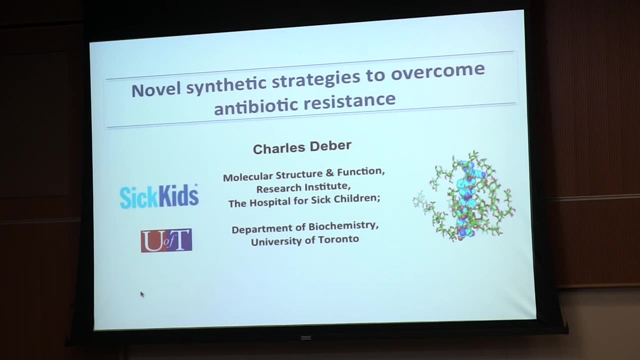 I do want to say a couple of things. First, I'm very honored to be the Gladys Everson lecturer. From what I read about her on the website, it seems she was a pioneer in the importance of exercise and the importance of good nutrition. 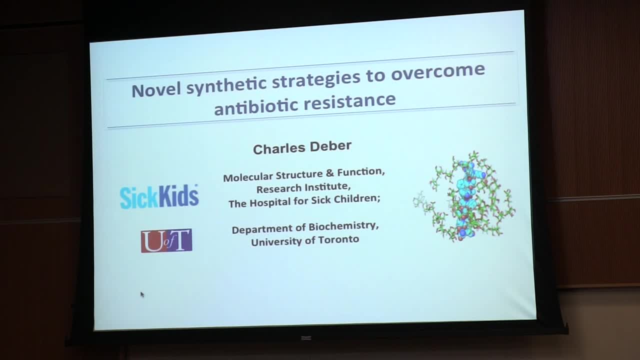 And those topics of course are very current today and I'm sure she would relate to that very favorably. As far as our experiences in Madison, my wife and I did come here from Boston, myself from Harvard, She from Alabama. 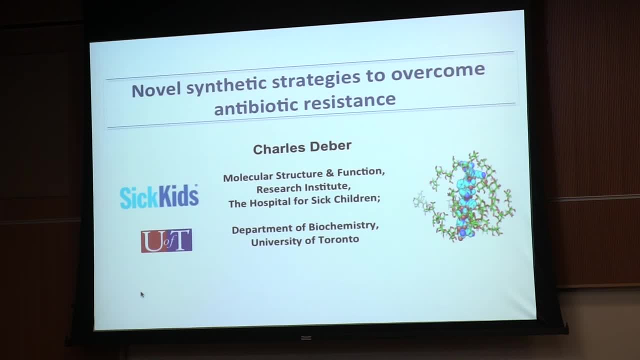 From MIT. She was an assistant professor in the political science department and I was a research associate with Henry Lardy in the Research Institute. We were here overall two or three years. She is Canadian and eventually we got two permanent jobs in Toronto, but we certainly remember our stay here extremely fondly and it's just great to be back here. 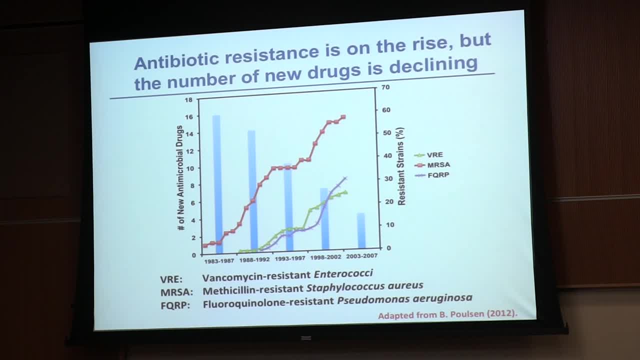 Well, most of you know that The bacteria are very tough customers and there's been a lot of negative things in the news about our fight to control them. The number of new antimicrobial drugs these blue bars here have been heading down. 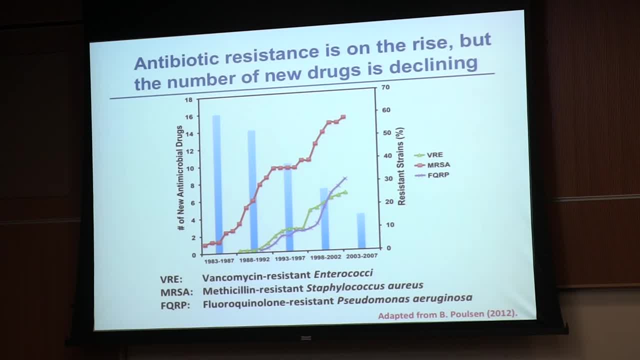 And, meanwhile, the number of resistant strains of these bacteria, including ones that are quite well known: enterococci, the MRSA, pseudomonas aeruginosa, which is the main bacteria. The question is, of course, what are we going to do about it? 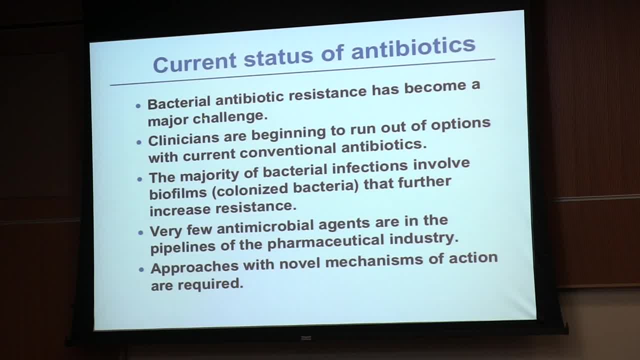 So bacterial antibiotic resistance is a major challenge and clinicians are beginning to run out of options actually with the classical conventional antibiotics. The majority of bacterial infections involve biofilms, sort of colonized bacteria, and I'm going to get into that in a little while. 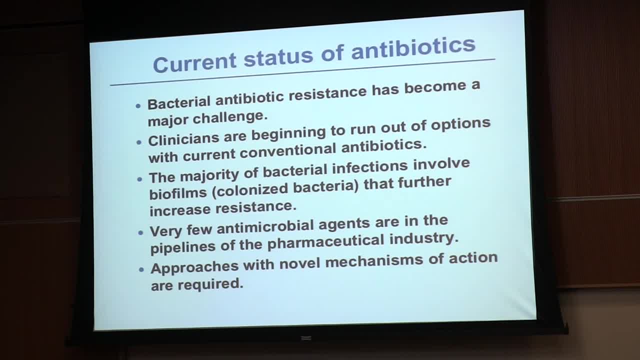 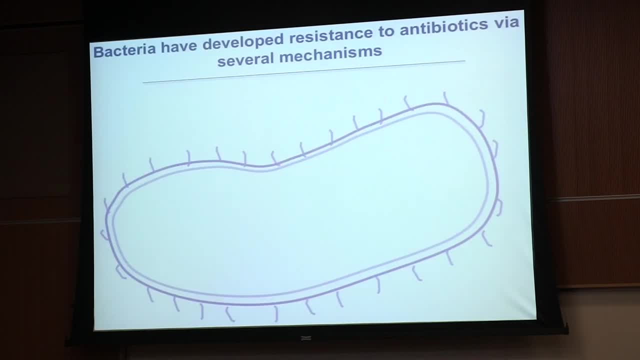 And very few antibiotics are going to be used. antimicrobial agents are in the pipelines, as we just saw, So approaches with novel mechanisms of action can certainly be used. So why are bacteria so good at this? How do they fight off all the drugs that we give them? 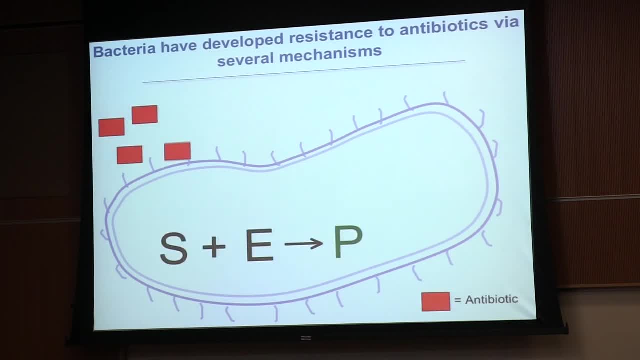 Well, we can look at this kind of schematically. If we have an antibiotic, for example, it gets across the bacterial membrane, It combines with an enzyme and it inhibits the action of that enzyme. So all of a sudden, the bacteria aren't inhibited anymore. 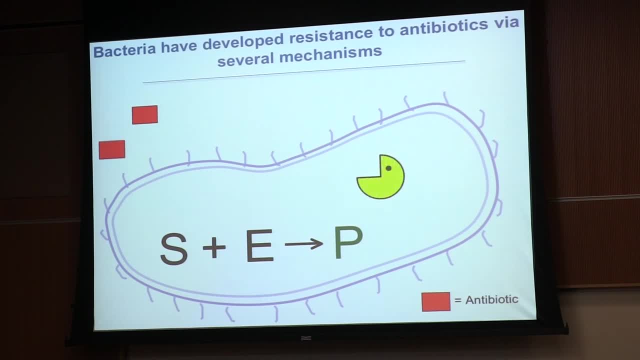 They just make a slightly different enzyme. There are other factors and enzymes in the bacteria that have power to just chew up just about anything we do, And there are bacterial pumps, these so-called small multidrug-resistant proteins that are in the bacteria. They're in the membranes of the bacteria. 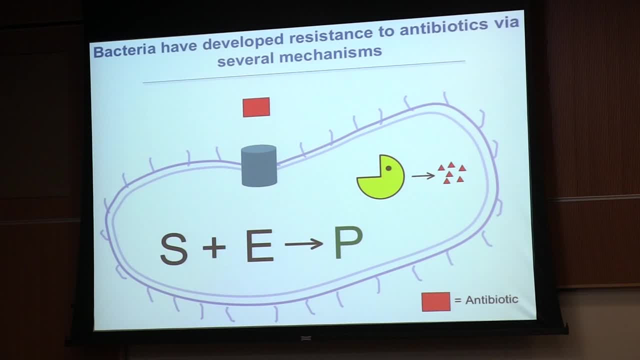 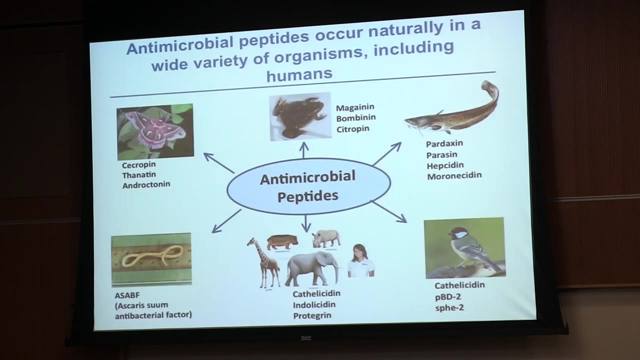 And if you give the bacteria a drug, it just pumps it right out pretty efficient. So what are we going to do to combat these types of mechanisms? So, since our work in the lab is focused on peptides and proteins and membranes, we're going to look at the bacterial membrane. 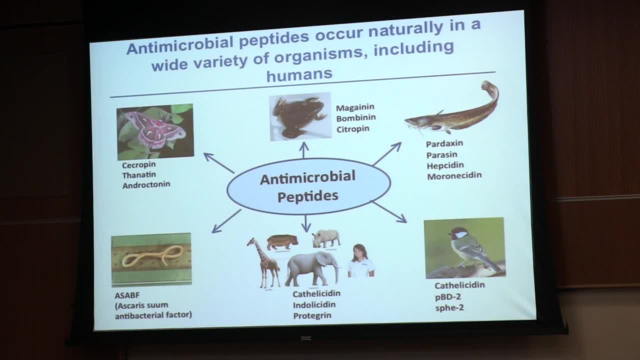 from a couple of different points of view. Now, in order to fight bacteria, we have to fight off the bacteria. It's not just the antibiotics that we give them. Our body also tries to fight off the bacteria with antibiotics And most organisms, everything from butterflies to frogs. 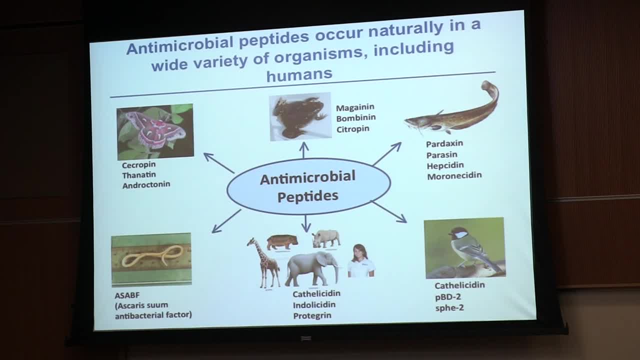 and birds and mammals and so on. they all secrete some kind of native peptides in conjunction with the immune system to try to fight off the bacteria. And most of these peptides, which have, I think, a lot of them, names like meganin and sucropin, indolecidin, protogrin, 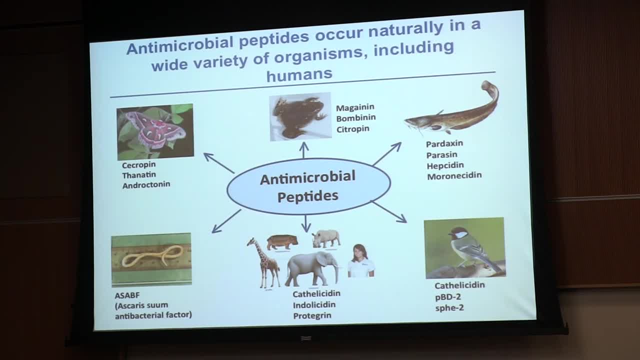 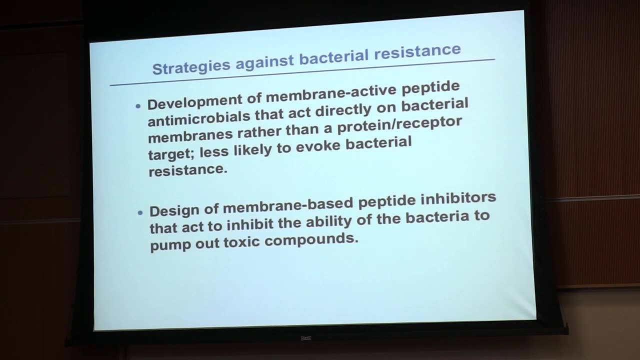 Some of these are names you may have seen And these are peptides that are basically membrane active. They just go to the membrane of the bacteria And they don't have any specific target, And the idea is to get into the membrane and just disrupt the bacterial membrane. 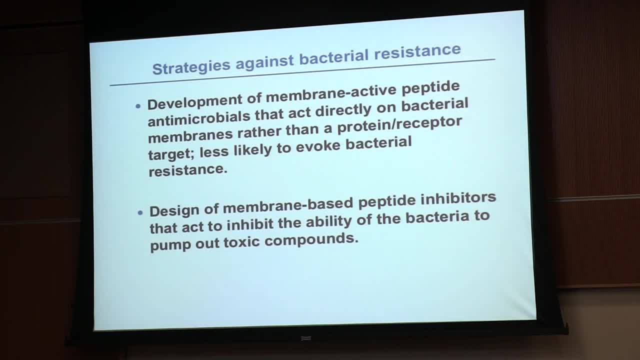 So what I'm going to tell you today is two themes, two strategies that we've tried against bacterial resistance. The first one. The first one Is the development of membrane-active peptide antimicrobials, as I just mentioned, that act directly on the membranes. 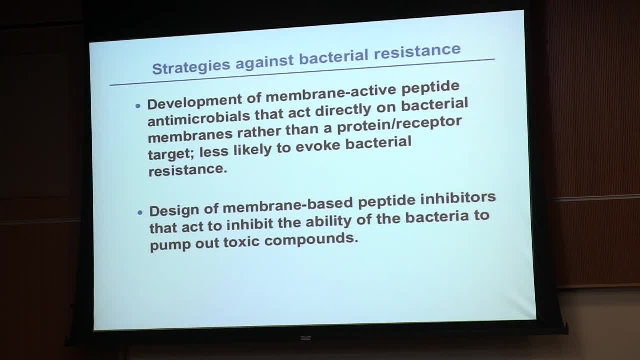 rather than on some sort of protein or receptor target. This is less likely to evoke bacterial resistance. And even though all the organisms do this, it's obvious that, whatever are the secreted peptides, they haven't been enough to kill all the bacteria. 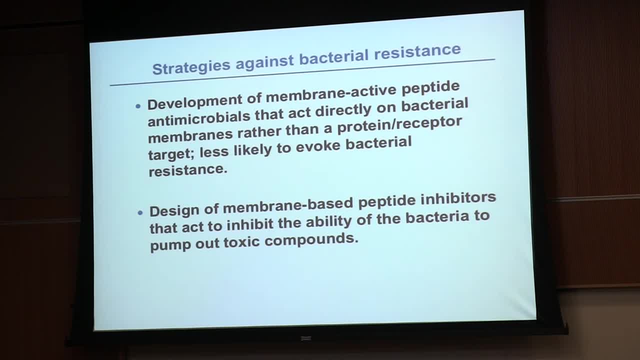 So maybe there's some new twist on it that we could think of. And the second thing We're going to talk about in the last part of the seminar today is the design of membrane-based peptide inhibitors that actually inhibit the ability of the bacteria to pump out the drugs. 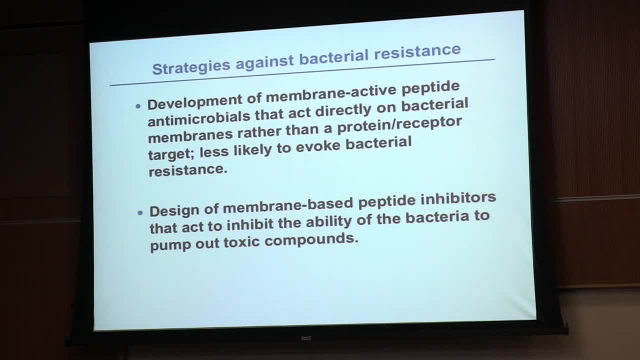 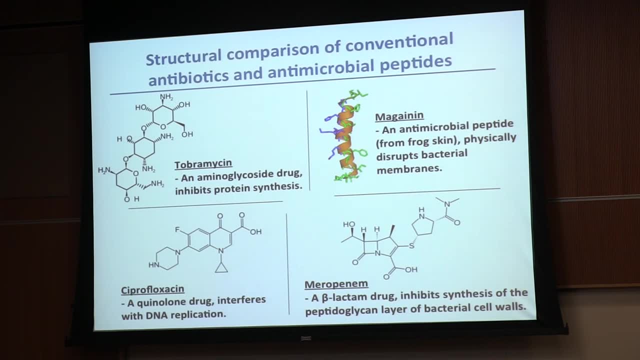 So we'll look at those two things And we'll see what we can do in the laboratory to get at that. So if we look just for a minute at a structural comparison between so-called conventional antibiotics and what antimicrobial peptides might be like, 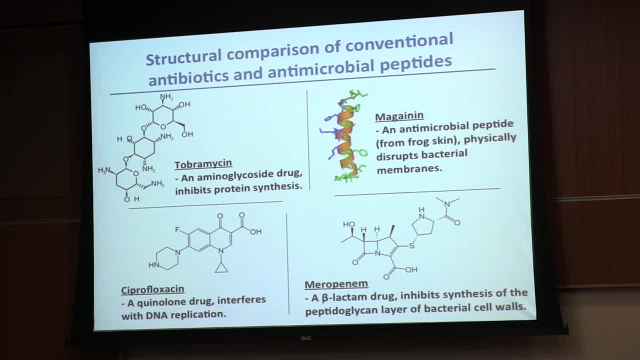 you can see just at a glance that some of the well-known antibiotics like toto, tobramycin and aminoglycoside. Ciprofloxacin is a quinolone drug. This one called meropenem is a penicillin derivative. 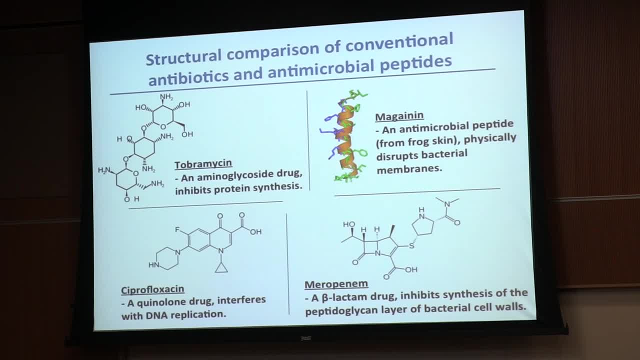 one of these beta-lactam drugs. They each have some sort of target in the bacteria And these are the drugs that bacteria develop the resistance to. So, on the other hand, meganin, as I mentioned before, is an antimicrobial peptide from frog skin. 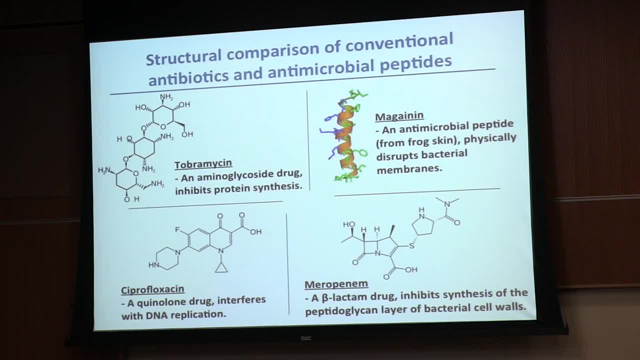 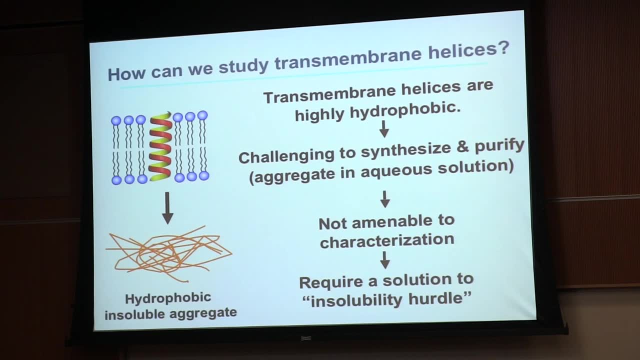 And it acts by a mechanism of physicality. It's actually disrupting the bacterial membranes. So it's the meganin is the one that we're going to try to model ourselves after. So if we want to make peptides like meganin, that 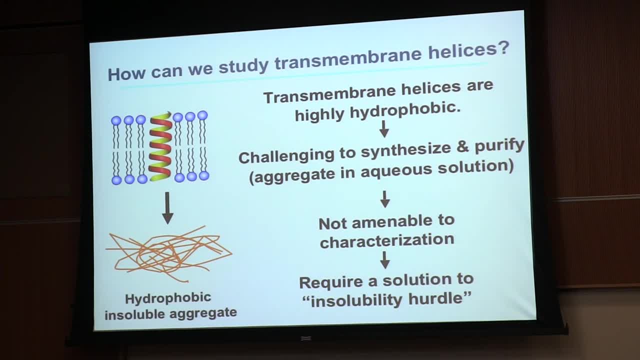 get into bacterial membranes. there is a practical side to all of this. They are very insoluble in water, And they should be, because they're supposed to be in membranes and not in water. So we have to think of some way to make membrane active peptides. 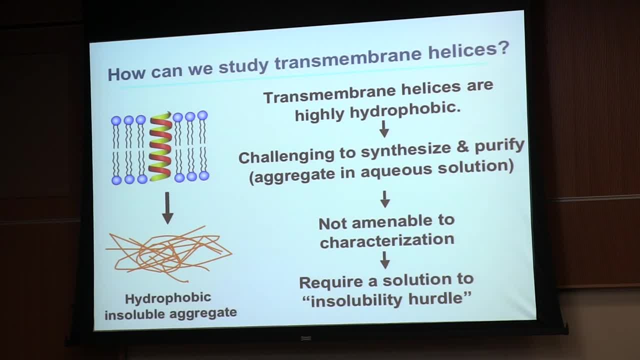 make them soluble in water and be able to make them, purify them and characterize them. So transmembrane helixes, as they're called, or TM for transmembrane, highly hydrophobic. It's challenging to synthesize them. 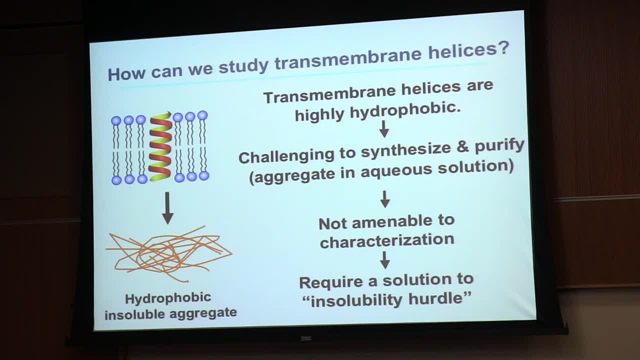 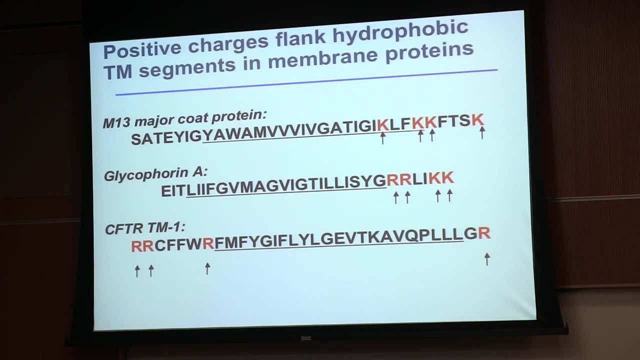 They're not amenable to characterization And we required a solution in the lab to overcome what's been called the insolubility hurdle. So we borrowed, basically, a feature from natural transmembrane segments. You can see these ones from native proteins like M13, glycophorin, CFTR. 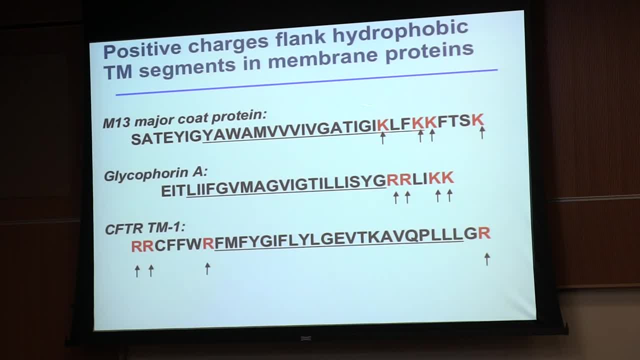 This is cystic fibrosis protein. When they exit from the membrane, they usually exit with a bunch of positive charges, often lysines, sometimes arginines, Sometimes they're on one side concentrated here, Sometimes they're on both sides. 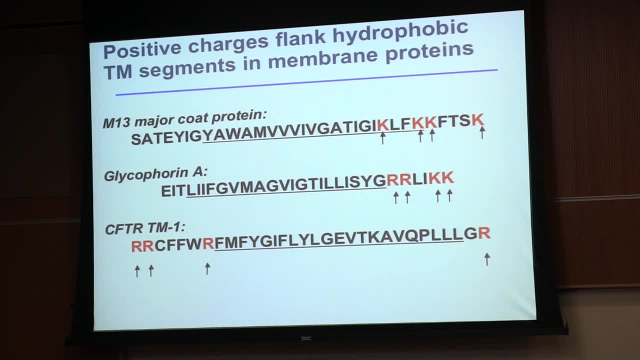 So basically, the idea is we would make hydrophobic peptides and we would make sure they have enough positive charge in order to help them be water soluble And then, when they approach the membrane, they use their hydrophobic portion to do the interaction with the bacterial membrane. 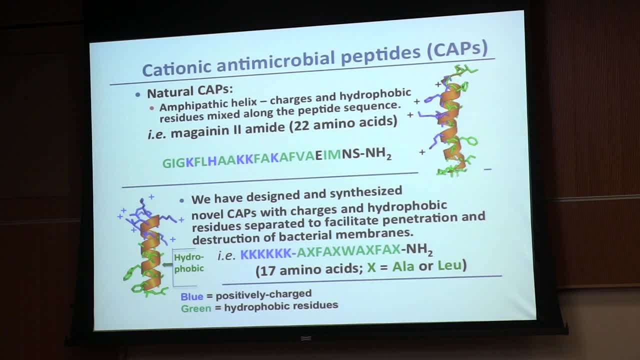 So this is what it looks like in a little more detail. We call these cationic antimicrobial peptides, or CAPs, So I'm going to use that name from now on. So natural CAPs like meganin- it's one you just saw from the frog skin, amphipathic helix. 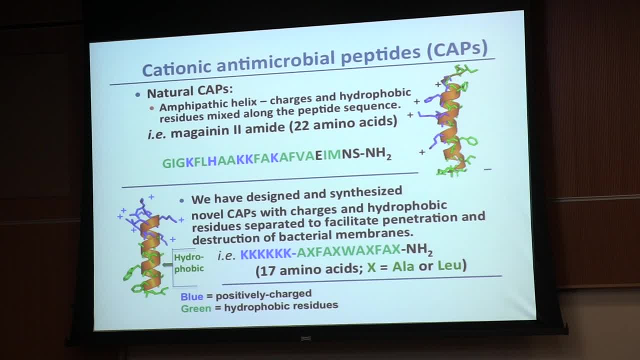 And it means that the charges, the positive charges and the hydrophobic parts, are inter-dispersed all throughout the sequence. So when you're doing a test, you're going to want to do that, And then, when you're doing a test, you're going to want to do that. 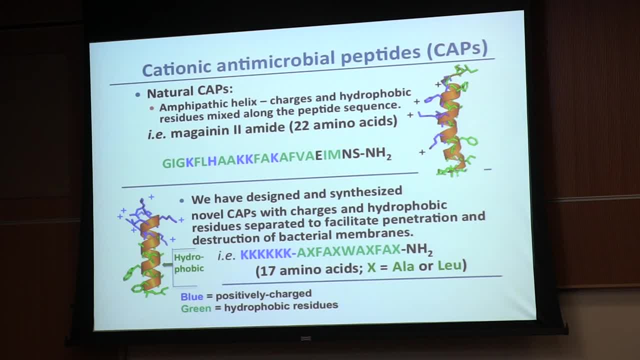 So when you're doing a test, you're going to want to do that. So when you're doing a test, you're going to want to do that. So when you fold this up into a helix, you've got one face that has just positive charges. 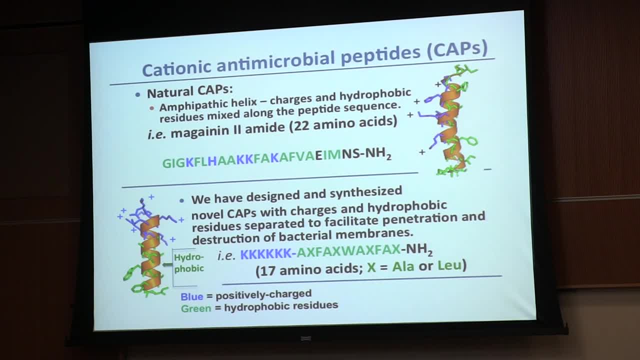 the other face that has just hydrophobic residues. This is the sequence: meganin. You can see the blue residues are the lysines, histidine. So when this folds up into a helix, you can see. the positive charges are on one face. 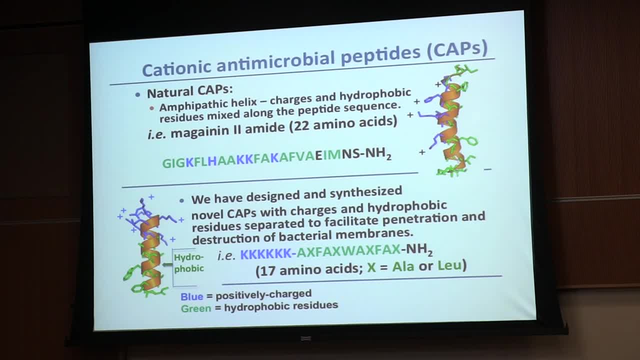 and the green hydrophobic residues are on the other face. So if this is attracted to a bacterial membrane, the positive charges go to the phosphate group and the head group And then the other residues like phenylalanine or leucine. 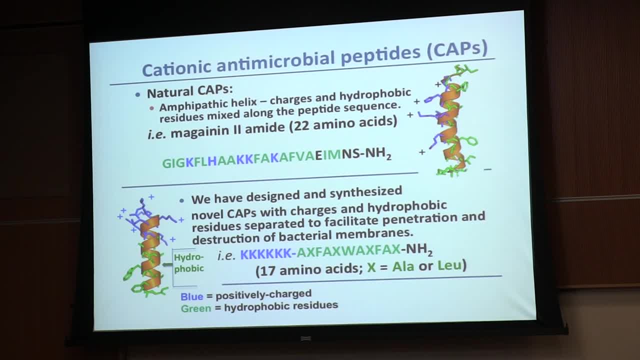 point down into the membrane. We designed and synthesized a novel version of that, But what we did is we separated the charges and the hydrophobic residues, And this is designed anyway to facilitate the penetration and destruction of the bacterial membranes. So here you see a model of this. 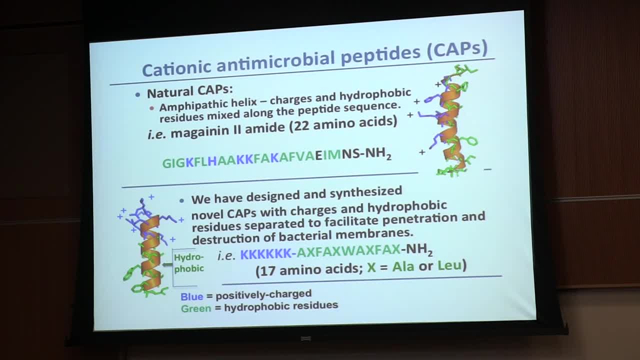 And you notice all the lysines are all grouped together on one side And then you have an uninterrupted hydrophobic stretch. So the best ones of these we found to be 17 residues, 6 lysines and 11 hydrophobes. 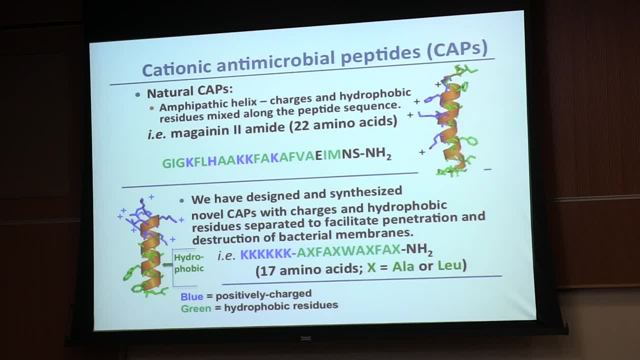 And the best ones that I'm going to talk about today have this kind of general structure: AXFAXW. We always put tryptophan in as a fluorescent marker, AXFAX, so the F comes the 6F17,. are we calling it that? 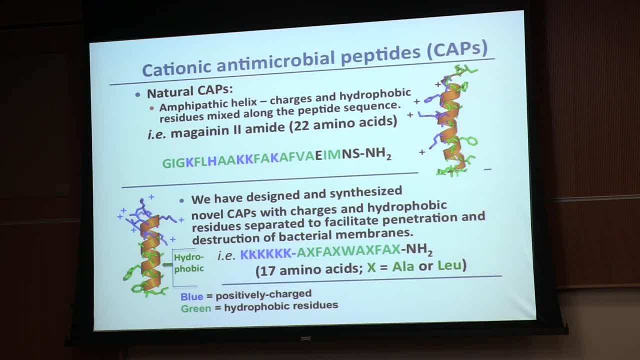 I don't see that here. We're calling it 6KF17.. And there's 17 amino acids And X can be a mixture of alanine or leucine And that depends on how hydrophobic you want to do it. 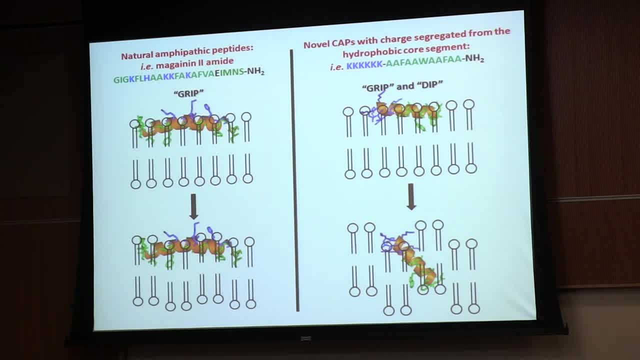 So we thought that the advantage of this would be, in contrast to the natural amphipathic peptides- if you take a bacterial surface, just as I mentioned, that the peptide can be gripped into the surface, But it's held there. 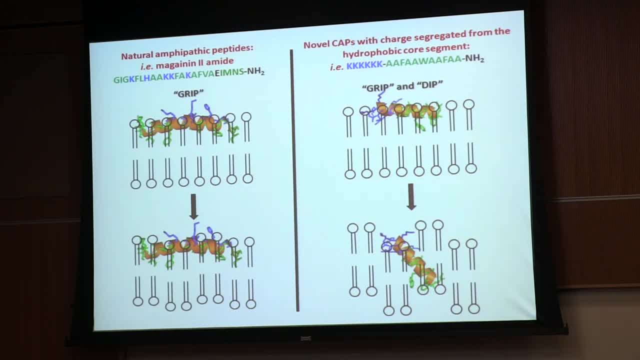 It's held there by the lysines and it can't get down too far. This is the idea, Whereas with our peptides, which we call, instead of the grip, we call it the grip and dip mechanism, where we have the peptide in the surface. 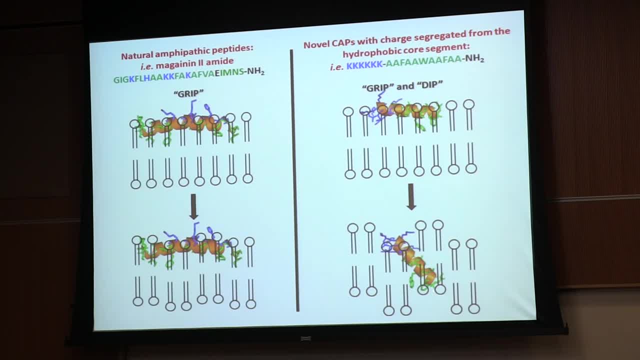 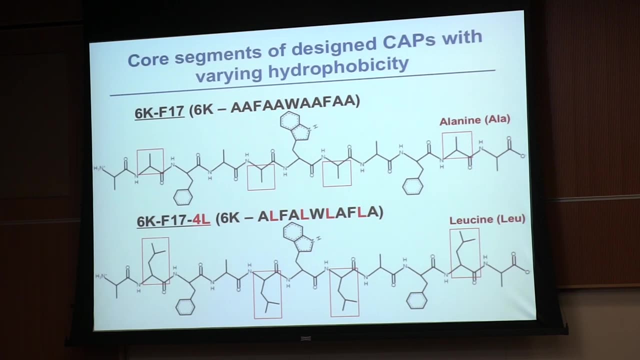 of the bacterial membrane, But then the lysines stay up here and we think that the hydrophobic part can penetrate and be more effective at disrupting the membrane. This is, of course, a dramatization, And it's at least the thought behind the experiments. 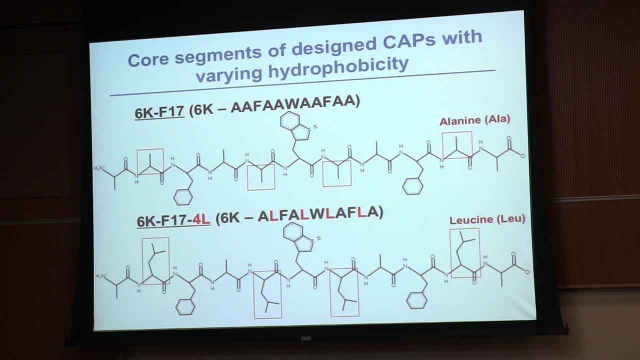 So coarse segments, the 11 residues can vary And the hydrophobicity- if you're talking about inserting something into a membrane- is a huge factor. It has to do with how it interacts with the lipids. It has to do with propensity to partition from the water. 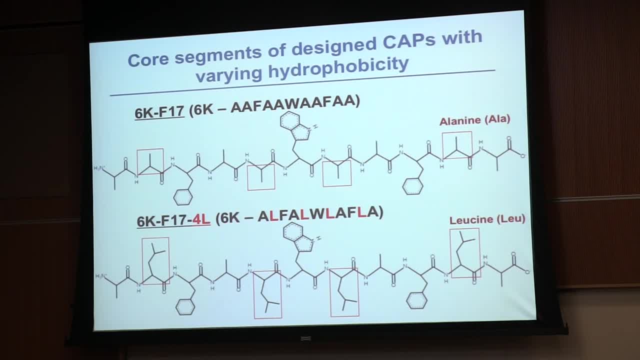 into the membrane, Several factors going on. So this is the chemistry of this, what these peptides actually look like. If you put the lysines off to the side, you can see you can have alanines in this position: phenylalanine, tryptophan. 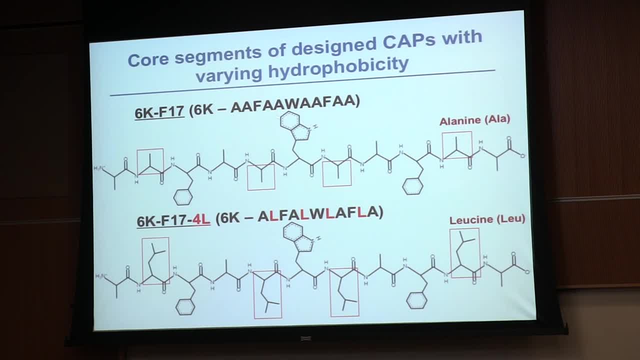 So what I'm calling 6KF17 is this one: AAFAA, WAAFAA. So that's this one, And you can improve the hydrophobicity by putting leucines in instead of alanines. So in some positions we put in four leucines. 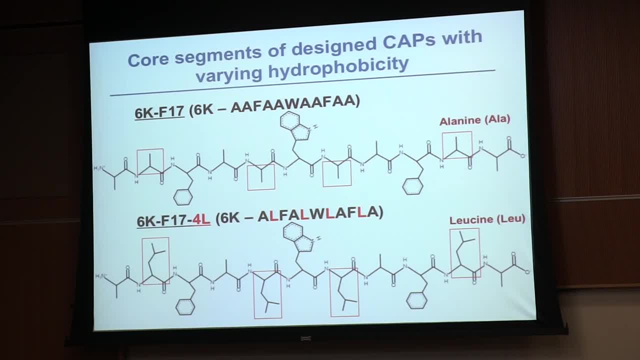 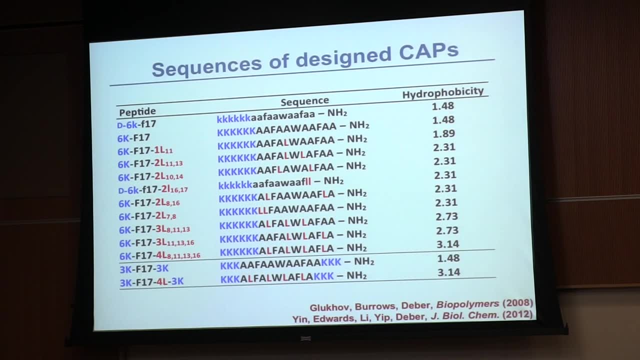 in this particular example. So these are where they substituted for alanine. So the 4L version of this is going to be considerably more hydrophobic. So even on this simple design, really you can make millions of different combinations and derivatives. 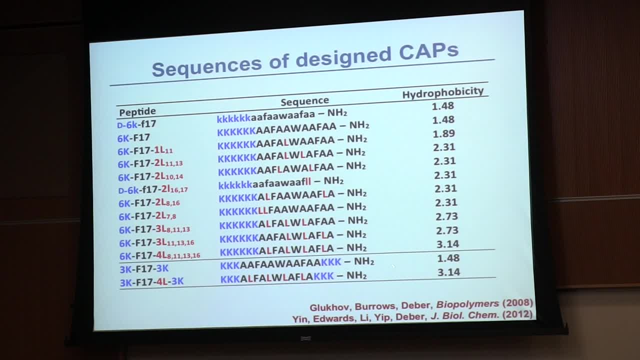 You can put the 6Ks on one side or, if you want to, you can mix three and three just to test out the importance of gathering the charge together. You can put no leucines, or two or three or four. 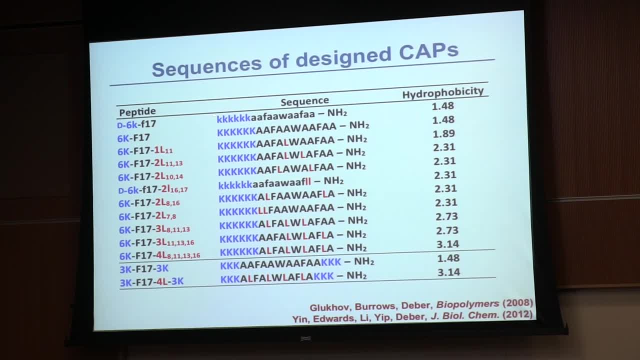 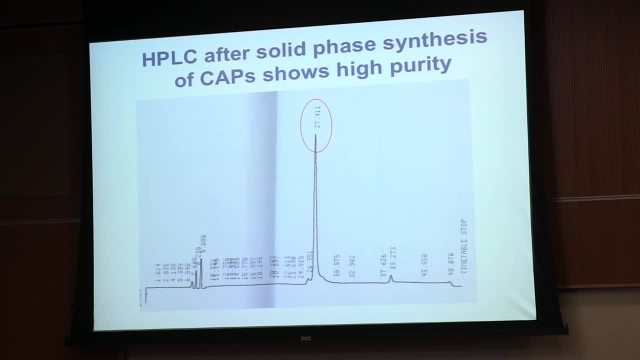 You can put D residues, As in this one, in the lowercase letters And you get different hydrophobicities for these different examples We make each one. Do it by solid phase peptide synthesis. We purify them by HPLC. 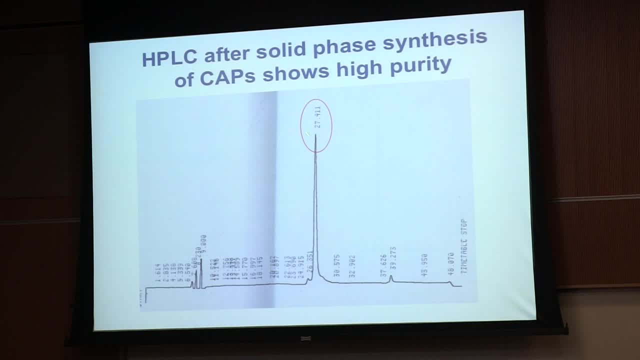 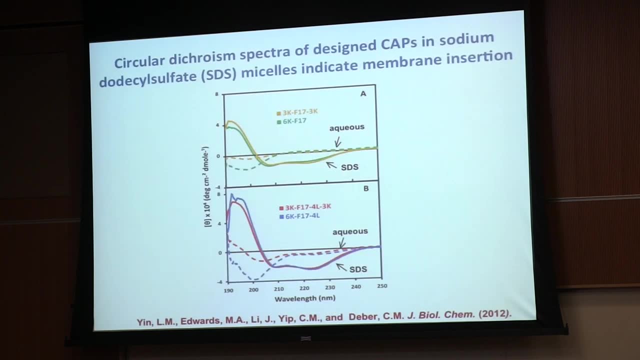 We check them out by mass spectrometry to make sure we have exactly the right compounds. So these are all relatively straightforward and easy to make. Another thing that's very important is you have to show that these will. instead, you know that these will insert into a membrane. 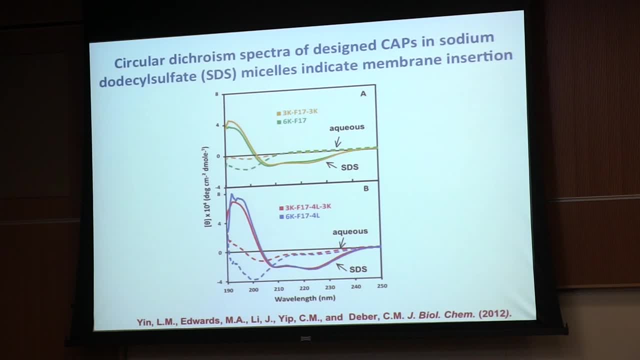 and be helical, because that's the trick. And in fact, if you try this in a detergent like sodium dodecyl sulfate, the most commonly used in the lab for this SDS, you can find that the 6KF17 gives this nice helical value. 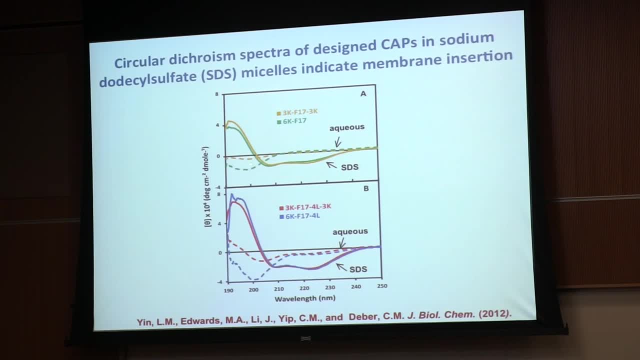 when it's in SDS, but it gives a random coil- That's the green dotted line here- when it's in a water phase. So it's water soluble. but when you put it in the presence of SDS it enters the membrane and it becomes helical. 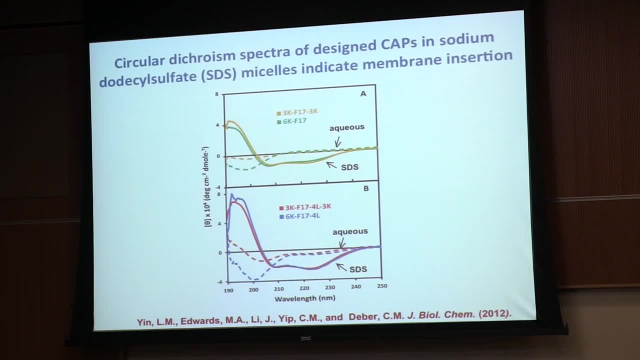 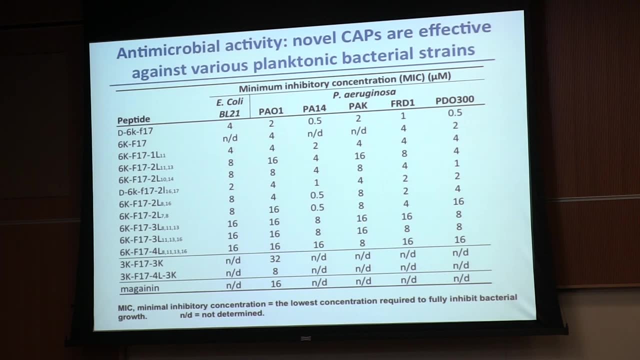 So that's exactly what we want to happen, And in fact, the four-leu version of this does exactly the same thing. So now this is one of these one-day-in-the-lab things. This goes back quite a few years now. 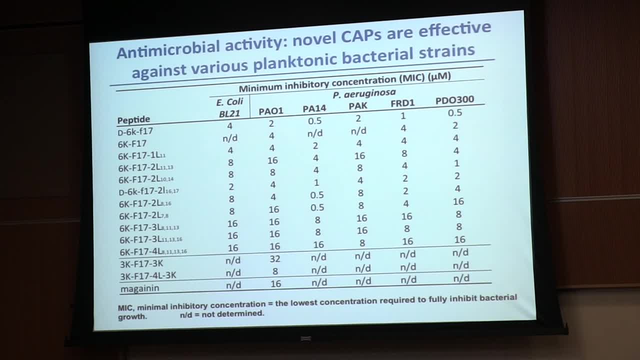 We were aware of all the natural caps that humans and animals secrete, and we realized some sort of- you know- a relationship between our peptides and those In those days. we had longer ones and shorter ones and all, So we decided to test them against bacteria. 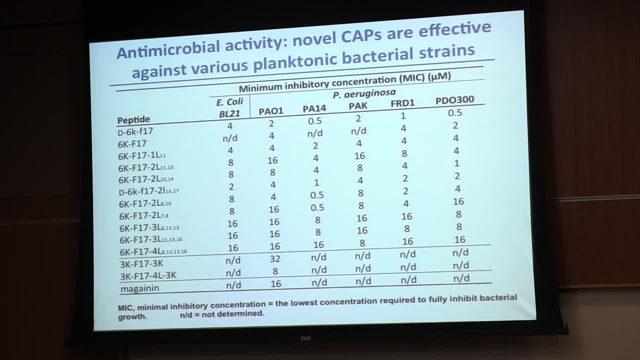 just to see if they had any antimicrobial activity. And this is without reading all the numbers, just to point out these ones like 6KF17 and so on. if you test them in E coli, you get these so-called MICs. 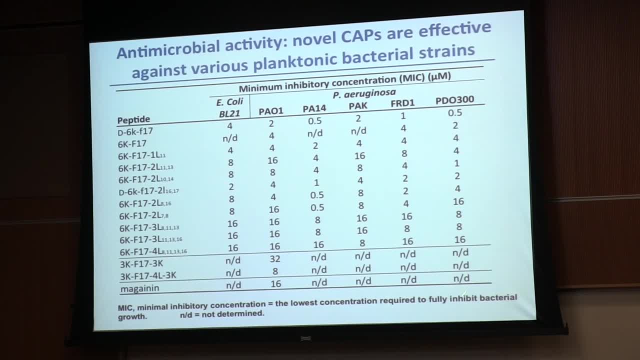 they're called minimum inhibitory concentrations, to fully inhibit bacterial growth, and there's very established protocols for carrying this out. The main thing is you want very low numbers. If you have two and four and one and 0.5, you're doing pretty well. 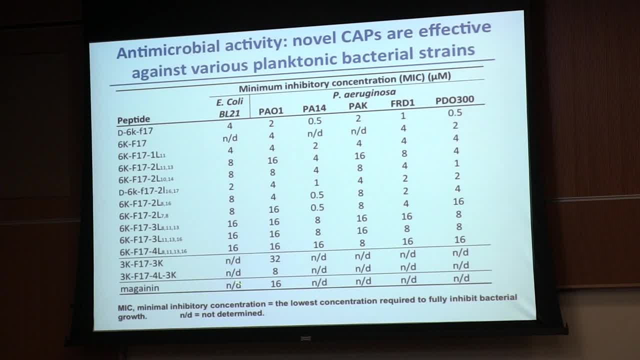 because in this assay the meganin is up at 16. So we are in many cases even better than the natural one, as in all these different- These are different strains. PA stands for Pseudomonas origanosa. 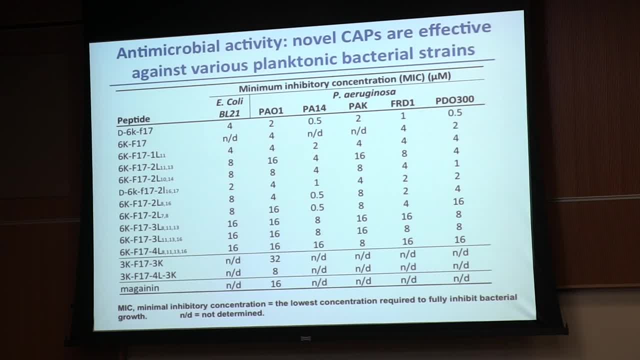 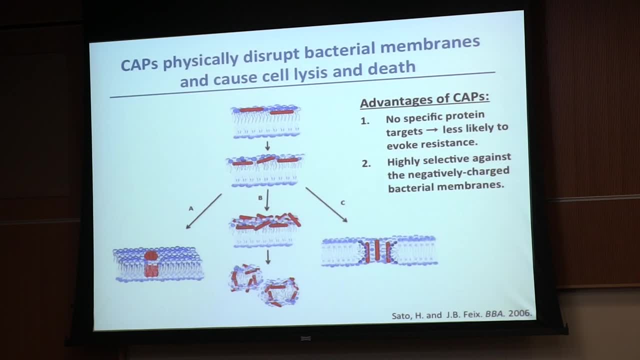 I'm going to come back to that. These are some of the strains that you get from cystic fibrosis lung tissue. So CAPs physically disrupt bacterial membranes. They cause cell lysis and death. The advantages are: no specific protein targets, less likely to evoke resistance. 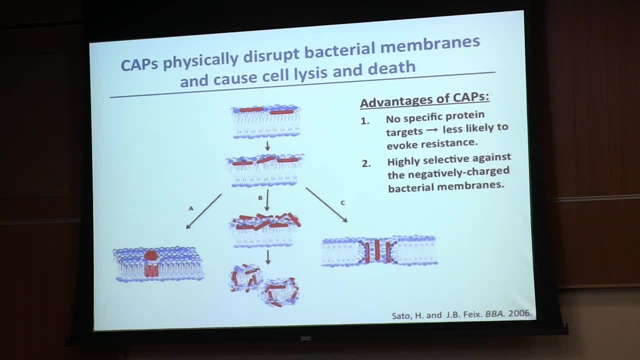 But here's another very important thing: They're highly selective against the negatively charged bacterial membranes, And when you have negative phospholipidase, phospholipid head groups and lysine-rich peptides, they are attracted to each other, sort of like an electrostatic complex. 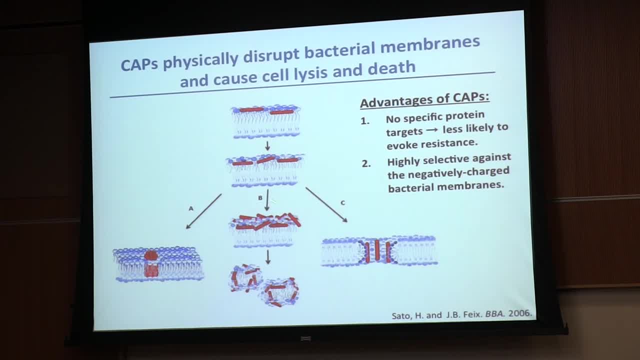 And, although the mechanism isn't really 100% proved, people talk about this in terms of the carpet mechanism, where the peptides accumulate on the surface and then they eventually just overwhelm the membrane and disrupt it. So this is sort of the carpet mechanism. 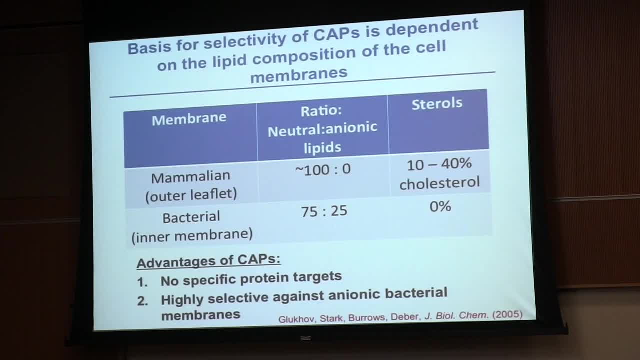 in combination with the grip and dip mechanism. So it's interesting to point out that bacterial membranes are highly anionic, but mammalian membranes, for example, the erythrocytes in our blood cells, for example- those are neutral. They are what's called zwitterionic. 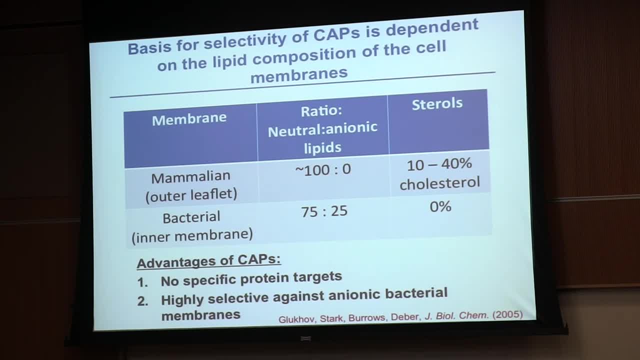 It means they're net neutral. They have a positive charge in the head group and some anion from the phosphate, but they end up being neutral. So this is a very good thing when you're trying to, you know, devise new drugs. 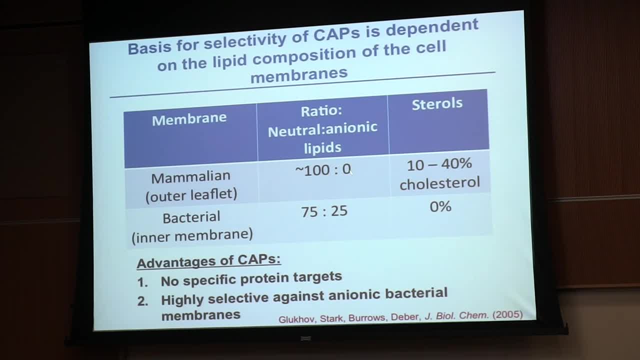 The mammalian outer leaflet is 100% neutral lipids. The bacterial inner membrane 75,, 25,, 25% anionic. They are also different in terms of mammalians have cholesterol. There is no cholesterol in bacterial membranes. 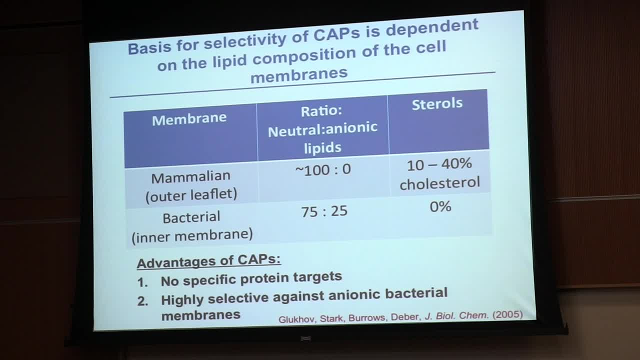 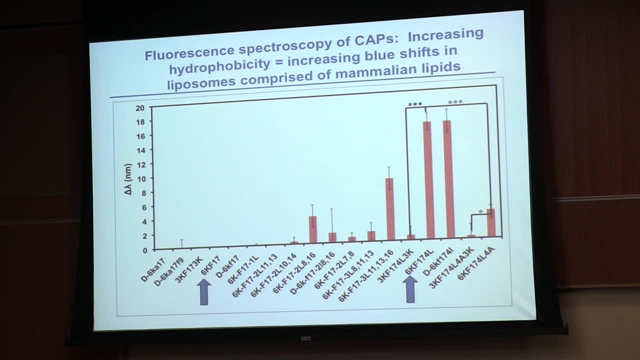 but because they're positively charged. our caps are highly selective against anionic membranes. So you can see this in a couple of different ways If you just do fluorescence studies on the compounds and just look for the blue shifts. and here what we did, is we incorporated or sonicated? 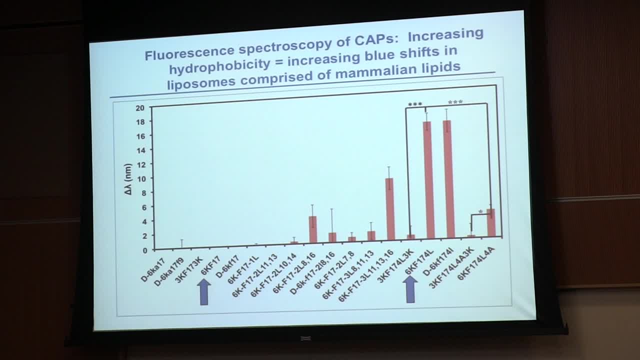 our peptides into liposomes that are made up of just the mammalian lipids. So these are all the net neutral lipids And you look at some of the compounds I showed in that list before you see the 6KF17 has no blue shift. 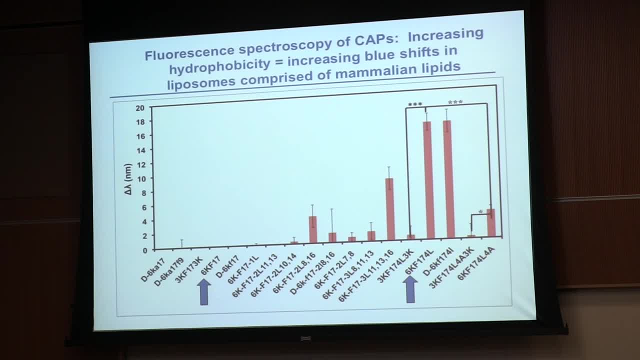 And the blue shift is characteristic of putting tryptophan in a more hydrophobic environment. So these ones down here, 6KF17 and so on, no blue shift. so that tells you that they're not entering the membrane in the mammalian types. 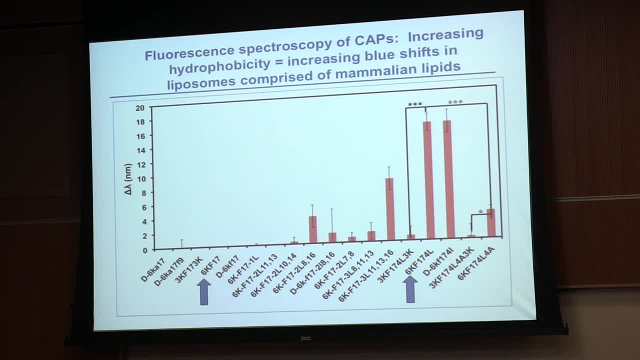 And whereas if you start increasing and putting more leucines, these 4Ls, into here, all of a sudden you're getting huge blue shifts and that means that the peptides are directly entering the membrane. So if this happened to an erythrocyte, that wouldn't be a good thing, because if you want a drug against bacteria, you don't want it to hit the host. also. There's a couple of ways to look at that here. Look what happens if you add caps to some bilators. 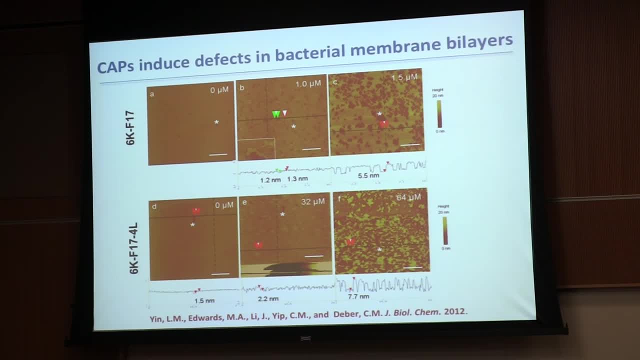 that have been painted onto a face here, Just the tiniest little bit, 1.5 micromolar, and you've already completely disrupted the bacterial membrane. And the 4L compound does that also, And I don't have the slide here. 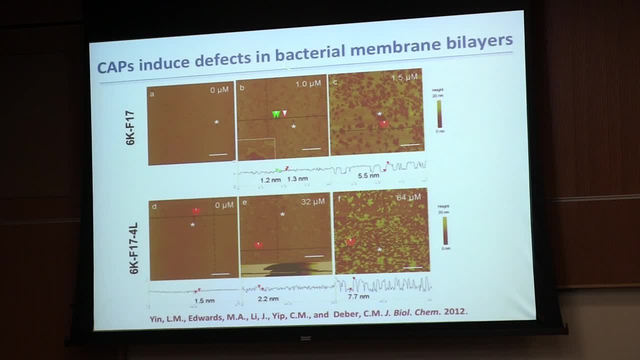 but if you try this same experiment with a mixture of mammalian lipids instead of bacterial lipids, it looks like this: It's like two things that just simply just don't see each other. So this is a very, very powerful cap at disrupting bacterial membranes. 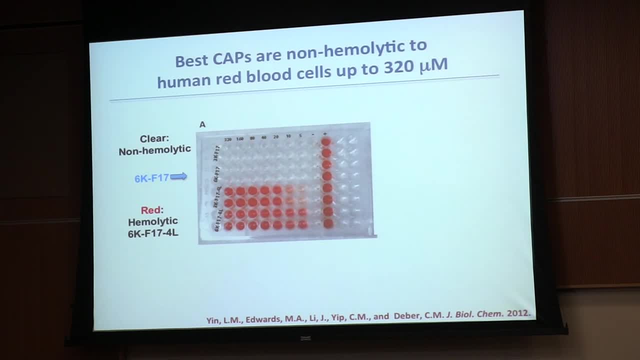 And this is kind of the biology proof here, if you will. The best caps are non-hemolytic to human red blood cells up to 320 micromolar. So you mix the caps with suspensions of red cells. If they get hemolyzed the hemoglobin comes out. 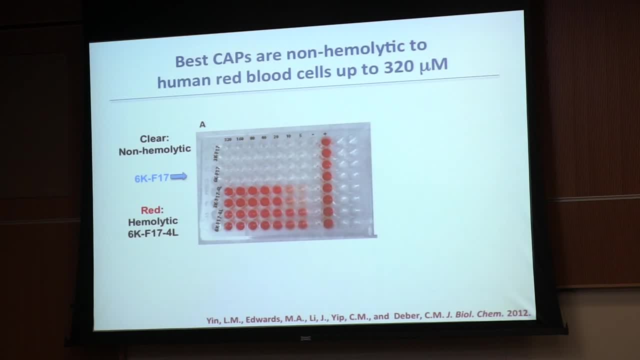 and you see the supernatant gets red. If the cells are not disrupted, then it just stays clear And you can see the stark contrast here, which fits the blue shift, which is this work that I just described, that the 6KF17 with just alanines. 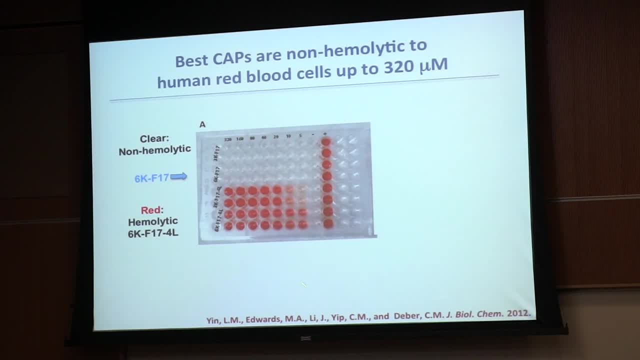 has absolutely no hemolysis. The 4-leucine one is really hemolytic. So you can immediately rule out anything with leucine like that as being a possible antibiotic, because it's dangerous to your own cells And this number, which is not sure, visible on the charts here: 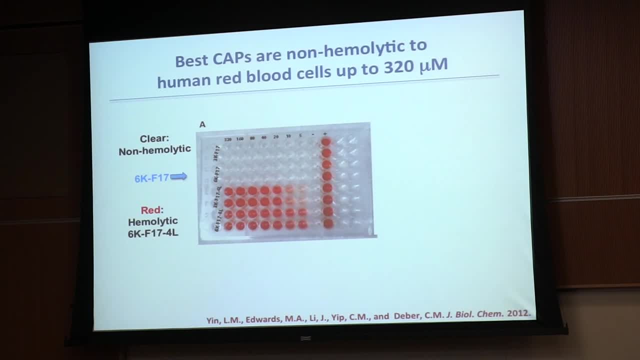 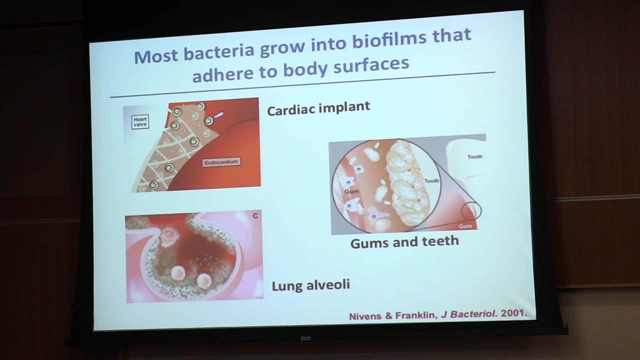 goes up to 320.. That's a huge high number for hemolysis And the gain in would be down around 10 or something much lower. So all the properties of these peptides is in the so far, so good category. But there's one twist on all this work. 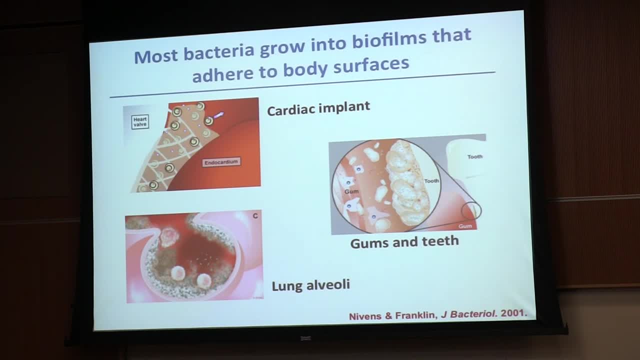 And the twist is that bacteria are not always free swimming around. Those are called planktonic bacteria. when they're free swimming, Most of them that infect us end up being colonized into what are called biofilms. I don't know if any of you have heard of this word. 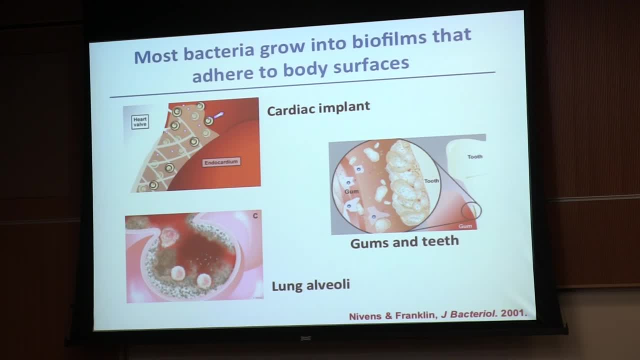 I mean five or six years ago the word biofilm was not so common. Then I heard it recently on a toothpaste commercial that you have biofilms on your teeth. So these things are basically the same bacteria, but they become colonized. 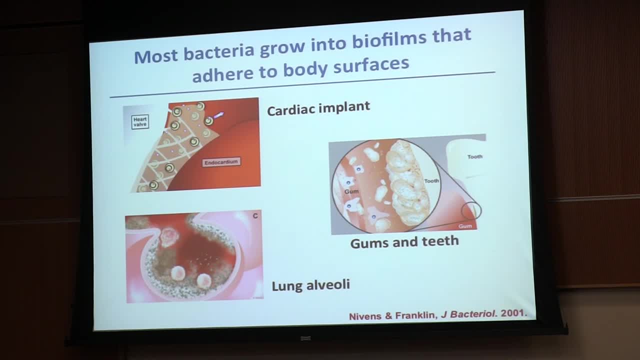 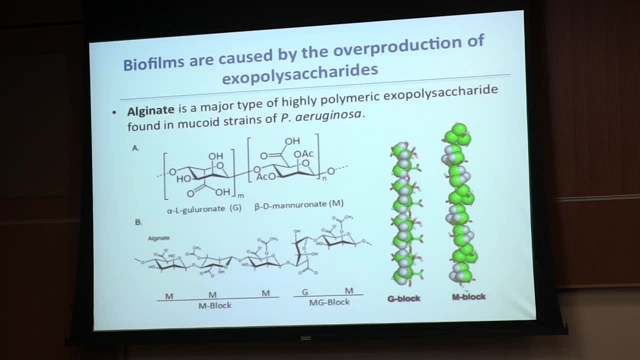 They adhere to your tissues or to your teeth, to prosthetic devices and so on, And then, once they form their colonies, they start secreting, mainly big, long chains of polysaccharides. The ones from Pseudomonas are called halogenate. 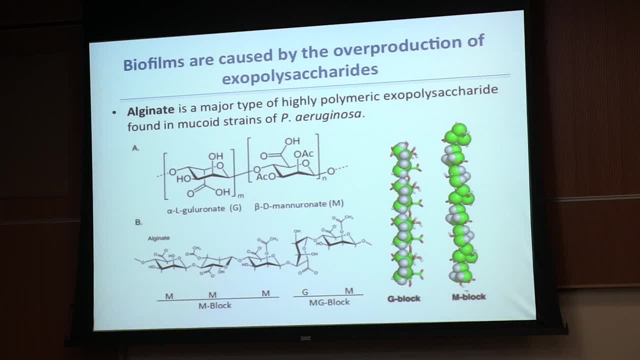 It's a major type of what are called exopolysaccharides, And they're formed in these biofilm colonies of the bacteria And they are basically sort of derivatives of mannose and this one goulose, And the difference is they just have a carboxyl group on it. 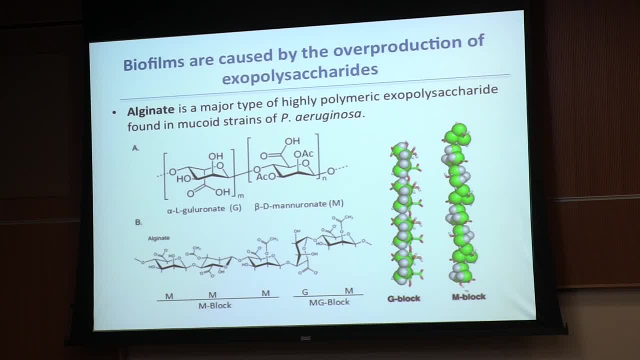 instead of another OH. But basically they're just a group of carboxyls. Basically they're just huge sugar chains. They come in mixtures of M and G blocks and depend what kind of halogenate They're actually found in seaweed. 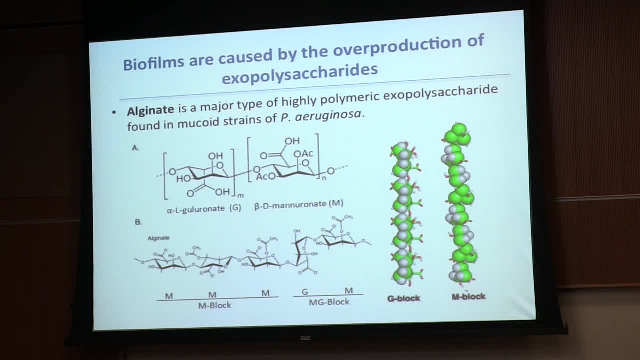 The word algae comes from seaweed. We've never been able to establish the connection between Pseudomonas auriginosa and seaweed, but it is a point to ponder. And the sugars themselves have conformations, just like proteins have helices, right. 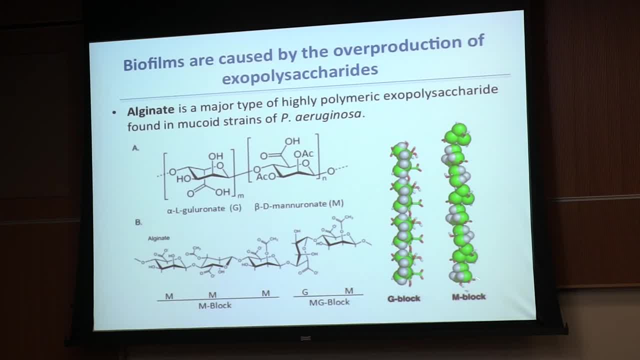 The sugars have things that look pretty organized like this little ribbons, structures, almost helical. And just a note in passing, some of them have well-displayed CH groups. The CHs on sugars can occur in different combinations, In mannose, for example. all three of them. 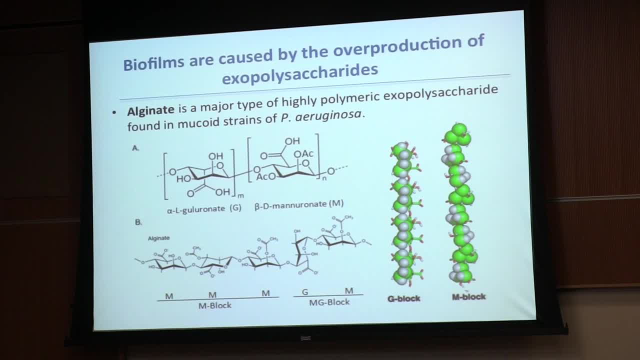 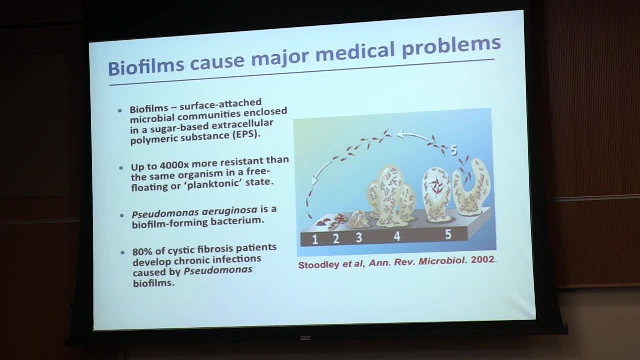 are on the same face, And that can play a role if you're trying to interact peptides with polysaccharides. So biofilms by definition, then, are surface-attached microbial colonies enclosed in this sugar-polymeric substance, And that makes them way more resistant. 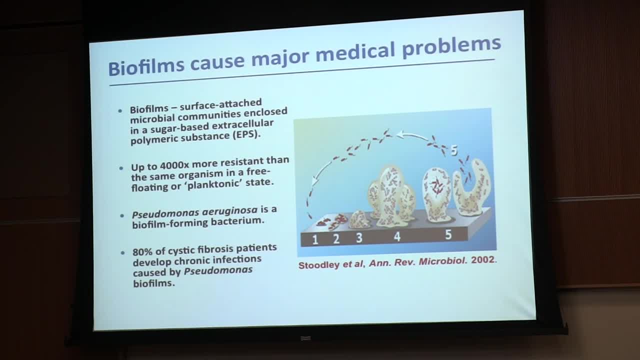 than the same organism in the free-flowing state, Because now, whatever antibiotic you give it, it has to penetrate and get to the actual bacteria. Pseudomonas is one of these biofilm-forming bacterias, And many cystic fibrosis patients develop it. 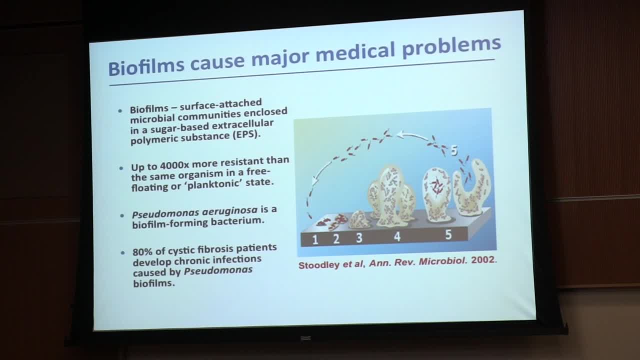 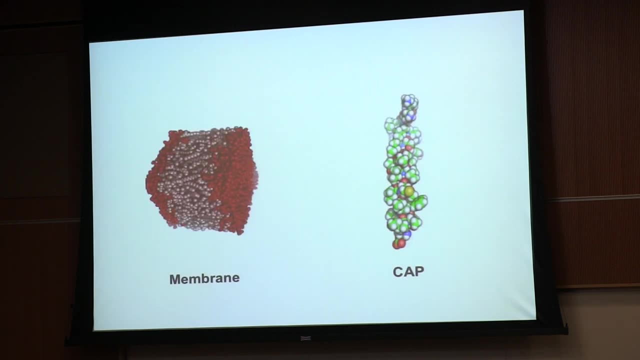 They develop these infections, And even though CF is a disease where the salt balance is not maintained, the mortality is mostly from these pseudomonas infections actually. So here's the situation, right, You've got say the bilayer of a bacteria. 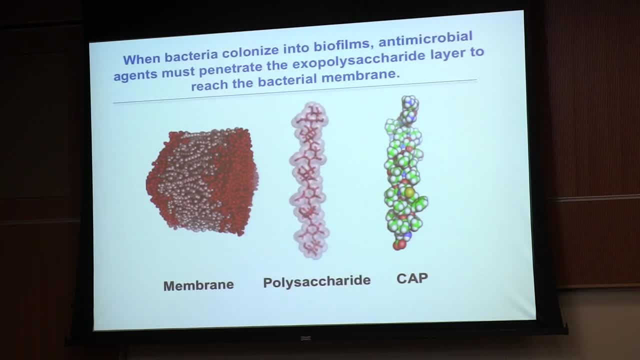 You've got a cap that's coming and it's going to interrupt the membrane, But all of a sudden there's a polysaccharide layer between them. So what is the peptide going to do when it hits the polysaccharide? 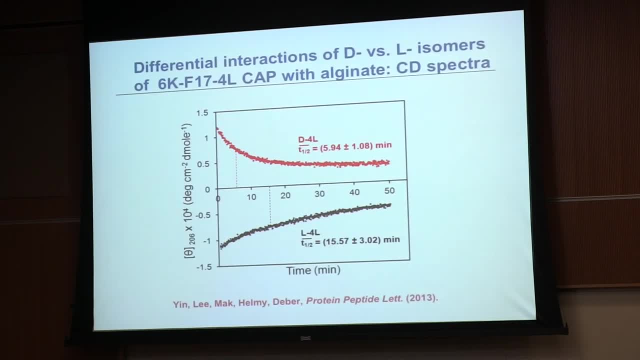 Got to get through. We found- and this is just one example of a lot of different studies- that the caps that we're working with- here's the example that happens with the 4-leu peptide that we did, but it works with all of them- that the peptides actually 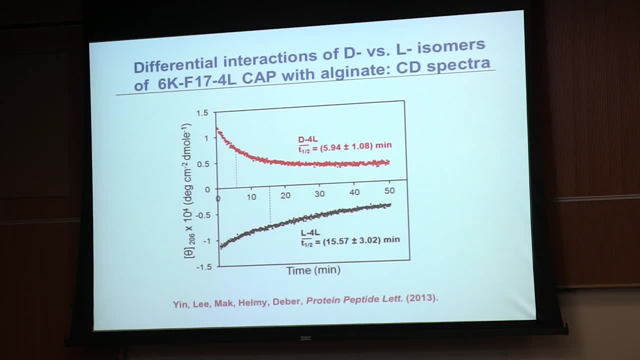 bind the polysaccharides. This is an understudied. This is an understudied area, I have to say. when we first googled polysaccharide, antimicrobial peptides- virtually nothing And the whole study of how peptides would get together. 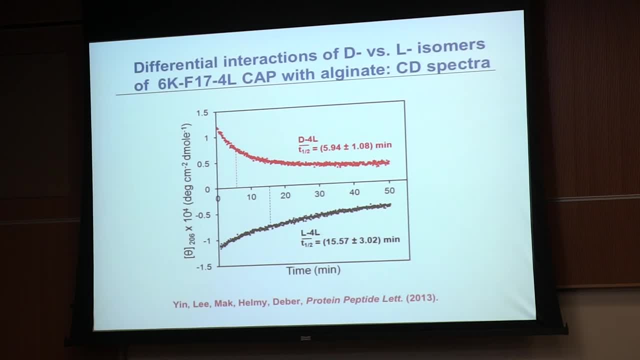 with sugars is quite an interesting thing just in itself, And considering that you have anionic polysaccharides and positive peptides, it's really the same thing. They're offering each other the same interactions that the bacterial membrane, And that's what the cap would offer to each other. 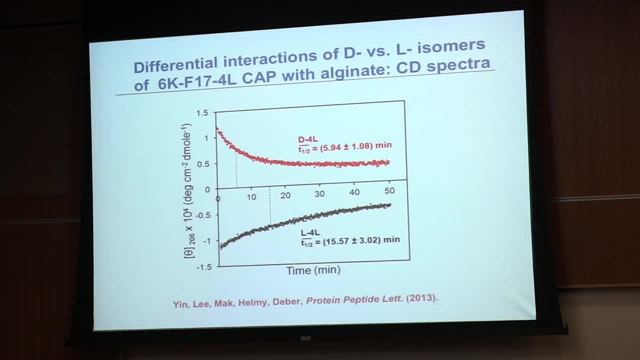 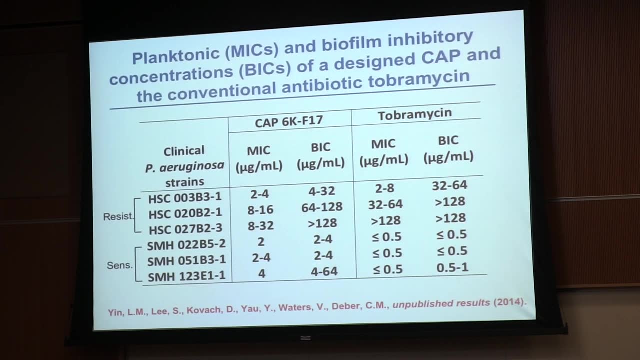 So in effect, our peptides really bind these polysaccharide layers And that can be used to advantage. So here's a chart. I don't mean you to read all the numbers here, But I want to show you what happens when you have a biofilm. 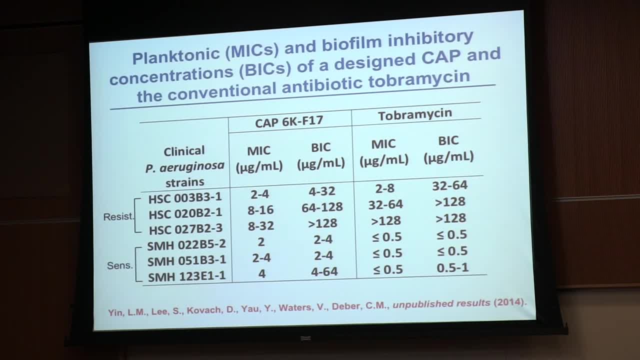 instead of a planktonic. So the MICs and the biofilm inhibitory concentrations, which we call BICs. we're comparing them with one of our other drugs, the T-Caps, and the conventional antibiotic, tobramycin, which is widely used against biofilms. 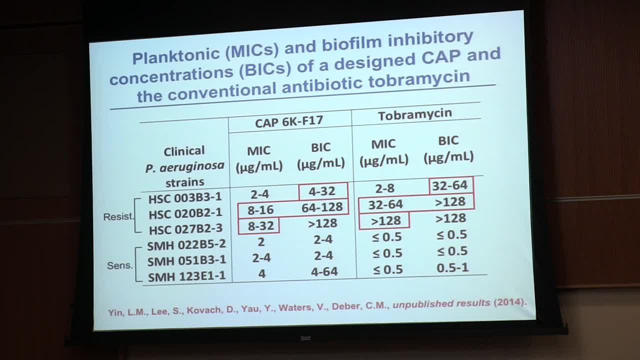 So you can see some of the numbers here. I'm highlighting just a few of them here, But for example, let's take this resistant strain- The MIC is 8 to 16 for the MIC And then it goes up to 64 to 128 for the biofilm. 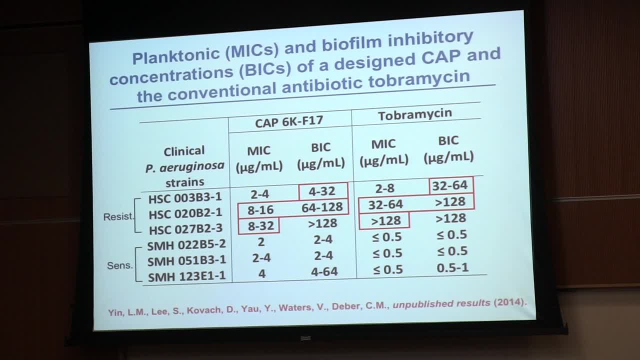 So you see, the biofilm is much more resistant. That's what that tells you. Now, This is a drug that's actually used in the clinic for these things. You can see, the MIC is around 32 and greater than 128 for the biofilm. 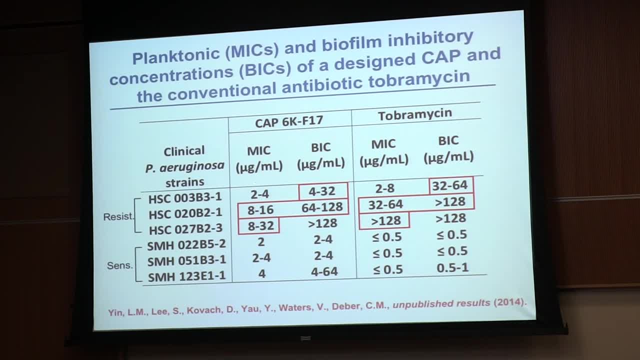 So what this means is that our cap has lowered both the MIC and the BIC, even lower than the one that's being used in the clinic, So this is a very good result. Here's another one. This one, in the MIC, is way lower. 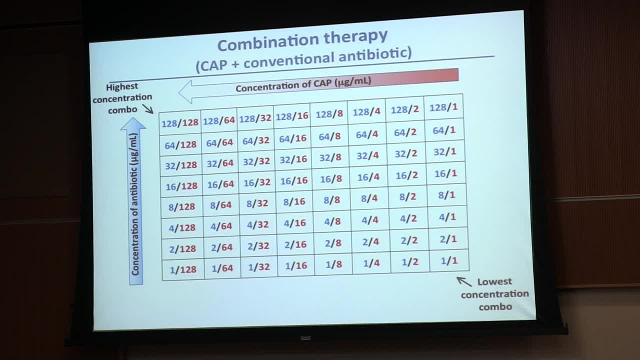 So, with this in mind, we undertook some combination therapy experiments And basically this is a grid where you add your peptide, let's say, in one dimension And you add your conventional antibiotic like tobramycin in the other direction. 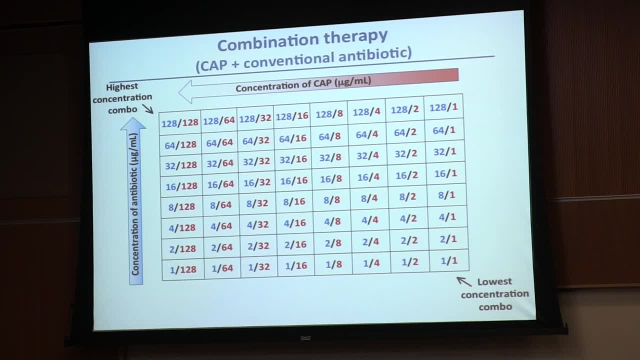 You mix them together, So each well has different concentrations and ratios of these things, going from the lowest combination. So it will be one micromolar, say, of each, or one microgram each here and up to 128 micrograms. 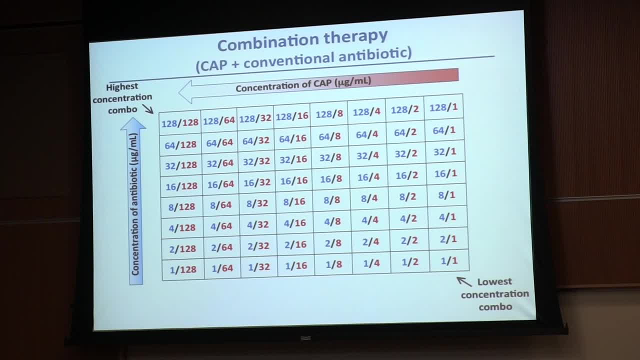 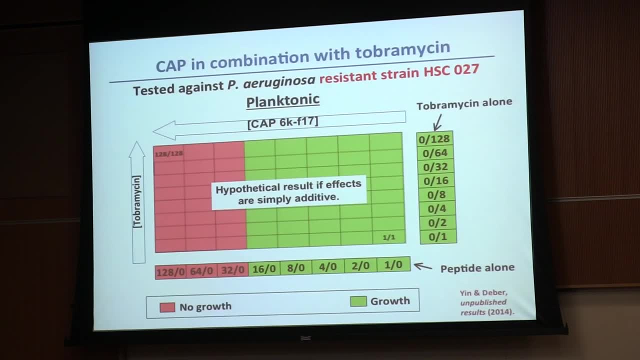 Each up here And you look to see how they work alone and then how they would work in combination. So here's an example of how we graph these things. Tobramycin alone, if you used it against this particular resistant strain of pseudomonas in the planktonic form. 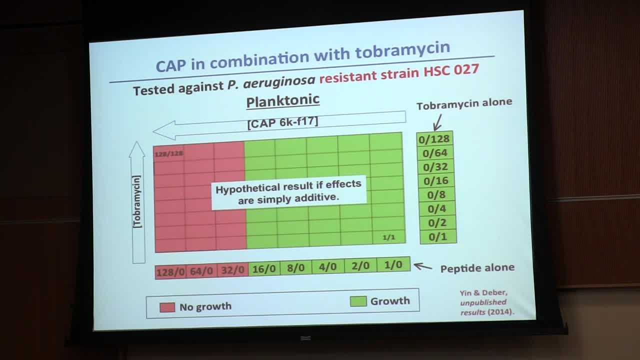 no matter how much you add, from 0 up to 128, it's green, which means that there's a little bit more, that tobramycin cannot fight this strain in that range because they grow no matter how much you put. If you try the peptide alone going along this axis, when you get up to 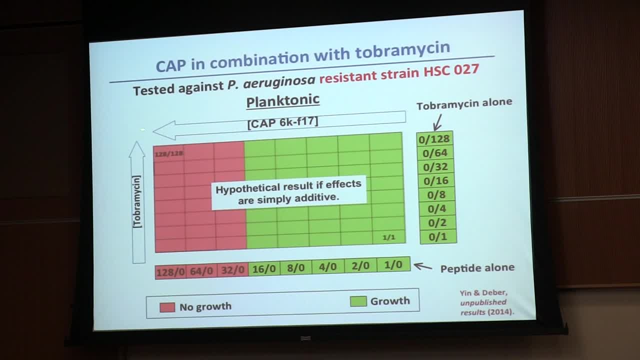 about 32 micrograms, it starts to kill the bacteria. So anything above here is all no growth. So this is what it would look like. if you had done these independently and just graphed them. you would see something like this: So now what would happen if we mixed? 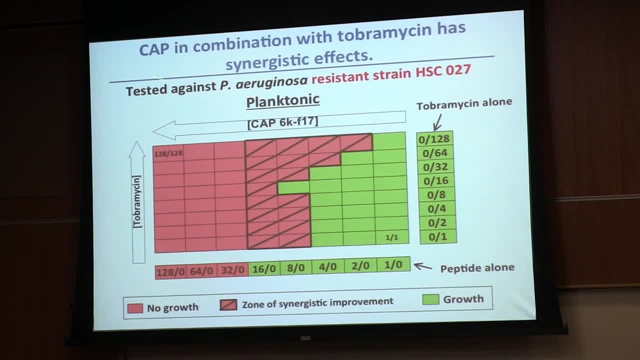 them together. So here we're testing against the planktonic resistant strain. Here's tobramycin alone. It's still green. here The peptide alone is still red, above a 32. But now the growth has been stopped in all of these wells. So in other words, the combination of these. 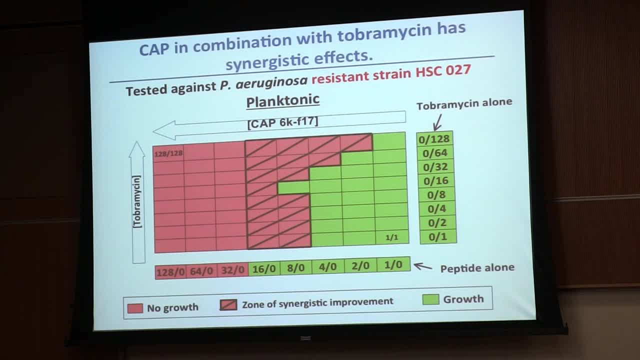 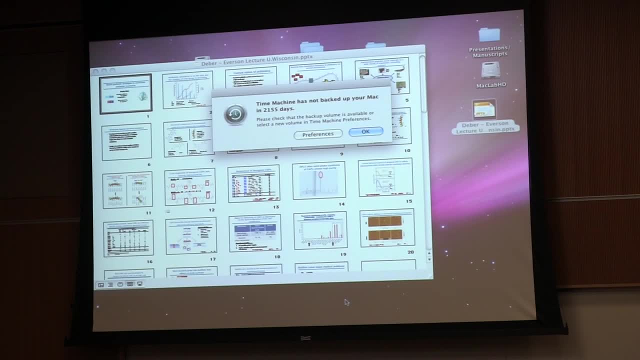 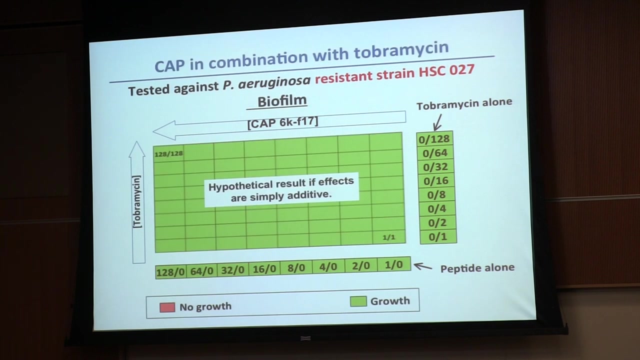 two is highly synergistic, And now between the two of them together they're able to kill the bacteria at a much lower rate. So this is a very encouraging thing here. I really must back this up one of these days Or years. Here's another interesting example of this. Here's a resistant strain and now 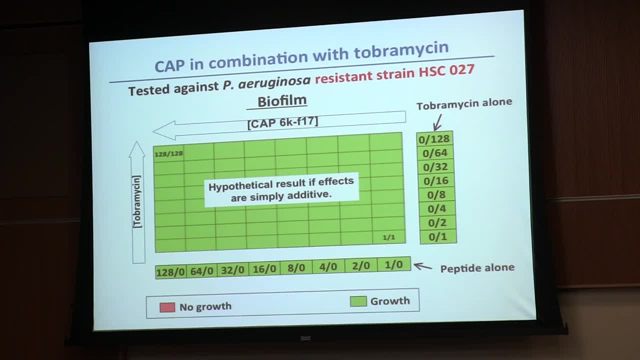 we've got the biofilm, So this is the big enchilada here, right, Biofilm. Okay, so this is a very interesting experiment. And this strain, tobramycin, alone- no effect. R-peptide, one of these 6KF17s, alone- no effect. So if we use either one of these individually, 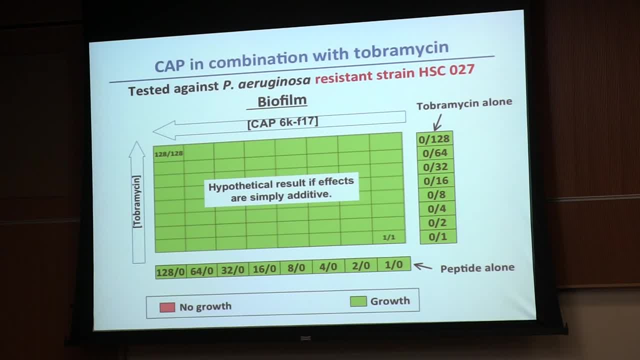 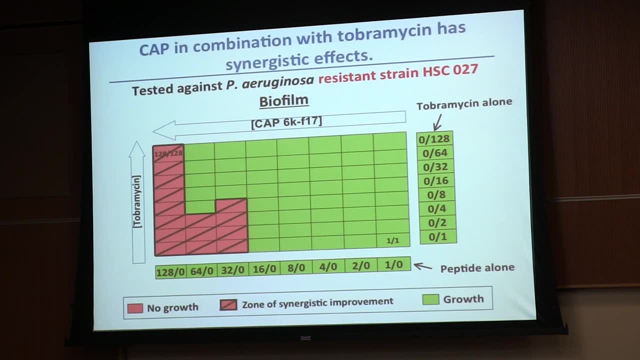 neither one of them can touch the biofilm form of this resistant strain, And this is the toughest ones in the lungs of the CF patients. I should say that these combination therapy experiments have been tested on clinical itinerants. Now, this is a very interesting experiment. 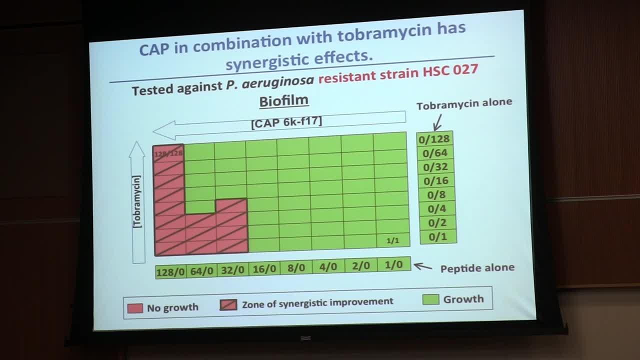 This is a very interesting experiment. Here's another interesting experiment. Here's a combination of these two. Here's a combination of these two. Here's a combination of these two. Here's. So this is from the sputum of CF kids at the hospital. 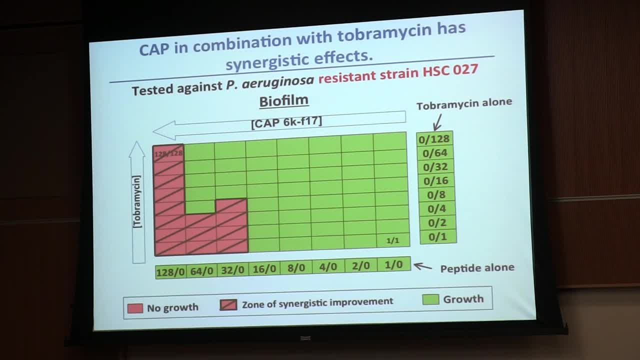 for sick children, So they each have a different strain of Pseudomonas, So we're testing them in a live way. This is one of the good things about working at the hospital is that the clinicians and the scientists kind of work together. 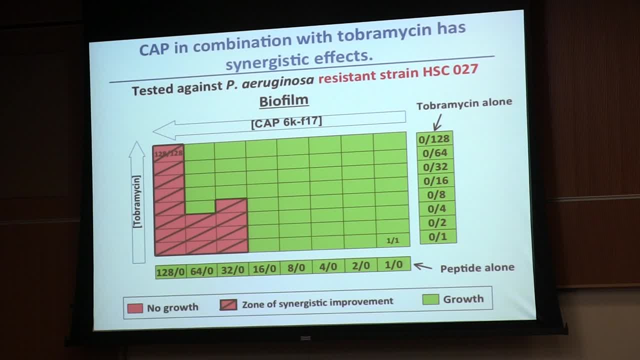 This is a really good example of what could be accomplished here, And this is a very good result, because now we have a considerable region of red, which means that in combination now these two drugs have the potential to kill the Pseudomonas in the biofilm form. 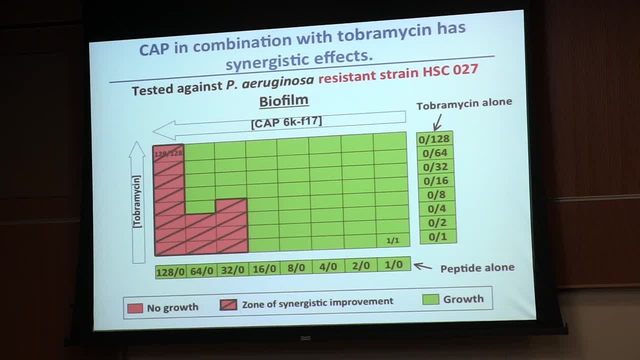 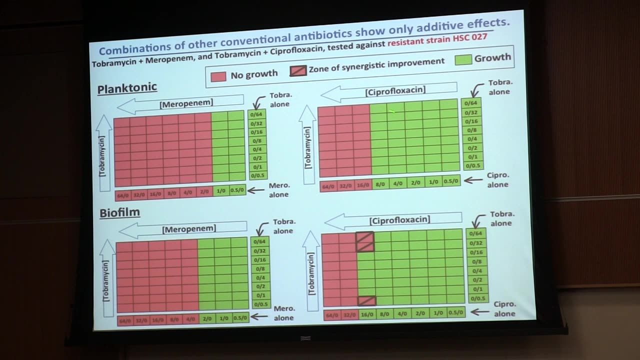 at relatively low concentrations. 32 micrograms is still pretty low as these things go for doses. So very pleased about all of this And we did, just for sort of controls, we did the three antibiotics that are used most often in CF therapy. 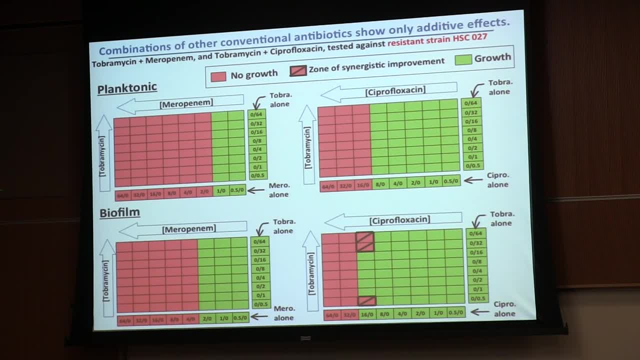 Tobramycin, And I call that Cipro or Meropenem, And basically just to summarize all of this, mostly they're just additive and there's very, very little synergy. So even when doctors use sort of a cocktail, as they call it, 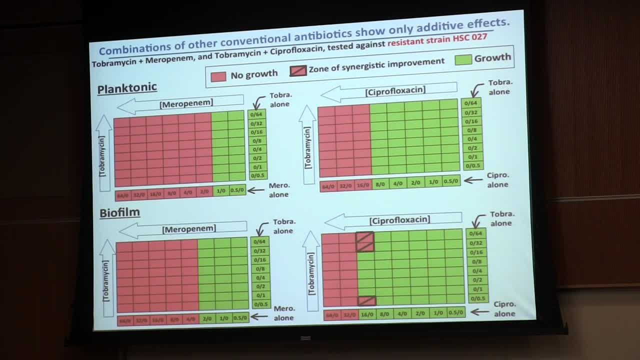 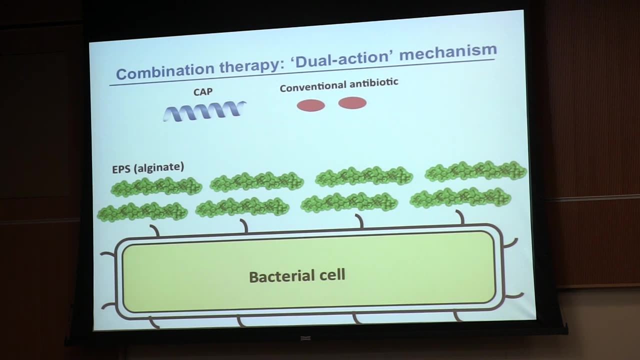 of different combinations of these. the combination really doesn't enhance the situation. Of course, these are all in vitro studies And you know everybody, every patient is different, But it's all very promising. So to sum up basically what I've been telling you about all these CAPs and the combination: 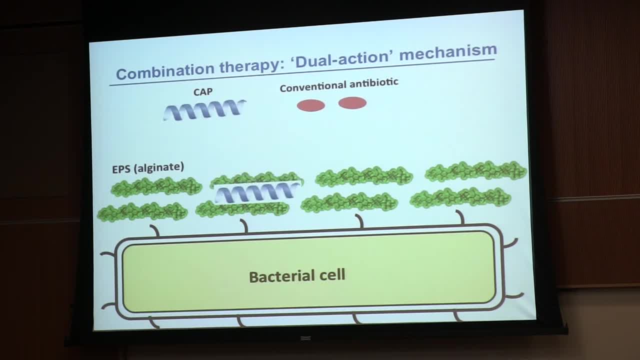 therapy. we think there's a dual action mechanism. We think the first thing that happens is that the peptides can bind the alginate or the polysaccharide layer. If you get enough peptides, it can basically disrupt the alginate and some of the peptides. 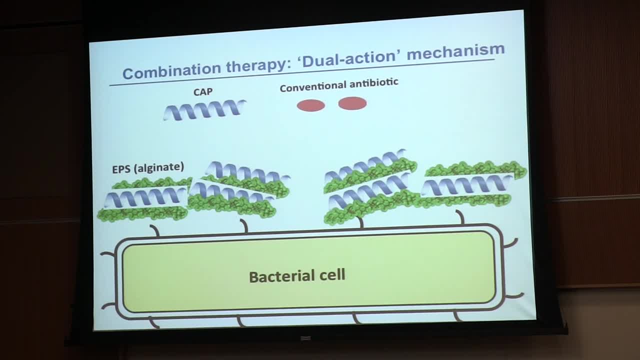 actually precipitate the alginate. You can see this in the test tube. So once the alginate layer is disrupted, one of the conventional antibiotics- so this is the combination therapy idea- can get past the alginate and get into the cell. 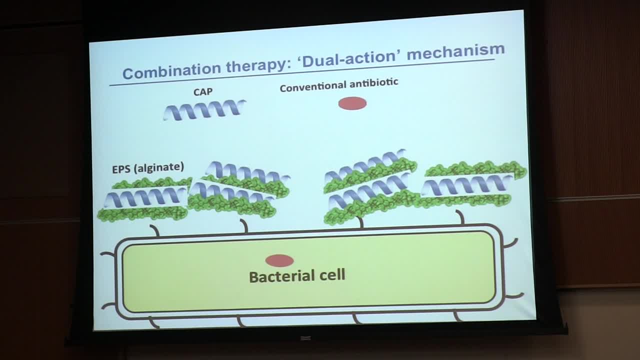 So it's almost like changing the bacteria back to a platonic planktonic. But that's not the whole story, because now, remember, the CAPs can coat the bacterial membrane surface like a carpet mechanism And weaken the membrane And weaken the membrane that way. 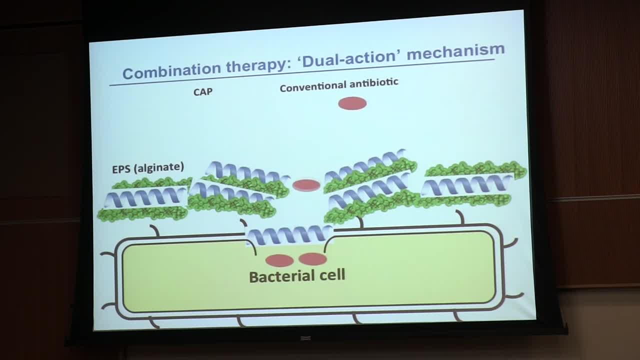 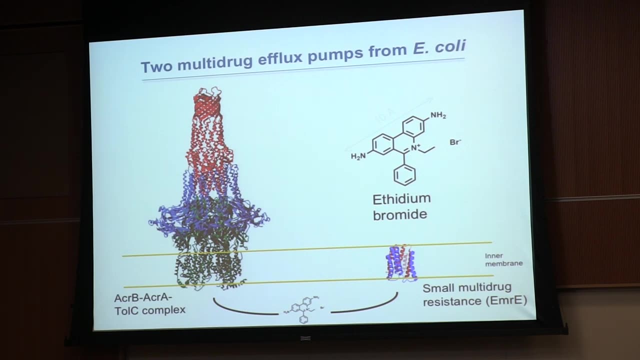 So now the conventional antibiotic has an easier path into the bacteria. I can watch this all day actually, OK. So right now a lot of interest around our place is in the CAPs and, we hope, in the longer range. People always ask about commercialization of academic discoveries and we hope this. 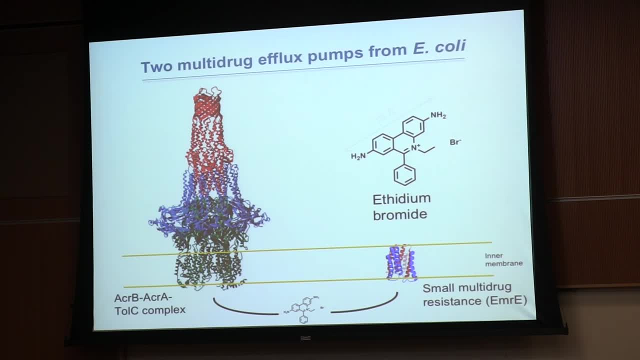 may be an example of it. So for the last few minutes here, I'm going to give you a survey of something that's happening relatively recently in the lab, And that is the idea of trying to stop bacteria from pumping out the drugs that we add to. 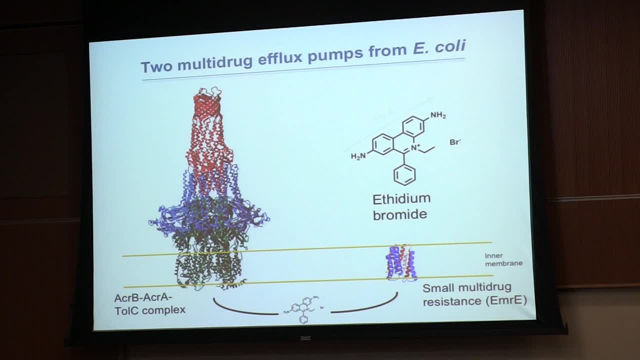 them Now. as I mentioned right at the beginning, the bacteria have small multidrug-resistant bacteria And the bacteria, as you can see on the slide, they're very resistant to these small multidrug-resistant proteins as depicted by that blue cylinder, if you remember. 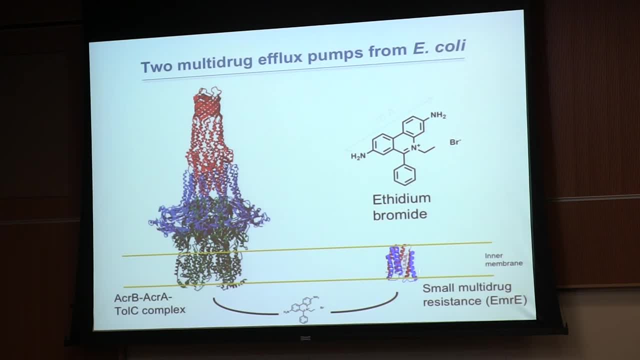 And that's what this thing is. They're called SMRs. A lot of bacteria have them. This one is called EMRE. This is one that happens to be from E coli. Now, bacteria have like five different categories of these pumps that pump drugs out. 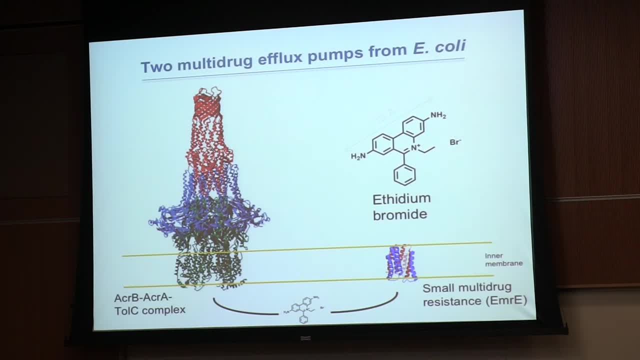 The two of major interest to us will be these small SMRs. It's called ACRB, ACRA, TALC complex. This part of it in here in the membrane is very similar to this part of this protein, And then it goes into a long and cooperative pathway, ending up in a sort of a beta-barrel. 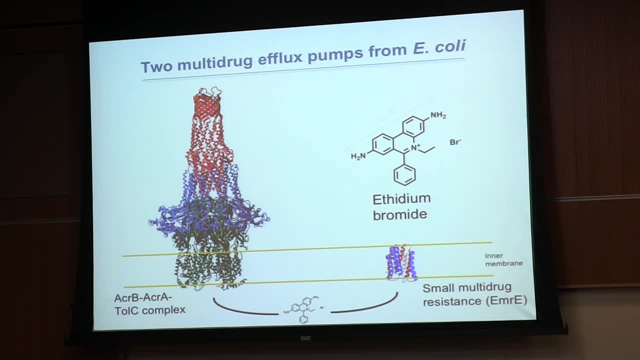 structure that enables the bacteria to pump the drug out and past the periplasm, and out past the cell wall, if there is one, and finally all out. So actually some people believe that the small ones pump it to here and it gets about. 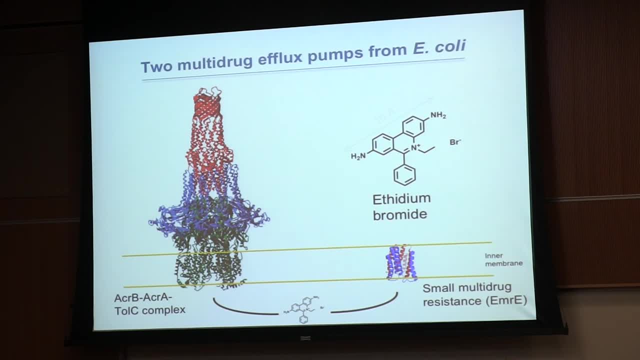 this far, And then it continues the rest of the way. So between these two they are the major sort of drug pumping complex. And now you may well ask here, doesn't this look a little bit small to be pumping out some big drugs? 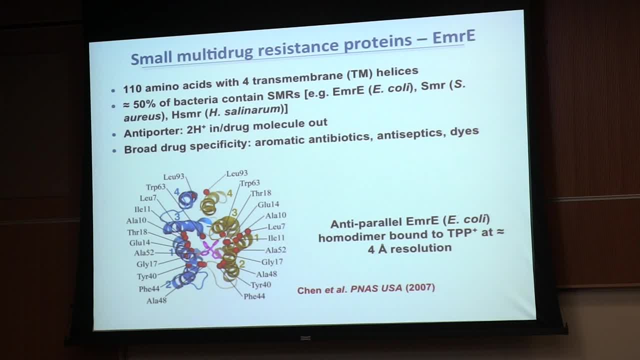 So let's look a little more closely at these SMRs. They're usually just over 100 amino acids. They have four transmembrane helices. About half of the common bacteria have these things, Including E coli and Staph aureus and HSMR, which is called H selenarum. 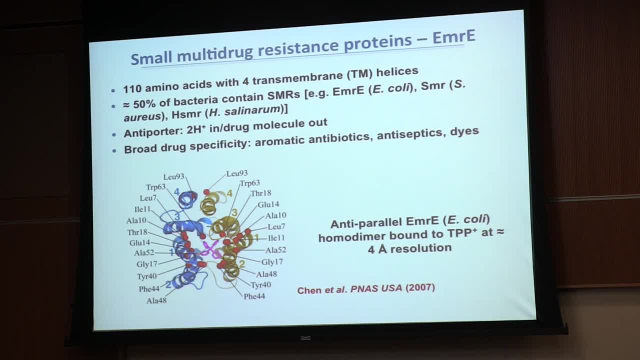 It's one of these archaebacteria that's used in lab studies, And I could add to that list Pseudomonas aeruginosa. PA also has these. There's a mechanism where protons go in and drug molecules get driven out. 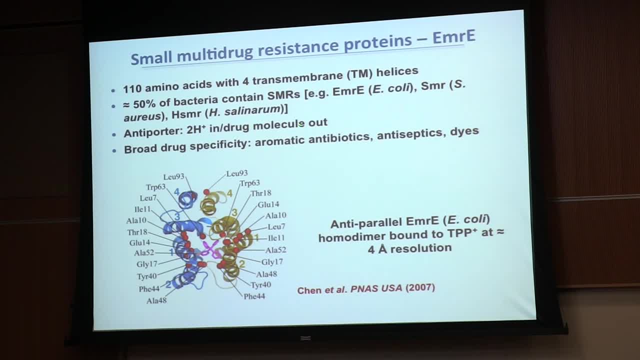 And interestingly, with these things there's a broad specificity, because you've got aromatic antibiotics, antiseptics like disinfectants, Dyes and so on- all be pumped out. So how does a small molecule pump out all of these things? 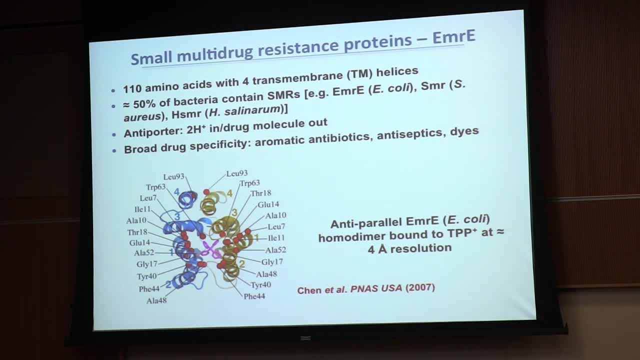 So the X-ray structure and just other evidence suggests that the minimum structure of these SMRs has to be a dimer. You can't have one thing with four helices pumping out big. you need some kind of channel or something. And it's believed to be formed by two molecules coming together with six transmembrane helices. 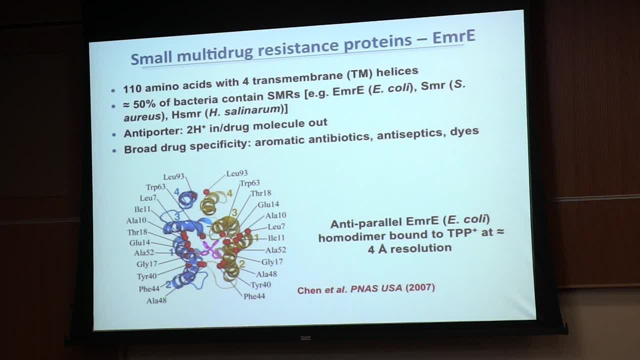 And this can figure out what's going on. There's calm, there's tension, there's saturation, and then the substrate goes through the middle. This one shown here is a tetraphenyl phosphonium. It's not a high resolution structure, but it does give the idea that this is the main. 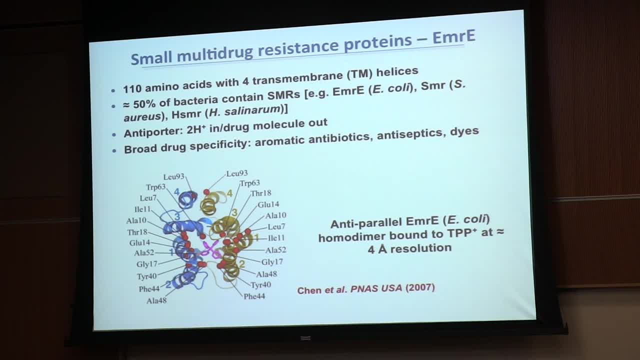 business part of the molecule, But it still has to be held together as a dimer. So the dimer is held together up here. The TM4, the fourth transmembrane segment, is like away from the other three here and then two here. 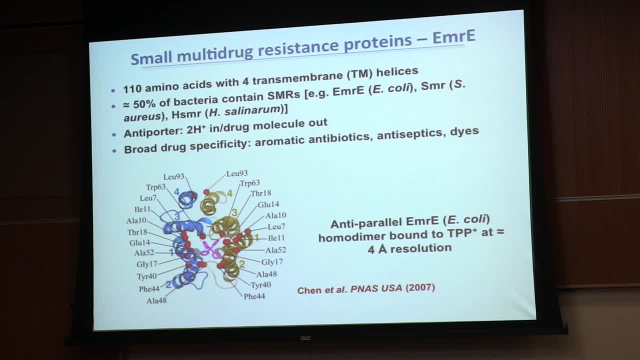 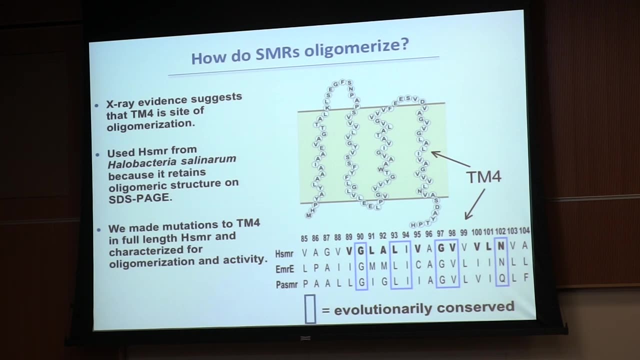 And these two bind each other through a cross-section of residues. It's a TM4-TM4 interaction that is basically holding the dimer together. So you can look at the sequence TM4 and see what's going on with there. The x-ray evidence suggests that this. 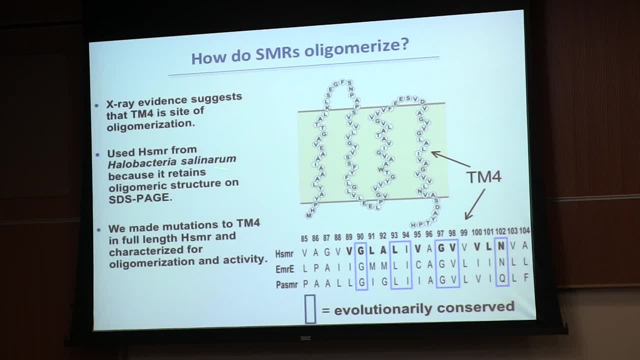 is the cytoligomerization. We used an H salinarum, HSMR because it shows the dimers on SDS page, And we made a bunch of mutations to the TM4 in one of these SMRs just to show that the TM4-TM4 interaction is the main thing. 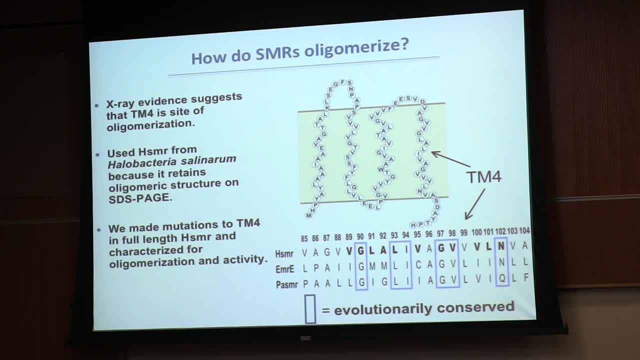 and also to determine what residues are actually involved in that. If you look at some of the actual sequences, you see some sites are conserved all throughout different bacteria evolutionarily conserved. So this gives us an idea that somewhere right in here between about. 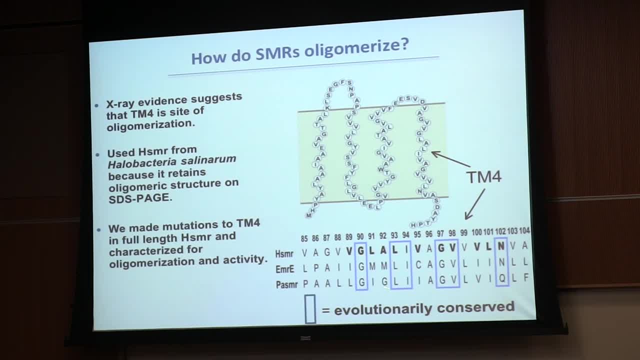 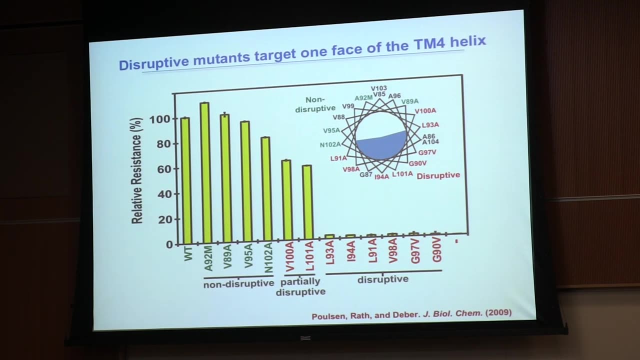 88 and 99, somewhere in there. this is most likely to be where the TM4-TM4 interaction is. It's a little bit like a scissor or cross-section through the middle of the TM. So we made mutants of all residues in TM4, focusing on the 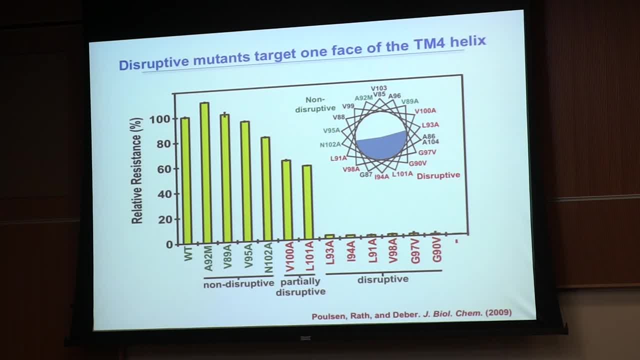 These are just some of the main results here And basically what we did. we made some small to large, Some large to small, like L to A or V to A. If we had G, we made it G to V, and so on. 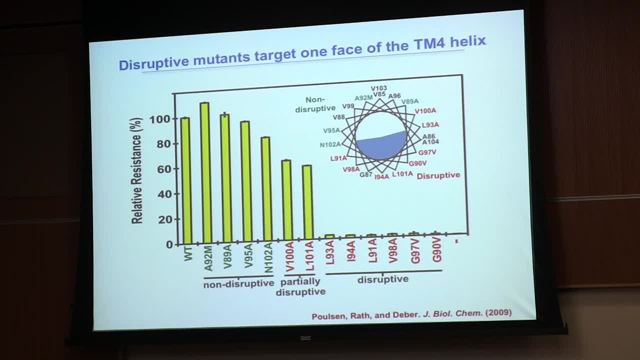 just with the idea of disrupting any motifs that might be dependent on the size or shape of the side chains. And we got this pretty remarkable result here that if you graph these residues on a helical wheel, so you're looking at it from the top. 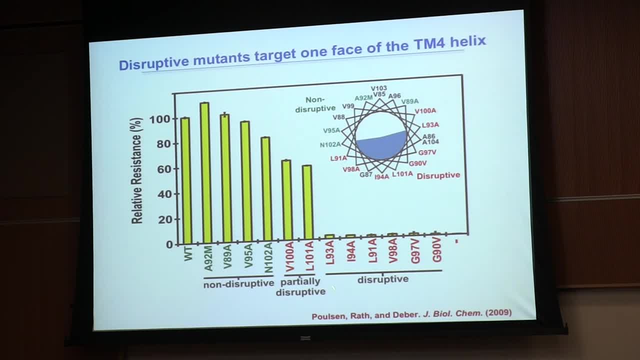 and you see all the residues. half of the residues had absolutely no effect really on the ability of, in fact, the proteins to pump out a toxin. The one we use is called ethidium bromide. It's a laboratory model. 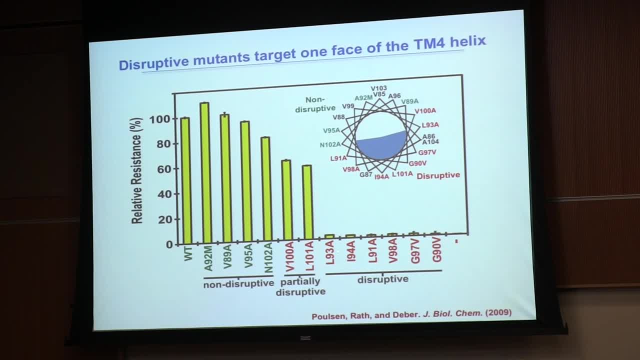 On the other hand, if we use these ones given in red, which map to this face here, you can see the distinction: All the disruptive mutants are on one face and all the green or non-disruptive mutants are on the other face. 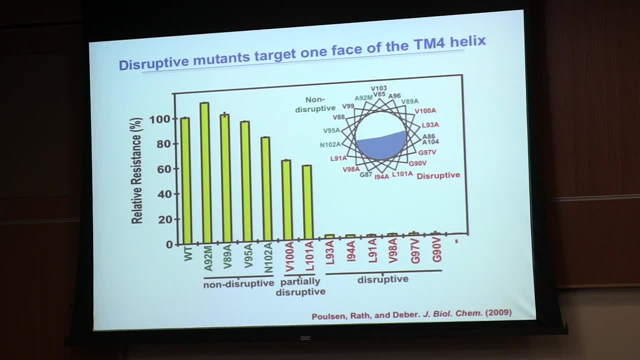 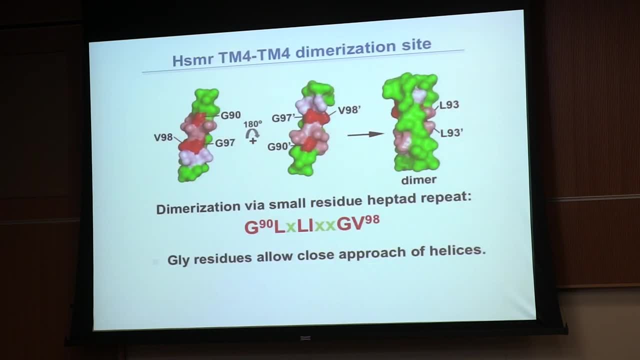 It's pretty well telling, Yeah you that this is the face that's going to be involved in the TM4-TM4 interaction And, in greater detail, this is what it looks like. here You have G90 to V98.. You have this. 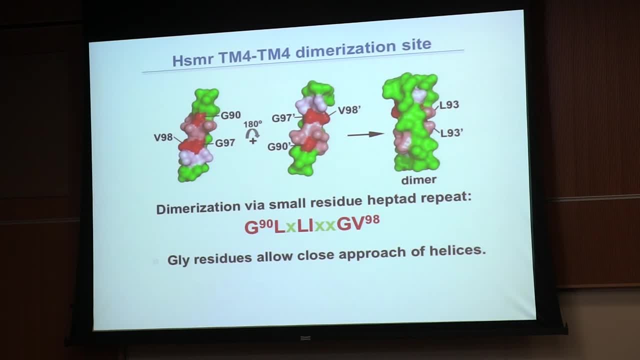 GG7 motif, which is similar to the GG4, two turns of the helix. that allows the helices to have close approach. You have a couple of hydrophobic residues of leucine and isoleucine and valine and then a couple of other of these X residues. that can be one of many different. 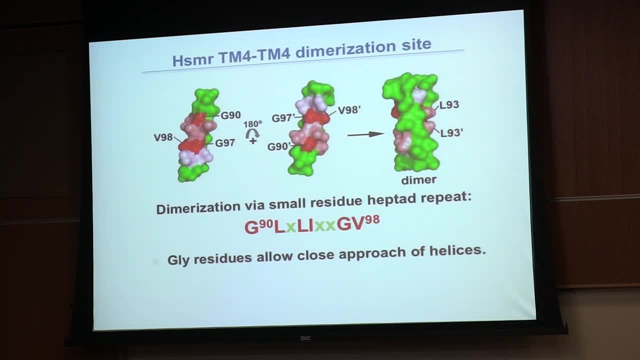 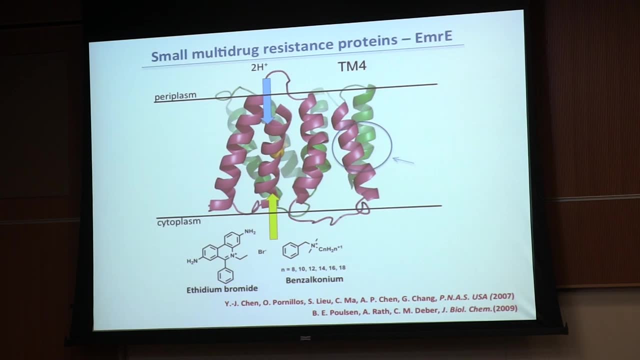 things. So this is basically the dimerization site and this is what's holding the SMR into a dimer. So, to summarize what I've said so far, here you have a dimer. You have these three helices: TMs 1, 2, and 3.. There is a glutamic acid that's conserved in there, GLU14. 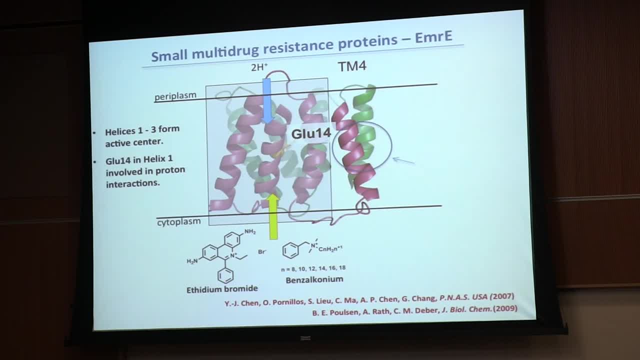 It has to do with a transient interaction site as the substrate passes through. And then you have the motif G90 to 98, and this is the minimal dimerization motif. So it's like two, almost like two separate parts of the dimer. 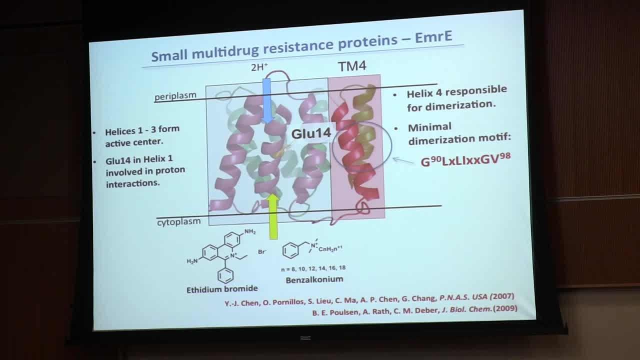 So this protein can pump out ethidium bromide, which is a toxic dye that has certain fluorescent properties that will be useful, And it can also pump out something that's called benzalkonadine- if you recognize that That's a disinfectant that's used in hospital surfaces when you 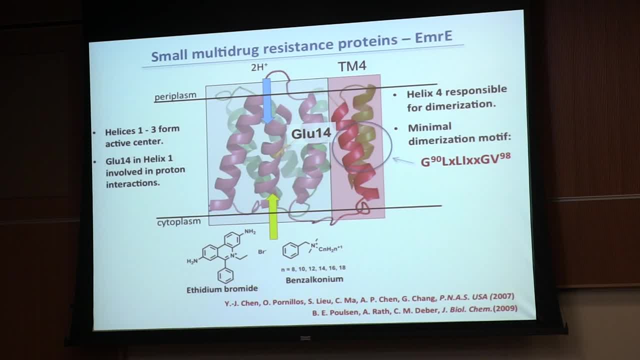 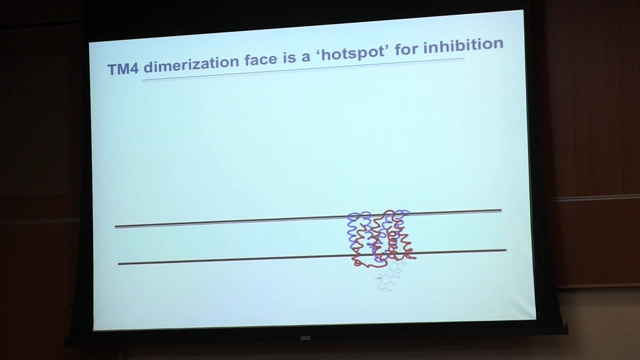 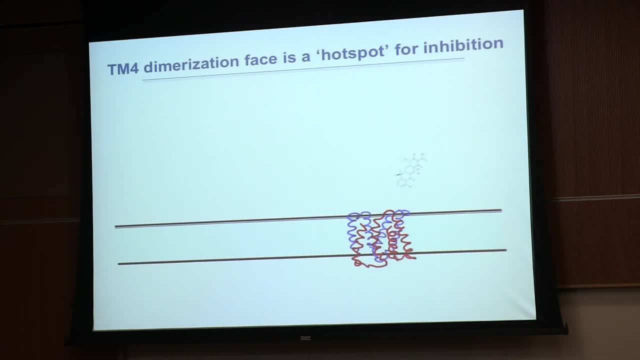 And it. now there's the record of this amine, Patyrac, Clar, silentlybird, Stimuli, Redmare, MS. And here's also the Petrocycline and the one of the substrates for the SMRs. So what are we going to do about that If we want to stop it and we have some understanding? 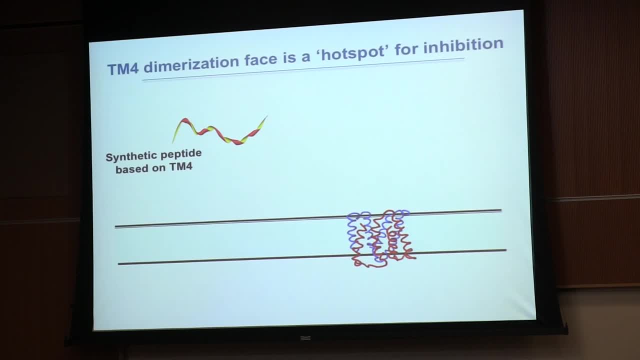 of these membrane active peptides we'll make a synthetic peptide based on TAM4. That seems a logical place to start And we hope it'll have some sort of transmembrane insertion And then we'll hope it will head to the TAM4, TAM4 interaction, bind the TAM4, compete the. 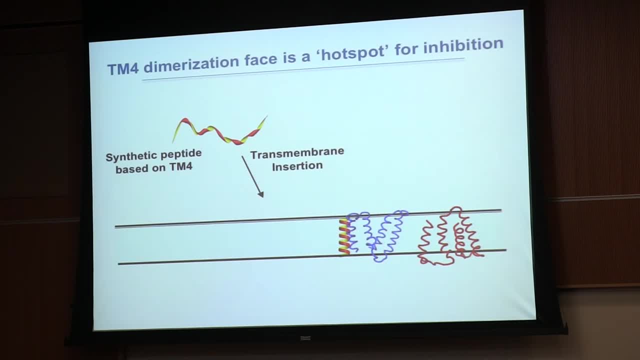 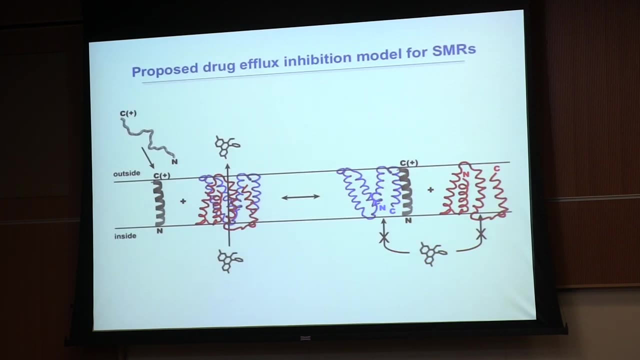 normal TAM4, TAM4udible dimer out and create in effect two monomers, And these monomers will not be able to pump the drug, At least that's the concept. So we hope to inhibit tetracycline transport. 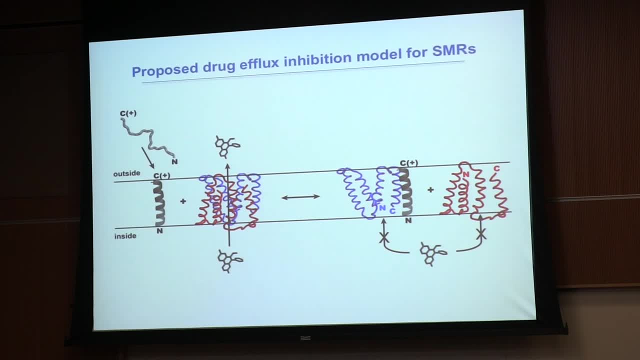 So, in order to do that, we had several iterations before we hit on one that really worked. Some prerequisites: First of all, you have to have positive residues, As I mentioned, or else the peptides are going to be insoluble. But in this case you have to have one end that's neutral. 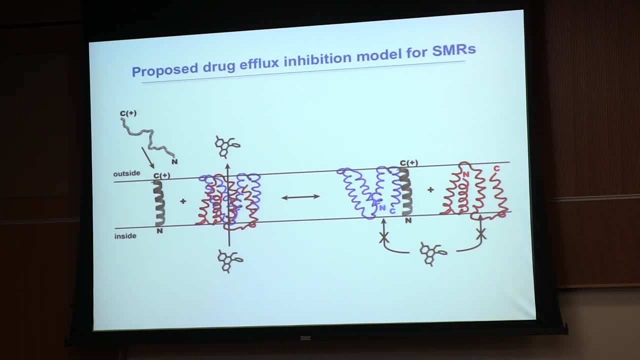 Because if you want the peptide to sort of tunnel in to a membrane like a corkscrew kind of thing, you can't have lysines on that end because it's not going to enter the membrane. So what we have anyway is, if we 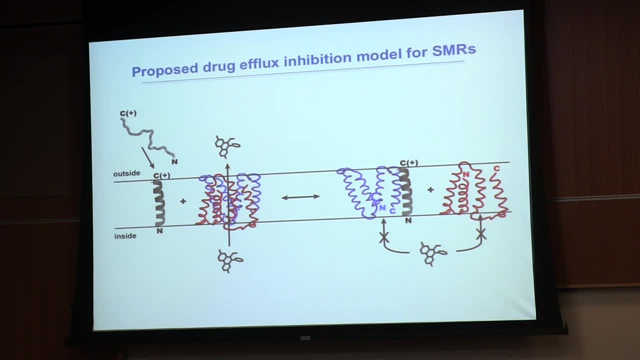 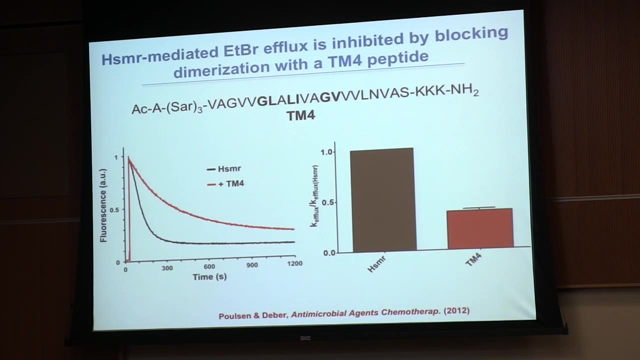 could design such a peptide, we hope that we would be able to inhibit the export of the ethidium. And basically, in this case, our idea is to just break down. Break the two up into two monomers. Well, it works. 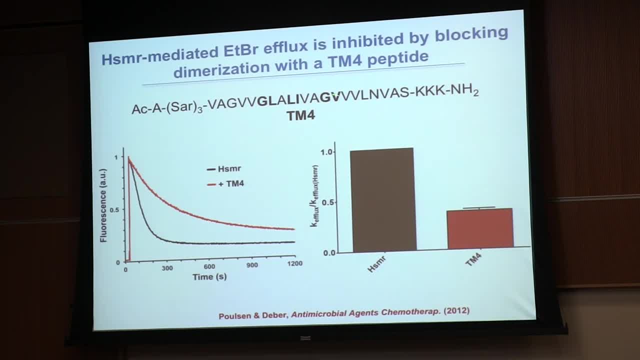 So if you make a peptide that is just TM4, that's the exact sequence of the wild type TM4, you put three lysines in over here just for solubility. And on this side we used after a lot of trials and errors- 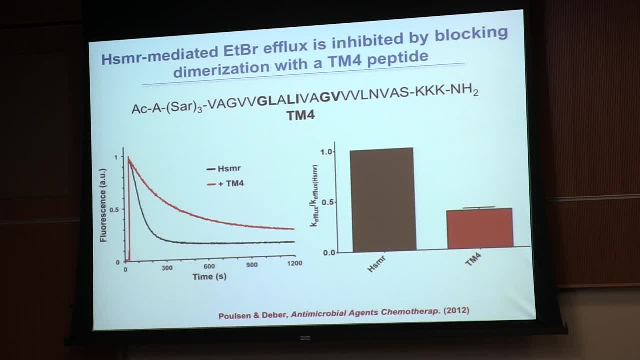 sarcosine. if you know what it is, It's an N-methylglycine. It's something that's called a peptoid. So proline would be an example of the natural thing where the N is substituted by another carbon bond. 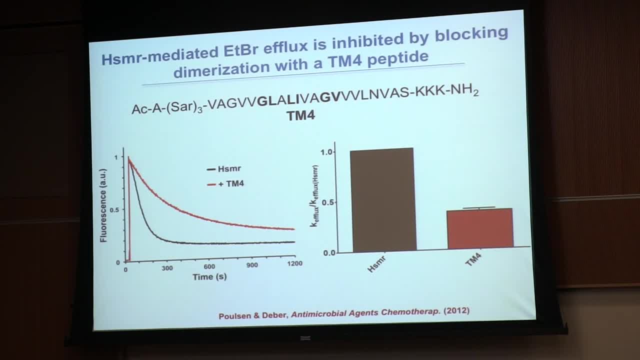 In this case it's just N-methyl, So it's actually a very simple glycine derivative, But because you put the methyl on, it gets much more water soluble. That's what happens actually. You get a secondary amine function. 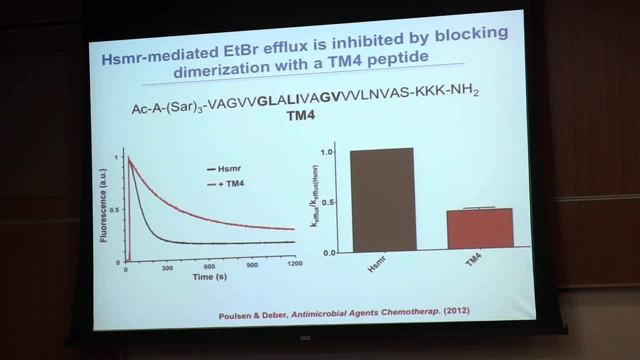 And right on the end of it is acetylalanine. So what happens here? if you take some E coli cells, you suspend them And you add ethidium bromide, which is a toxin, The cells just pump it out. 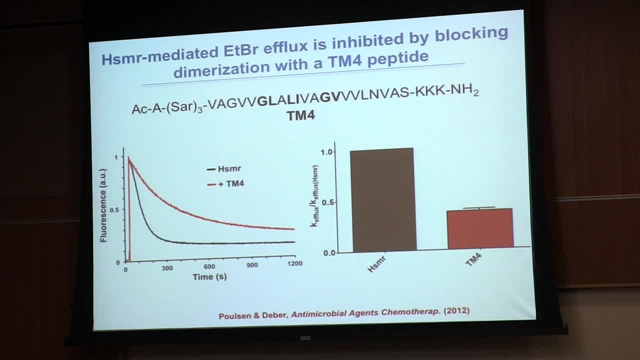 So the ethidium is a DNA-binding dye that is pumped out And it changes its fluorescence depending whether it's bound to DNA or just out. So this is the thing you normally see: The fluorescence signal drops. So what happens if we do the same experiment? 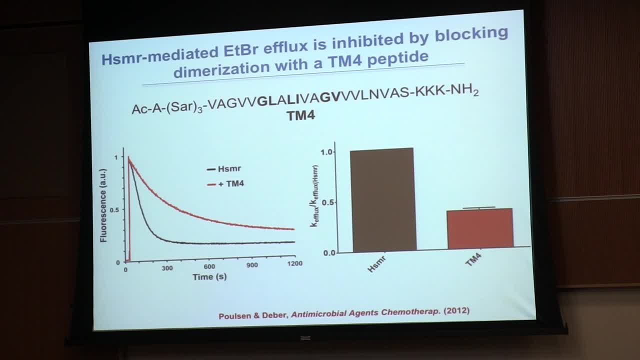 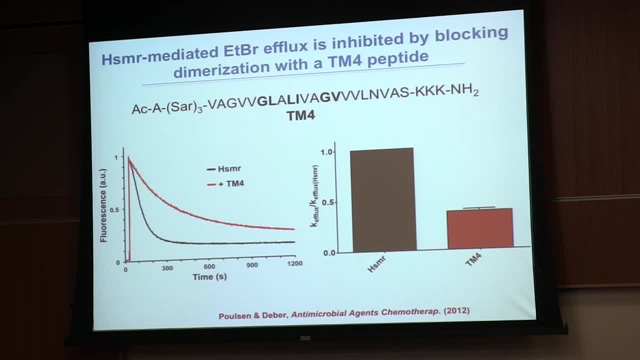 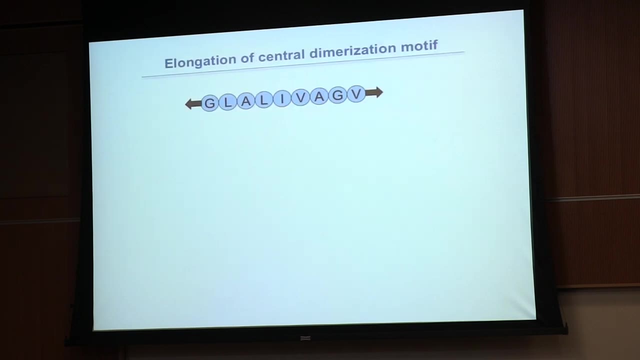 In other words the TM4 to a great extent- actually about 60%- is inhibiting the bacteria from pumping out the ethidium. Now there's always some background stuff because there's other transport mechanisms so on, But this we thought was a very good start. 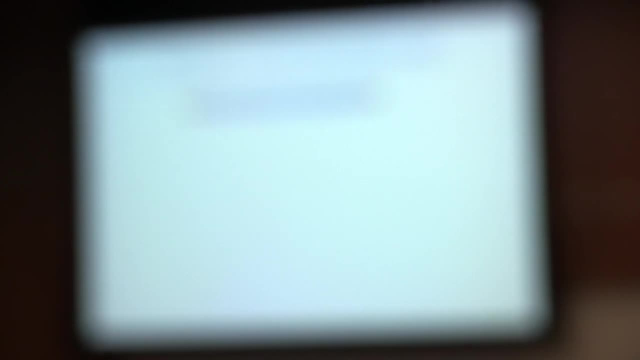 So now, if you want to make this a useful inhibitor that might actually be used in real life, something, Of course it's way too long, So the natural thing is to see how short Can we make it so that it would still work. 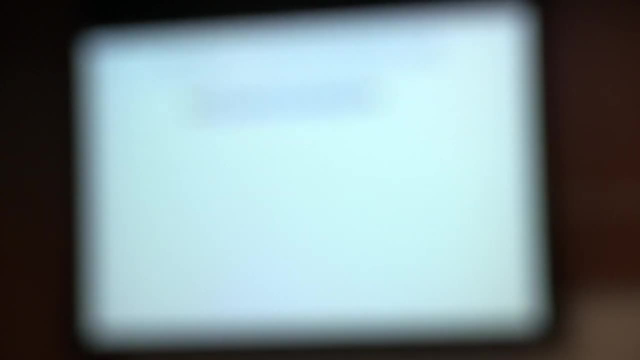 And what you're thinking of now is that heptad in the center part of the TM-TM4 interaction. So that's exactly what this sequence is here, And we can make shorter peptides with just TM4 90 to 98, keeping the sarcosine and lysine. 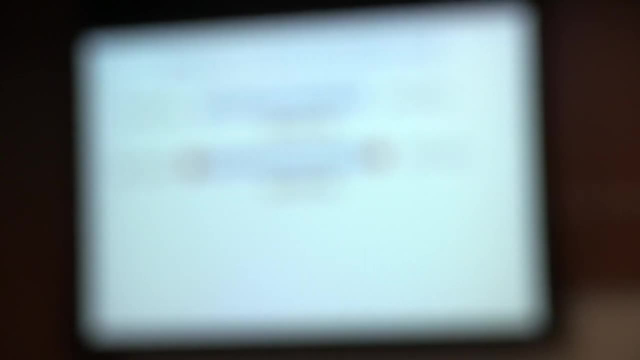 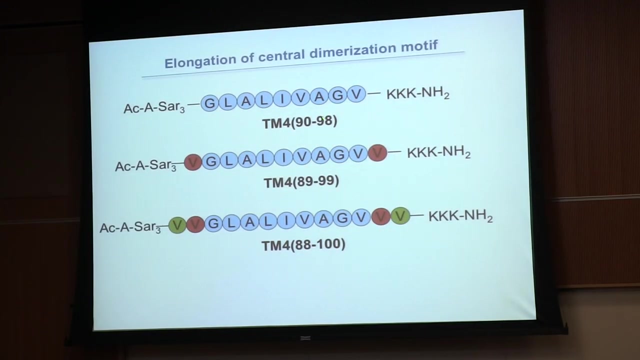 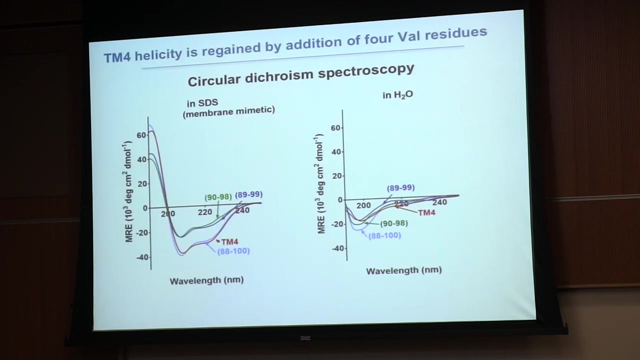 We can make it two longer. We can make it two longer, So keep in mind the numbers here. The shortest one is 90 to 98.. The longer one is 88 to 100.. So first of all, we showed an interesting thing. 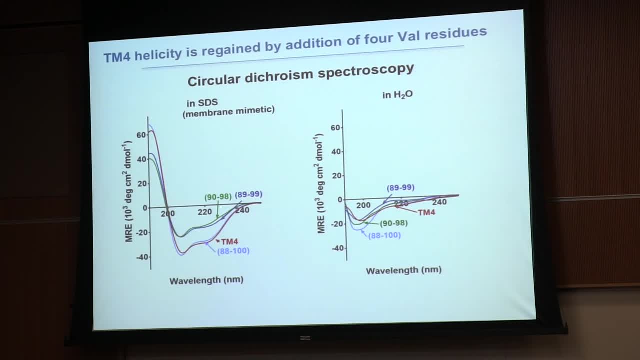 that the 90 to 98 and the 89 to 99 are helical in the SDS, but not as much as the natural TM4 in red. But the 88 to 100 suddenly jumps to the high helical value. So in other words, 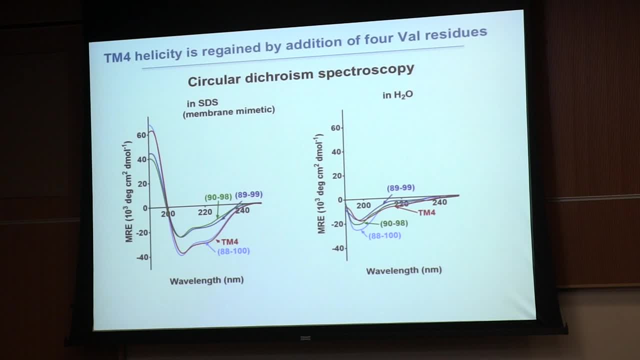 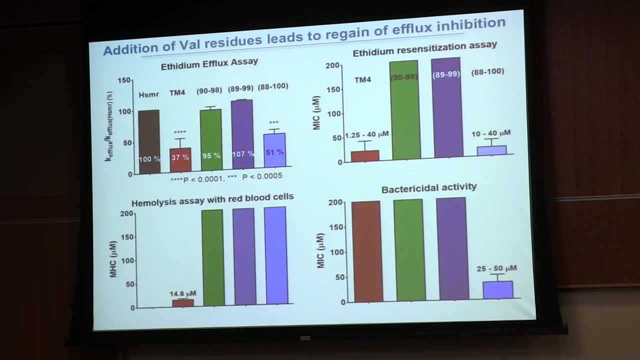 by making it just exactly that long, we're able to have the same amount of helicity. So that's a good sign that it sounds like this thing is penetrating into the membrane. So here's these bar graphs. They're very hard to read. 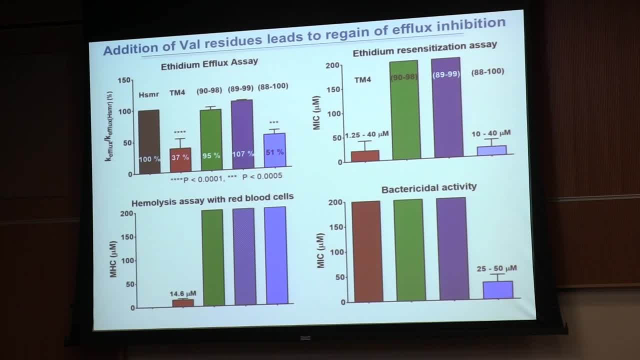 I'll just tell you in like one minute what this all means. In order to test whether these things are very useful, we did four types of experiments, and you'll see what each one. First of all, we did the ethidium efflux assay. 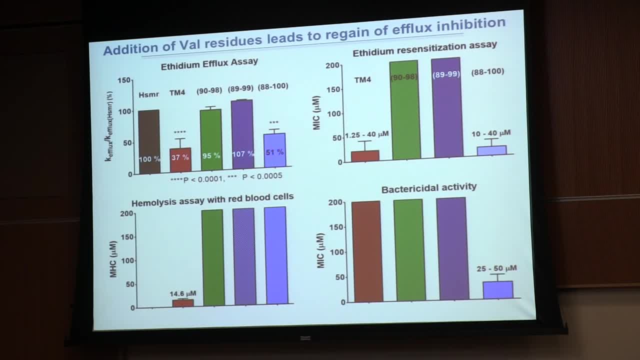 That's just the one you saw with the two things coming down. So here's our SMR set at 100%. So we saw the TM4 inhibits quite a bit. Then we found the 90 to 98 and the 89 to 99,. 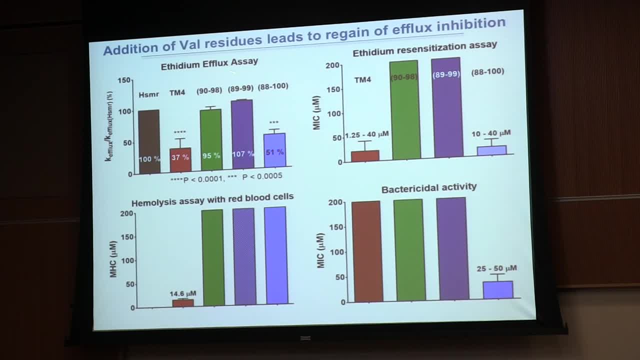 as we found now, don't do much of anything, but at least the 88 to 100 is down to about 50%. So that means in principle at least it's working. So now we did what's called the resensitization assay. 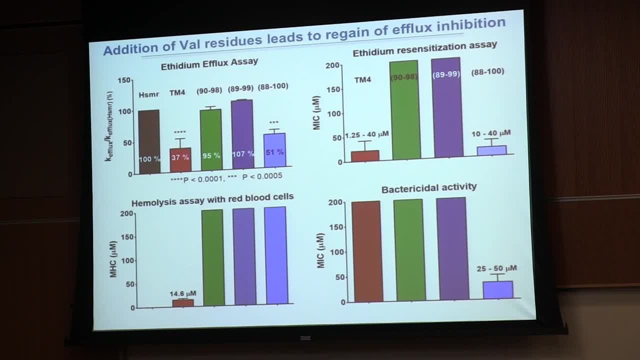 and all you do here. instead of doing the kinetic thing with the efflux, you just incubate the bacteria overnight with your peptide of interest and you see if the bacteria are dead in the morning. And if they're dead then they're down here. 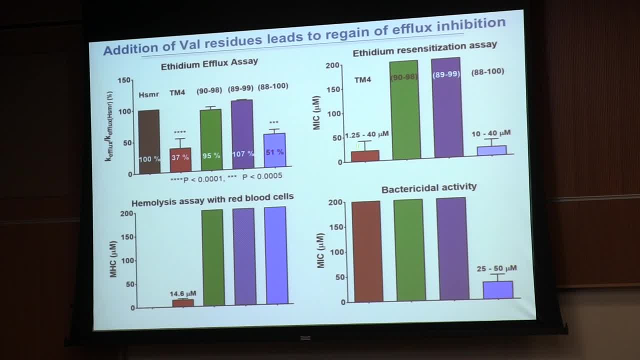 because it only takes 1.2 micromolar from the TM4 to kill them And the 88 to 100 worked pretty well. The other two nothing. The bacteria just go on living. So you can see right away from this. 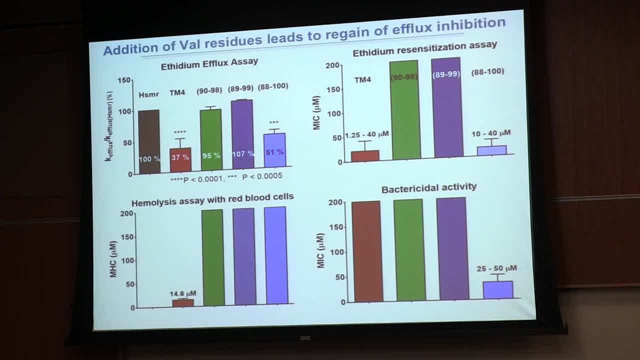 the 88 to 100 is really the minimum length that's going to work here. Then we got a real fun day in the lab. here We found in a hemolysis assay- remember that thing with the red things- Our TM4, the original one that I described. 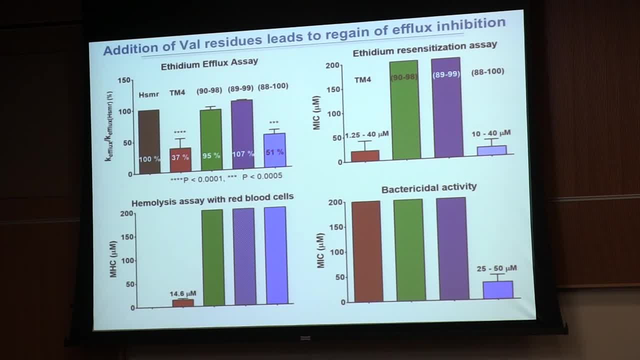 killed every red cell I touched, Really poisonous, You know. all right, You know the first sense is: well, we tried, you know That was not a good thing at all. But the other three, including the 88 to 100,. 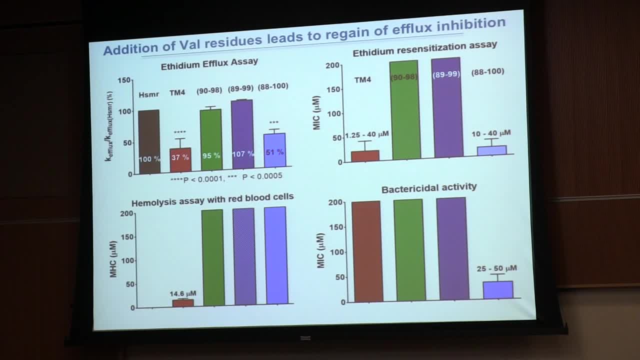 have no effect on the red cells. So at least got to reprieve And in another assay you can study these things just as bacteria, The way you do the MIC assay. you just see if it's an antimicrobial peptide or not. 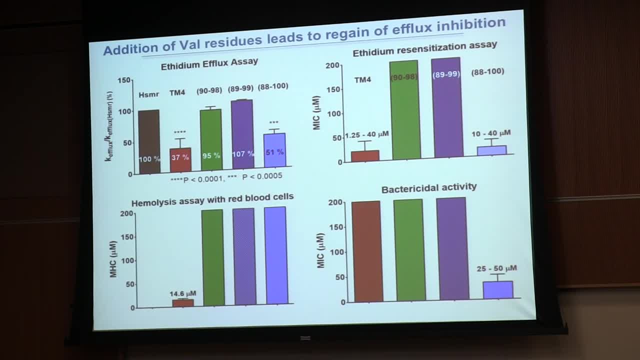 despite the mechanism of disrupting the SMR, And in our case it looks like the 88 to 100 works pretty well just as an antibiotic. And that's not necessarily what you want, because if it's an antibiotic mechanism it could be evolving resistance. 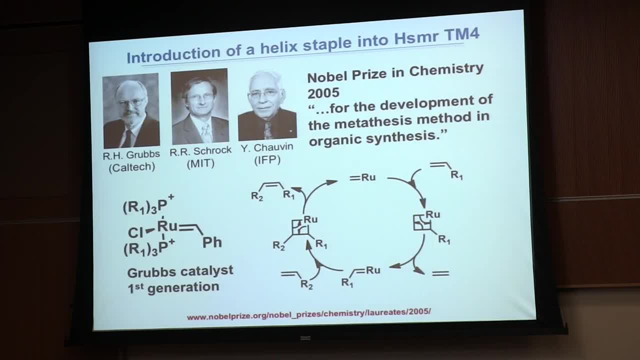 But that's a side thing. So we did one more thing that I'm going to tell you about here, which is where this work is really at right now, the last couple of months or so. There is a reaction that is called the Grubbs metathesis. 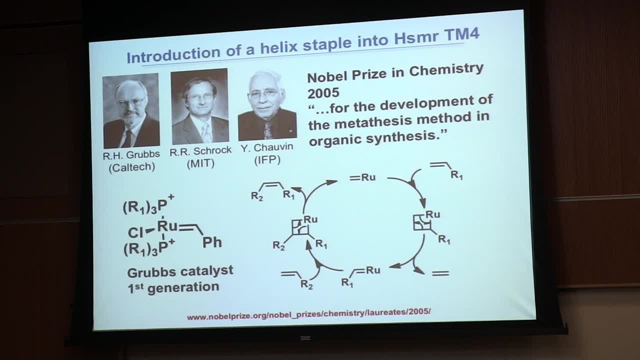 And my organic chemistry is long behind me and I'm looking at Chuck here. But this catalyst, basically it takes. you know it takes a lot of time to get to the point where it's not, But it takes. in summary, it takes two unsaturations. 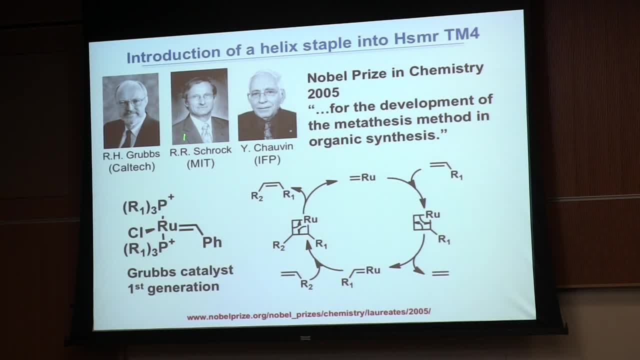 let's say R2 here and R1 here, and it goes through a cycle which creates an R1, R2 olefin between the original two separate ones, And this leads to the introduction of what is called a helix staple into a peptide. 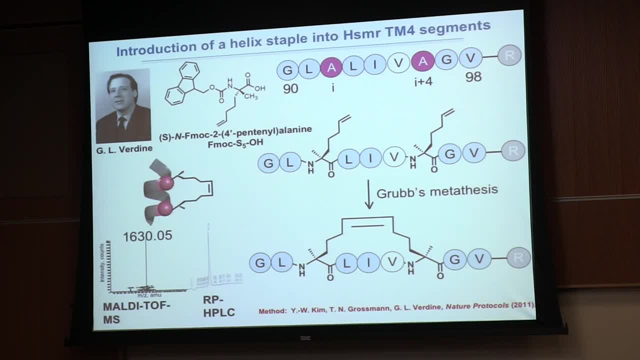 And Greg Verdine pioneered the use of this for peptides, not just the organic molecules, but peptides specifically. And what you have to do during the synthesis: you have to get this commercially available pentenyl alanine, which has not only the methyl group. 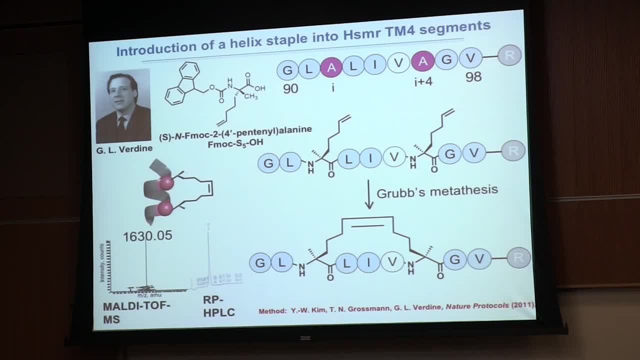 but a side chain that comes out like this with a double bond on the end. So you see, you've got the R1 double bond and the R2 double bond. That's the idea of this, And what you want to do is use this Grubbs ruthenium catalyst. 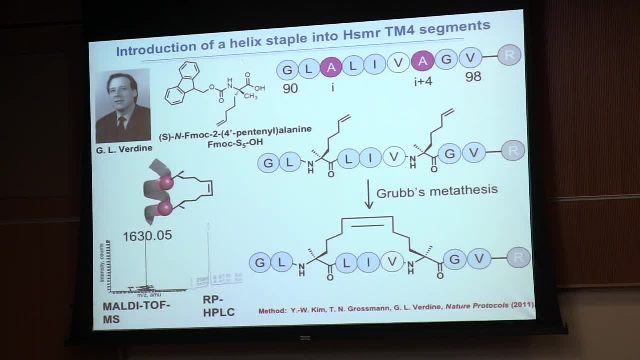 with these two here And you can try it. We tried it first with the 90-95.. And you get a peptide that looks like this, And now you have an olefinic bridge in the middle And actually this peptide is now more hydrophobic than it was before. 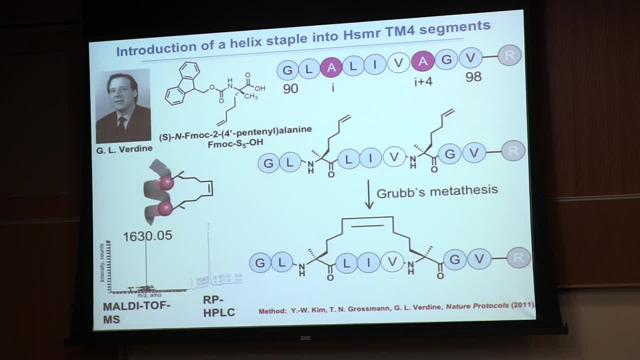 because you have all of this CH2, CH2, all of this stuff. It makes a very interesting compound, But the idea is to freeze out the geometrically crucial TM4, TM4, heptad, so that it basically, if you choose the positions of this and this, 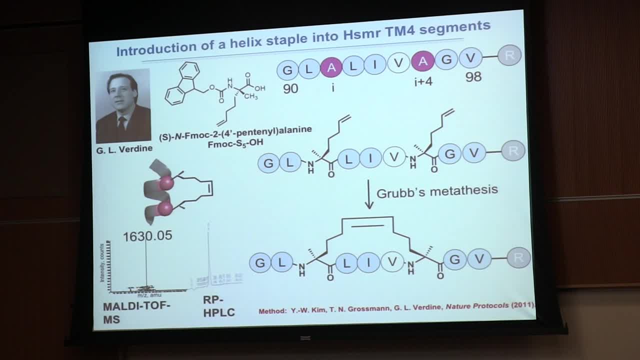 the two alanine derivatives you can freeze out the geometrically crucial TM4, TM4 heptad. So you go one turn of the helix, you lock it in on one side and then the backbone over there is exactly right for the helix. 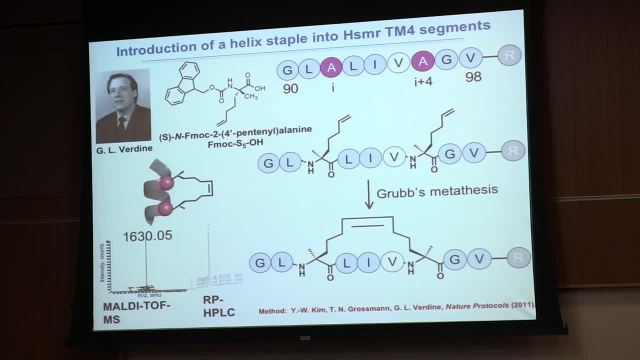 that's going to interact with the TM4 in your competition. So that's the idea. These have been used in pharmaceutical circles now to do just that: to freeze out the pharmacophore of interest. First time it's been applied to membrane peptides, to our knowledge. 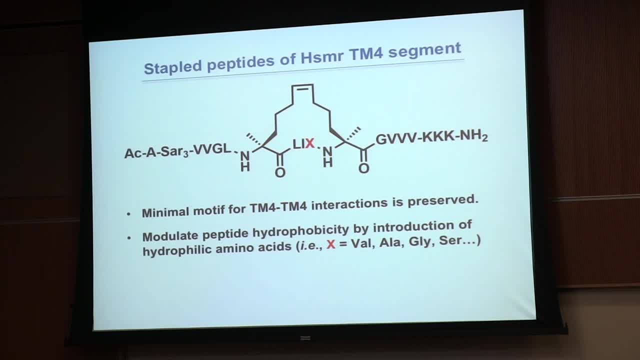 So now we know the minimal motif. It needs to be 80 to 100. And we can operate on some of the residues within that heptad section, because those are not the ones that are evolutionarily conserved. So we can, for example, take an X residue here. 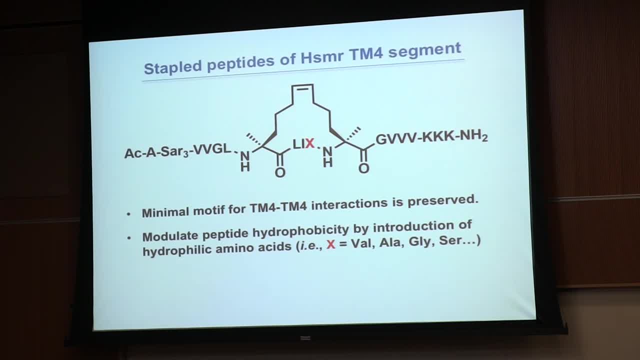 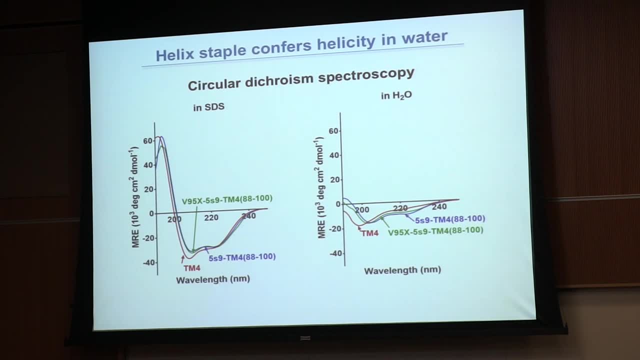 and change it from the wild type to veil or allergly or serer, basically anything we want to do. And we made some of those stapled ones, without going into too much detail. They are suitably alpha helical, But you'll notice here that they're starting to take on a little bit of helical character. 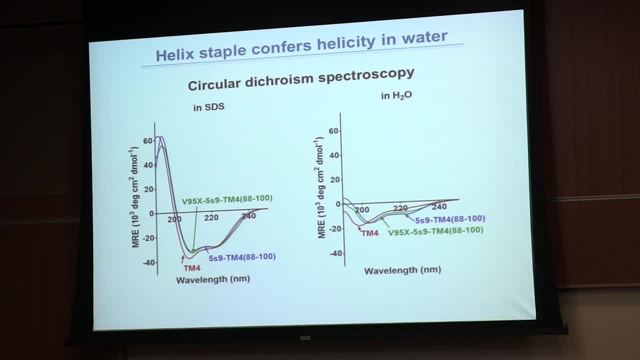 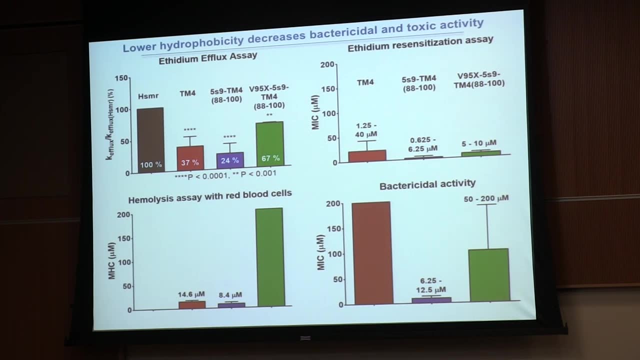 even in water, which gives you an example that the conformation is stabilized. And now we've got some good results with here. This one, here the stapled one I'm calling V95X inhibits 67% in that efflux assay. 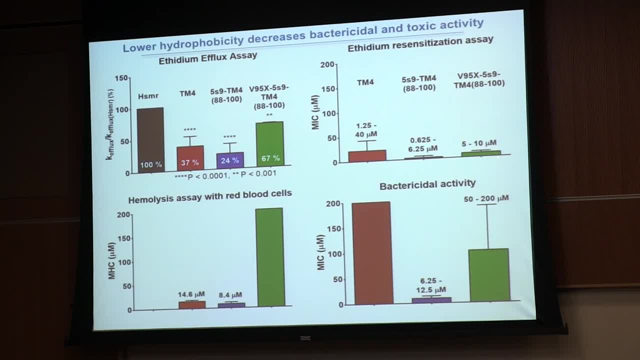 but now it's down very, very low over here. So this is a great one for killing the bacteria. Re-sensitivity- And here's the good news, This one is not hemolytic. It's hard to predict which ones will or won't sometimes. 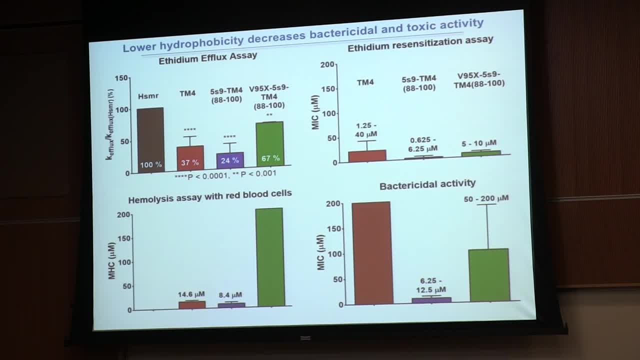 And it has a little bit of bactericidal activity. So we actually have an inhibitor here that fulfills essentially almost all four of the criteria that we're after, And we think we're on the right track to make a really good inhibitor here. 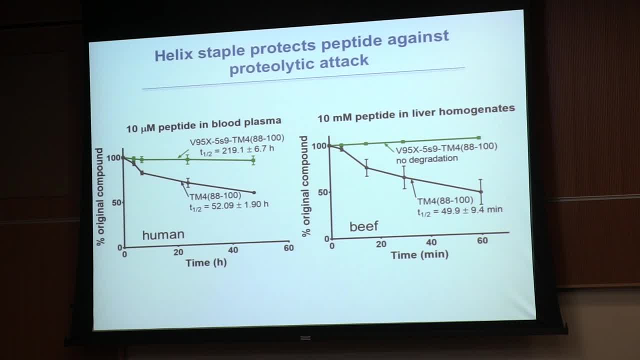 So this is something like they say in the movie. in the movies, you know, it just might work. The most recent data on this shows that the helix staple protects the peptide against proteolytic attack And in blood plasma samples, the liver homogenates. 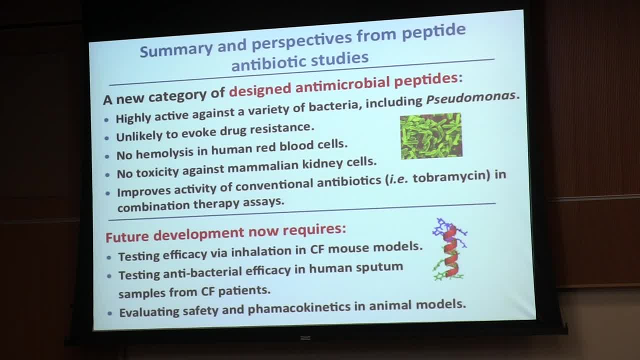 The lines stay right at the top, It means that they're not being metabolized, So that's very preliminary. So, to summarize all of what I've been telling you, here we have a new category of designed antimicrobial peptides that are highly anti-inflammatory. 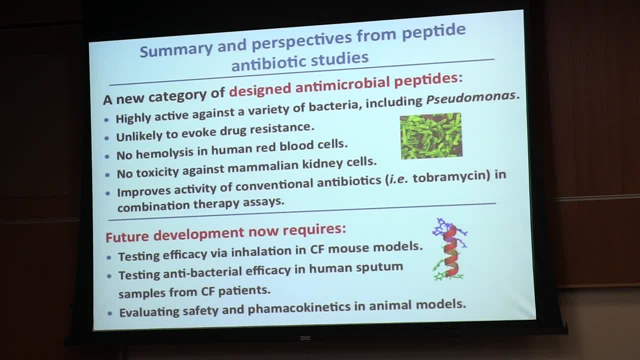 They're highly reactive against a variety of bacteria, Unlikely to evoke resistance. no hemolysis. We tested different types of African green monkey cells. There's no effect And it obviously improves the activity of conventional antibiotics and the conventional therapy assays. 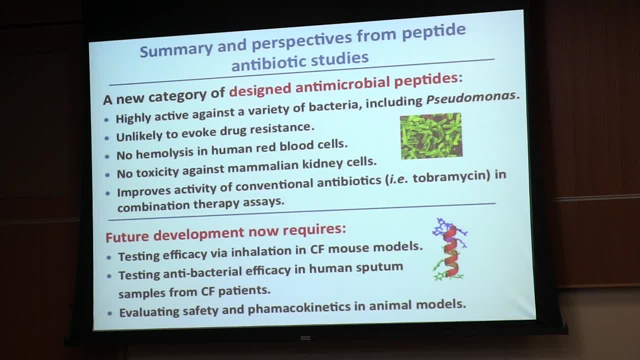 So now we have to test the efficacy of this in CF model mice to see if they can inhale it and kill an infection. We have to test their efficacy in human sputum samples more further than the couple of trials that we did. So we have to test their efficacy in human sputum samples more further than the couple of trials that we did. 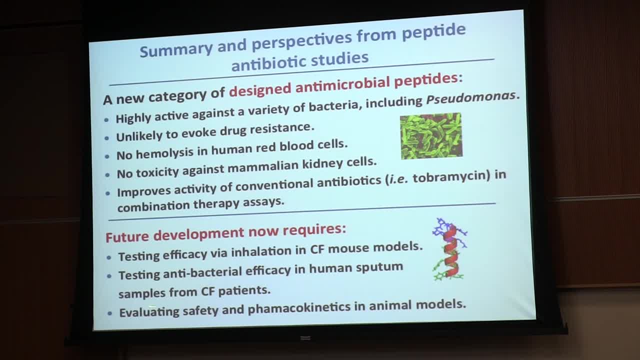 So we have to test their efficacy in human sputum samples more further than the couple of trials that we did. So we have to test their efficacy in human sputum samples more further than the couple of trials that we did, And this is something which is a big deal, very expensive. 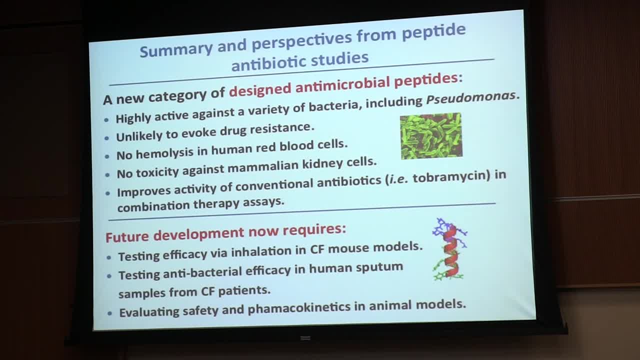 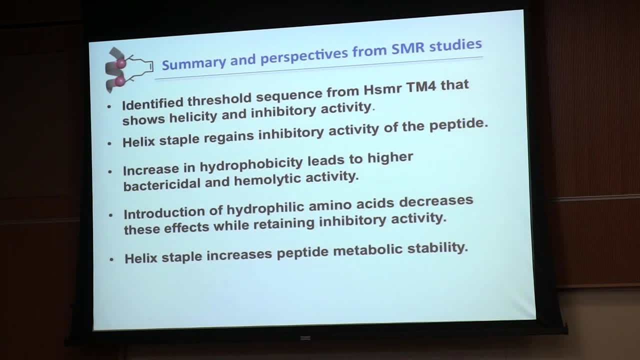 You have to evaluate the safety and the pharmacokinetics in animal models before it can go further. As far as the helix staple is concerned, I think we've identified a threshold sequence from a TM4 that shows helicity and inhibitory activity both. 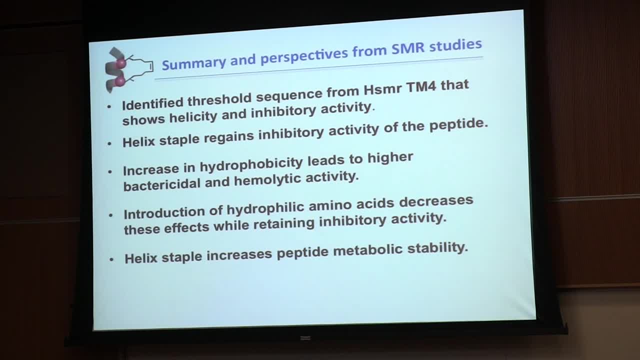 It retains the helix staple then retains the activity. The increase in hydrophobicity leads to bacterial and hemolytic activity. So we can put hydrophilic amino acids in the X positions and find just the right balance. And the staple increases peptide metabolic stability. 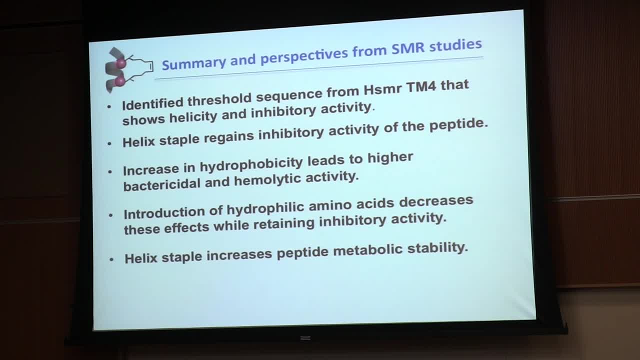 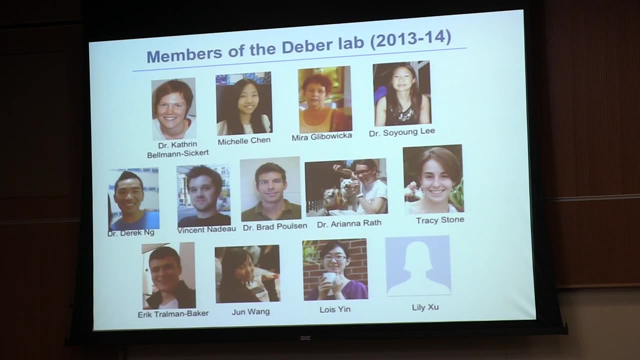 So these are two examples of things that we think can actually confront bacteria And with the appropriate amount of R&D they might in some way, some future time, actually prove useful. This work is a lot of people behind it. I get the chance to present it. 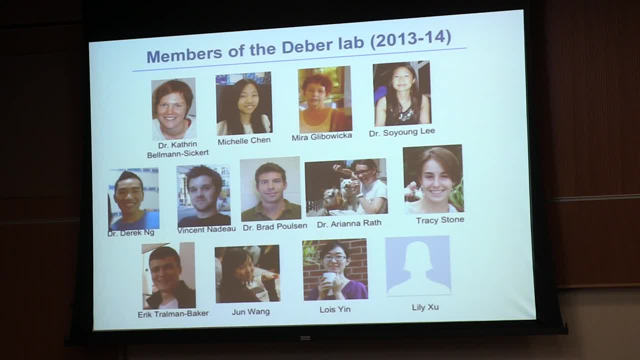 but I'm really very thankful to the members of the lab And in particular, just to mention: Catherine did the staple work that I just described And Brad Polson did the original TM4 work with the SMRs. Arianna Rath was involved with the CAPS work. 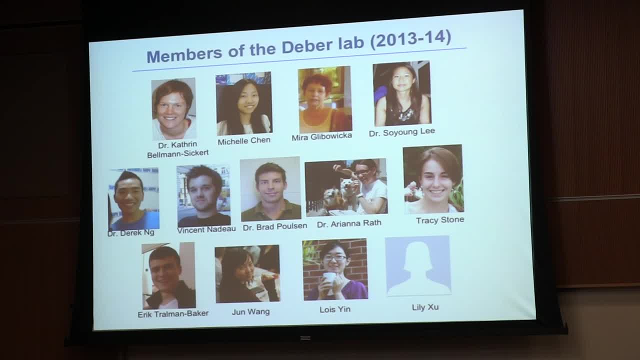 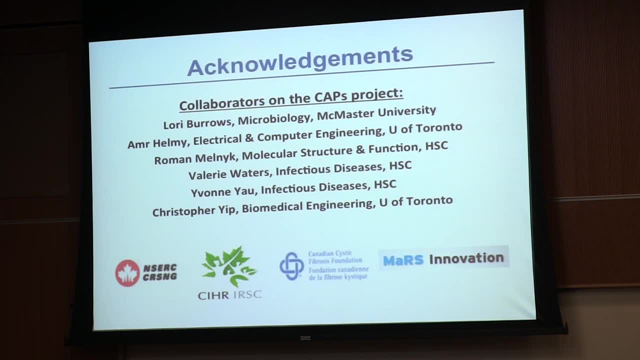 and Lois Yen did a lot of the testing and the combination therapy especially, So I appreciate their contributions enormously, And especially on the CAPS project. as you can see from this list, we had collaborators that came from many different walks of life. 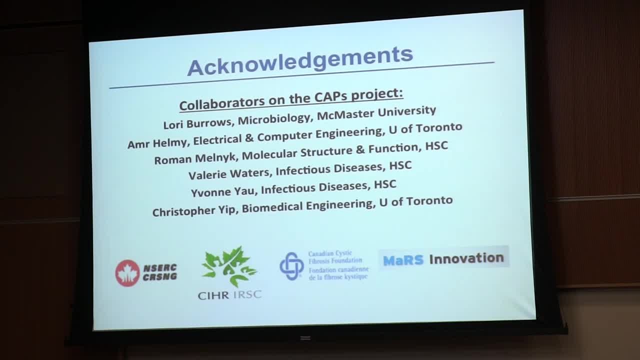 I'm certainly not a card-carrying microbiologist, to say the least. So when you start working with bacteria, you learn a lot of things you didn't know. For example, lysine got its name from the word lysis, which means that it blows up everything. 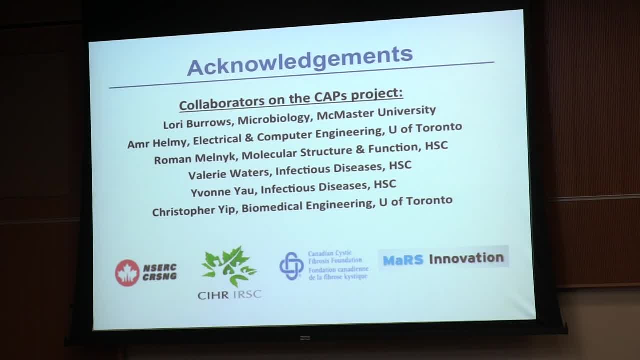 When I first told my microbiology collaborator, Laurie Burrows, that I had peptides that were good antimicrobial, she says: does it have lysine? I said yeah, yeah, it's got six of them, Like that was good. 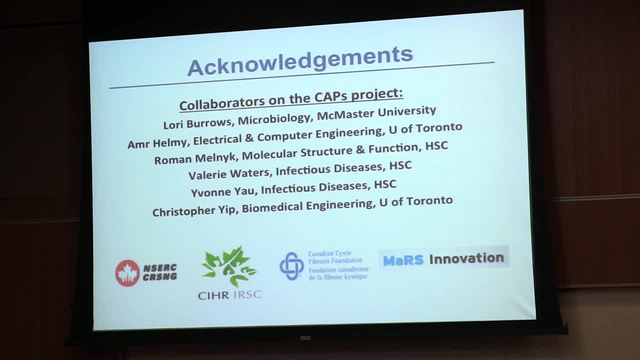 She says that's not good. So it turned out from what I showed you that if you choose the peptide right and you don't make it too hydrophobic, it doesn't lyse the human erythrocytes. So that was part of the R&D that went into this. 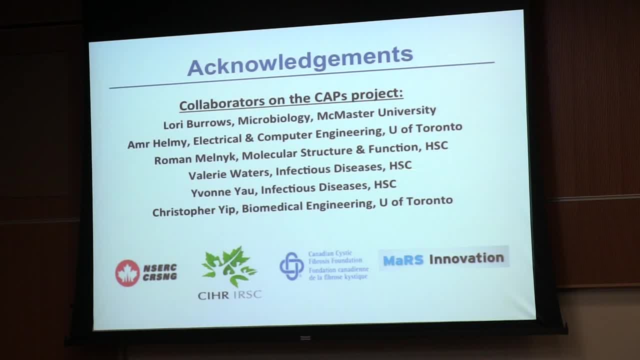 We've worked with the computer engineering guys, the molecular structure and function, the infectious disease guys, the atomic force microscopy guys, all trying to bear the maximum kind of information on the project And I thank these funding sources and I thank you for your patience. 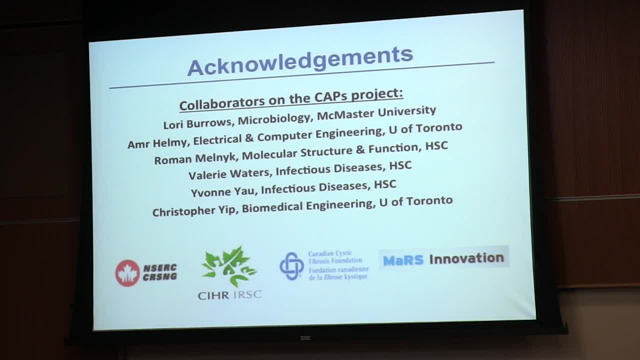 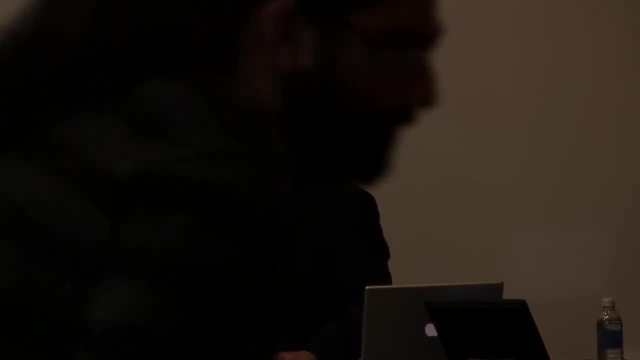 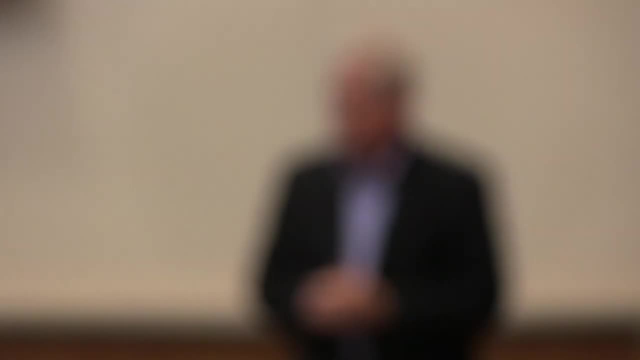 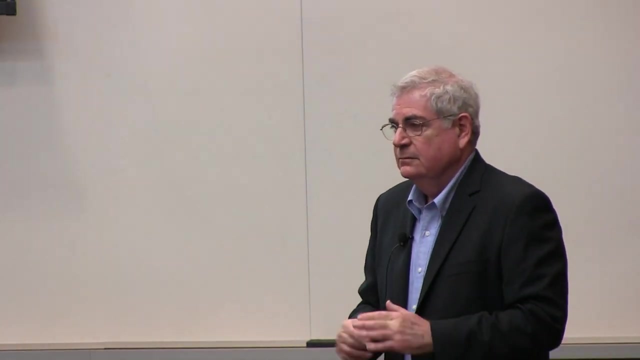 Thank you very much. Question: Yeah, With regard to the peptide. stapling peptides, I think, sometimes stabilize the appearance right, So you can try to shorten the peptide. Can you try to make shorter peptides that are stapling and see if they're still active? 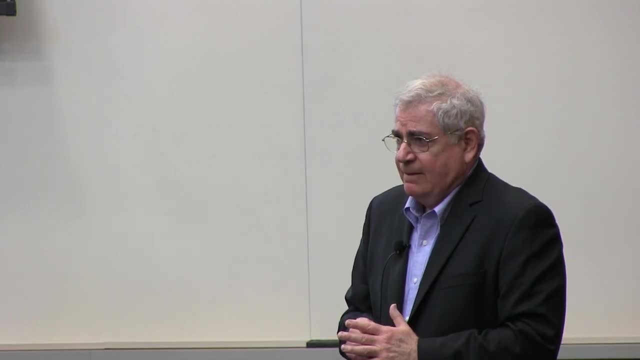 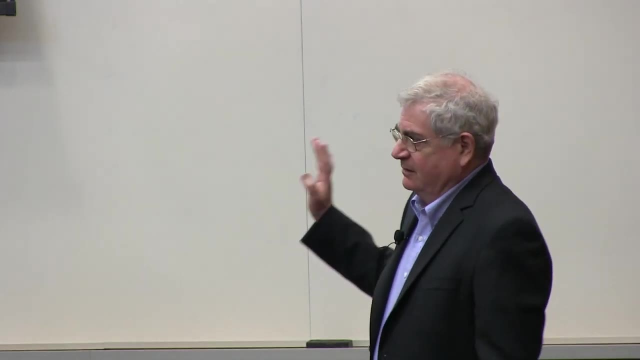 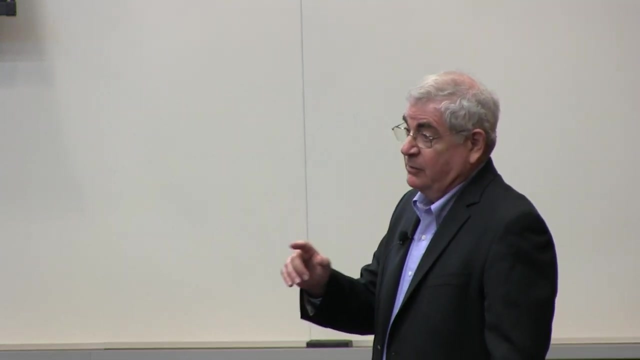 We did several combinations of those And they were all put through these four-panel graph things, So the one I showed you was just the best one of those, But you are right that it might be possible to make a shorter one, Yeah. 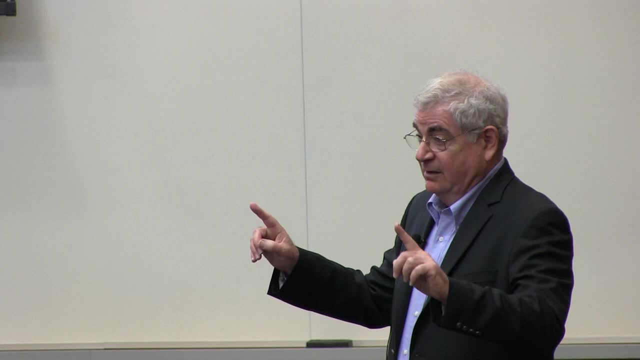 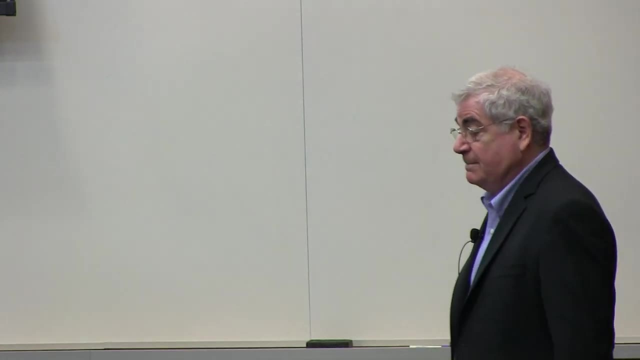 You can also make a longer one. I'm going to put this staple one in seven. We might be able to capture just the peptide with that. There's a lot of theme of variations possible with that. It's a good idea. Question about the lysine. 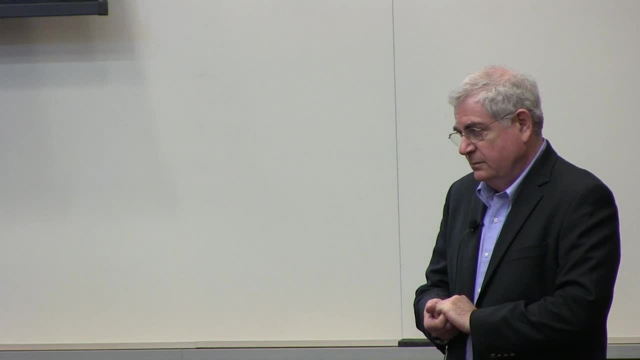 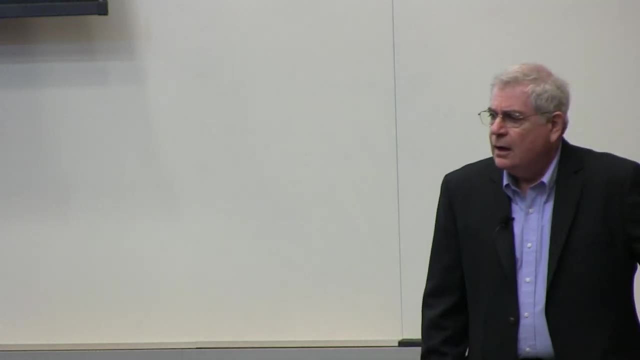 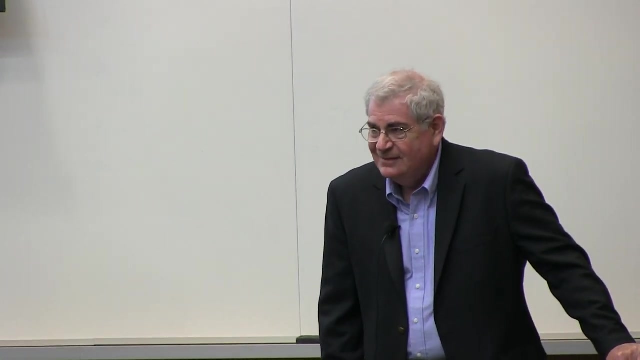 Do any of your peptides have a curative form of that? If you're having two positive centers 10 atoms apart, I don't curare. My question is about a curare form of- I don't know what that is- If you have two positive charges, 10 carbon atoms apart. 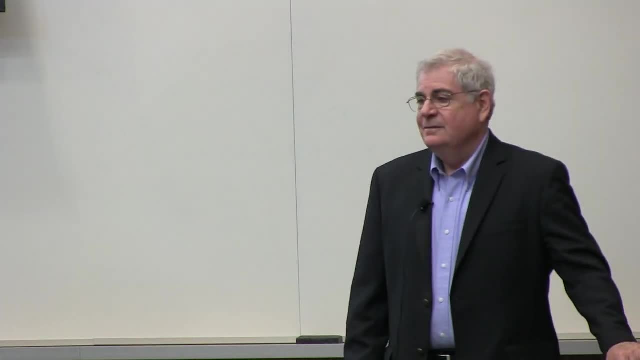 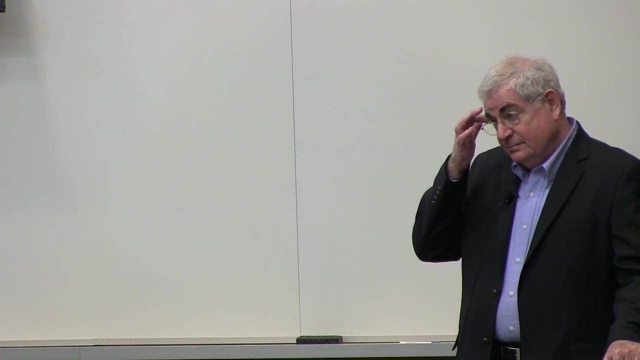 you can paralyze the neural muscle junction And so those lysines, some of them, are great on the bacteria since they don't have a neural muscular junction. But if you try it on an animal Right, Is there anything you have to do? 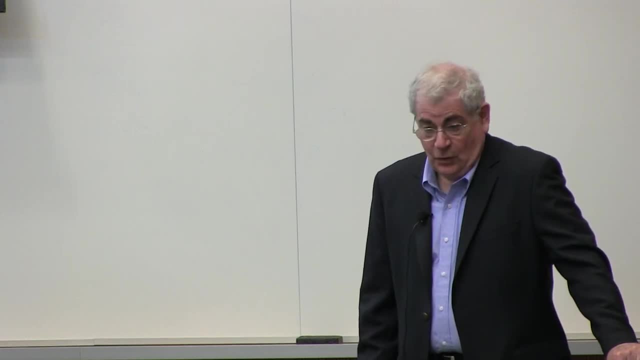 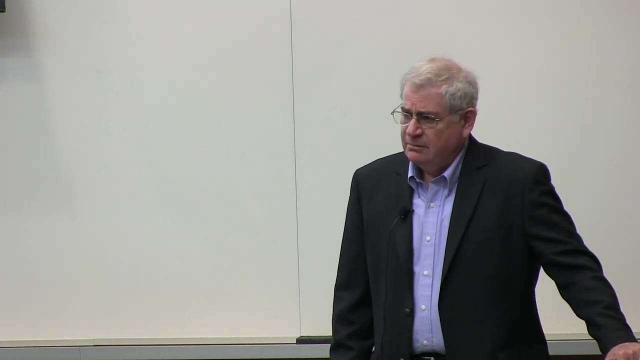 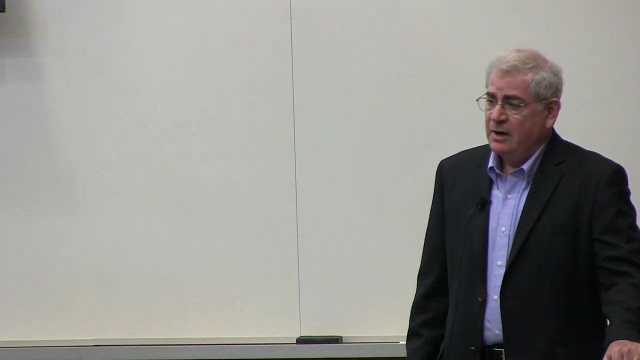 That is possible. Is there anything you have to do? No, No, we haven't really done much on that. We did one of the 6KF17s in a mouse model CD1 mice. This is not my expertise. The person that did it said that up to 10 times MIC. 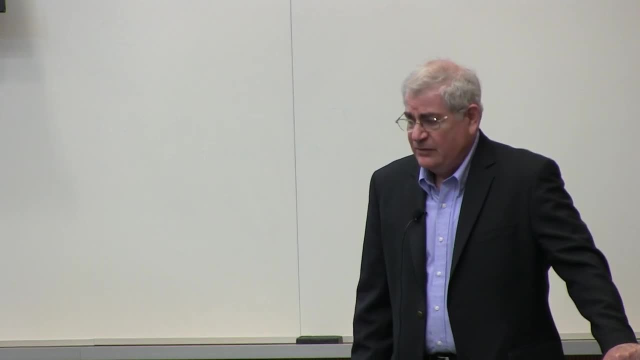 there was no detrimental. That's all we have, But that's way too soon to. We got to try all the D residues And yeah, There's a lot of stuff. Another question: That's a good point. You talk about the membrane, but it looks to me 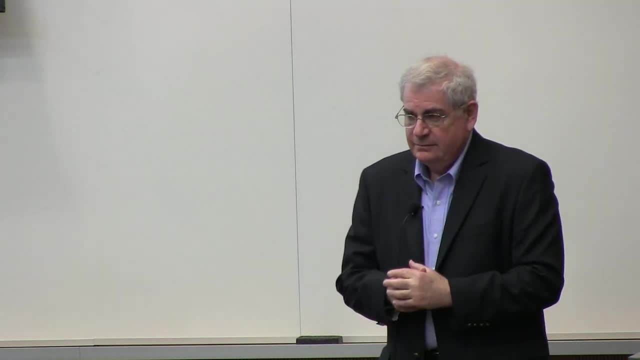 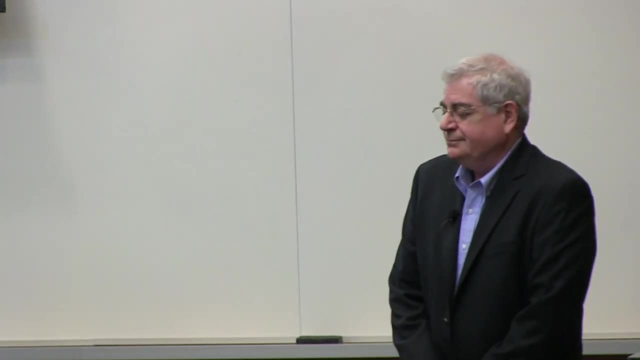 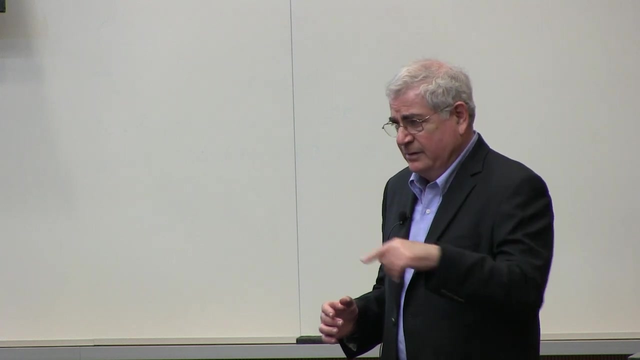 like you're concentrating on the outer membrane, But then what happens when you get to the inner membrane, Especially when you're in comparison between the? Yeah, that's a good point. Yeah, so the question is about some bacteria have like a cell wall and then a membrane. 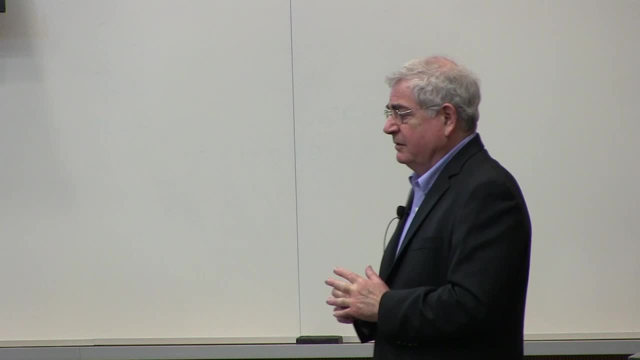 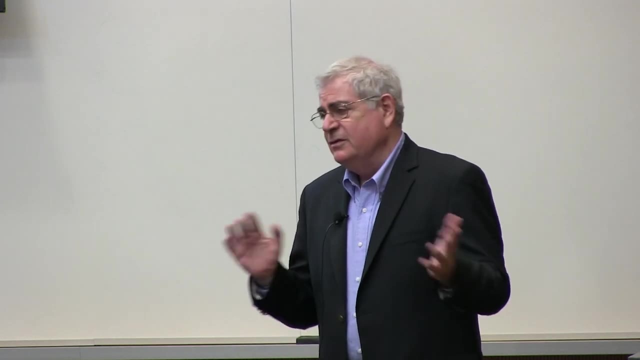 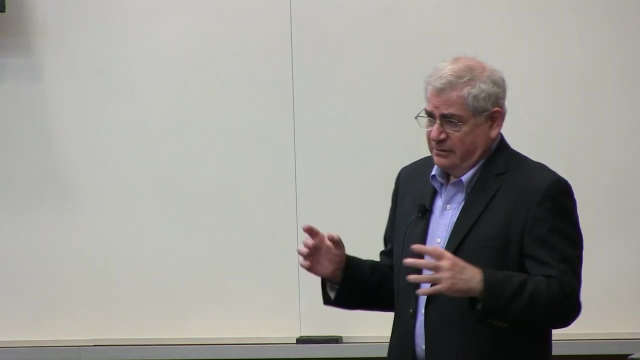 Yeah, it for some reason known only, And not me anyway. Everybody ignores this cell wall, Whether the bacteria are gram positive or gram negative. they just look at the plasma membrane of the bacteria And that's where all these pumps are and everything. 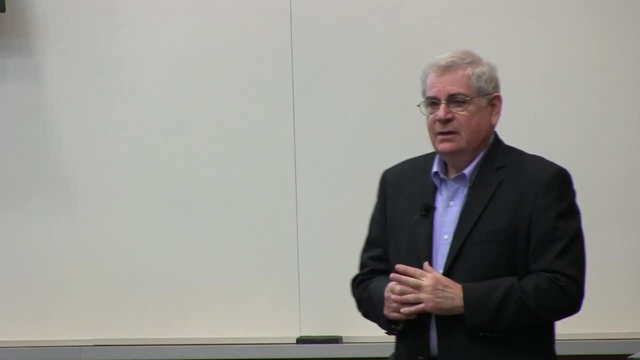 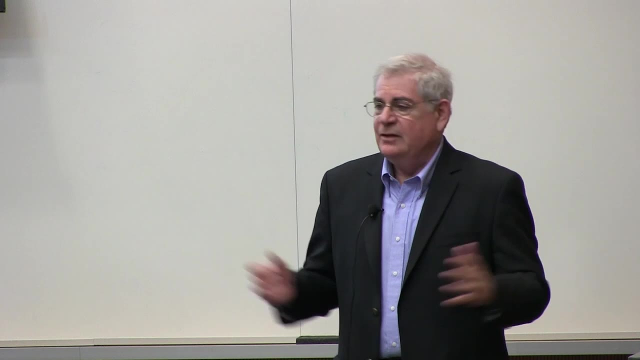 And it is kind of enigmatic in its own way how all these incoming peptides, how they get through the outer part. But that seems to be, oh yeah, they'll get through It's. maybe it could be that the outer wall is. 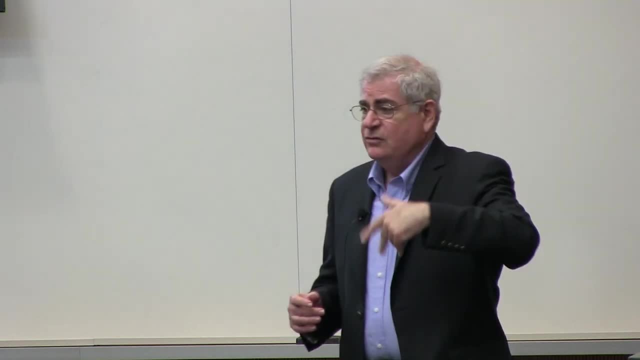 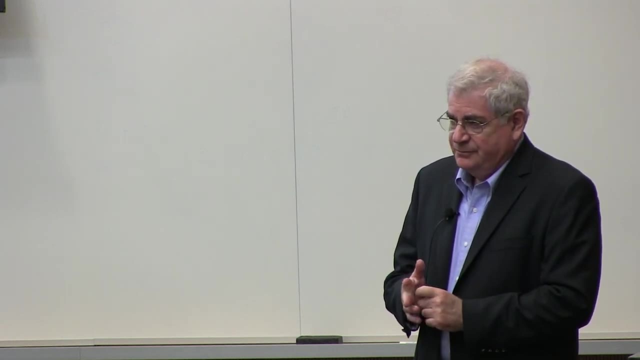 intended to be porous, Because I guess there's an exchange of ways. What about the wall membrane? There's two membranes: an outer membrane and an inner membrane. That I'm not. you mean which in the gram? The gram negatives, The gram negatives, yeah. 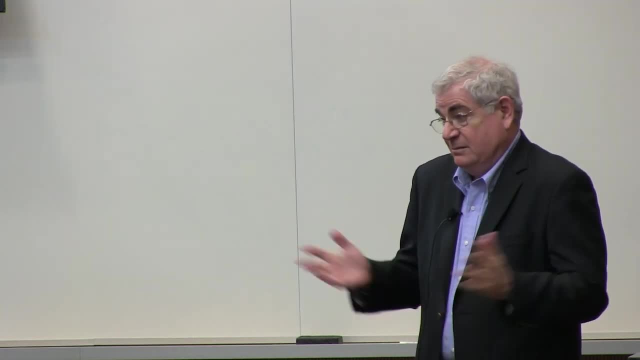 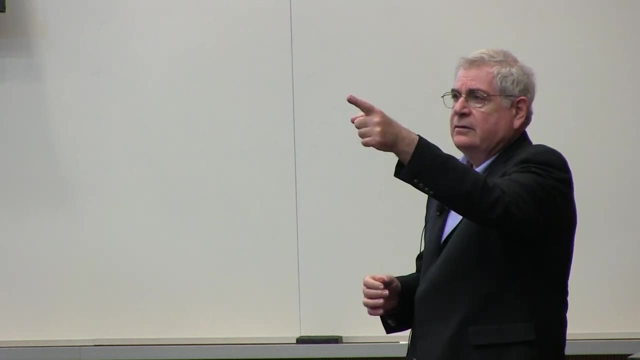 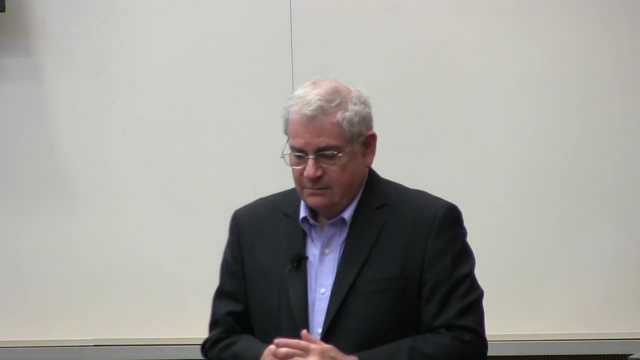 They just make it. No, they're. What was the other part of your question? The other was: OK, Oh, here, Sam. yeah, So you described the design hypothesis Right. You said that you're going to structure the positive. 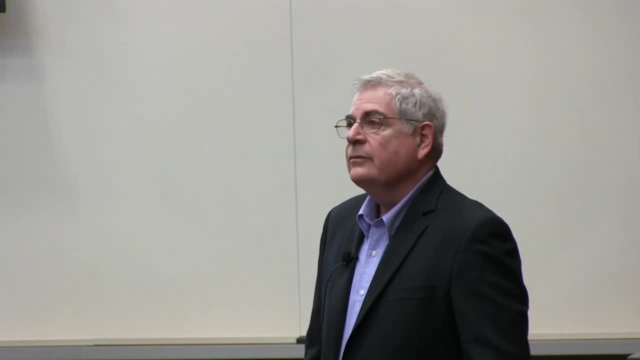 spectrum to the one end and not polarize it to the other end. Have you tested that hypothesis by making isomers where you gather the positive and the non-polar? But they didn't make it, So I feel like you're going to gather them all the way. 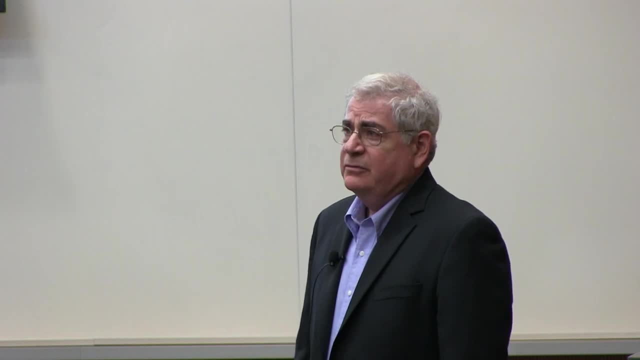 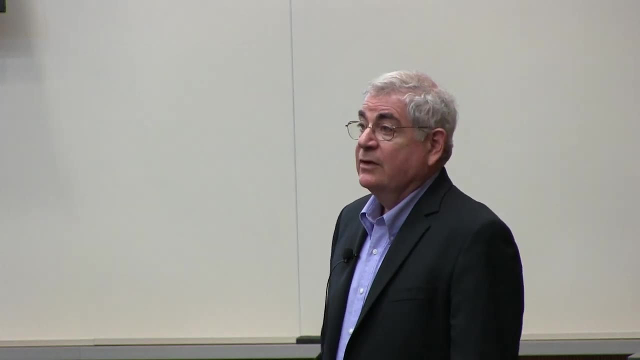 Yeah, we got 20 or 30 different versions of these things, some of them with the lysines in the middle and some of them I showed, with the lysines on two ends. So if you point out the beginning, those are all amphipathic sequences. 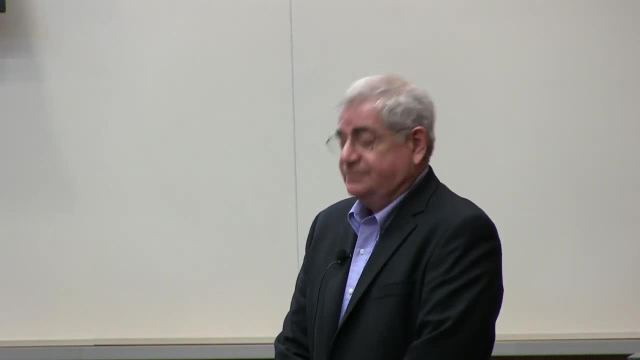 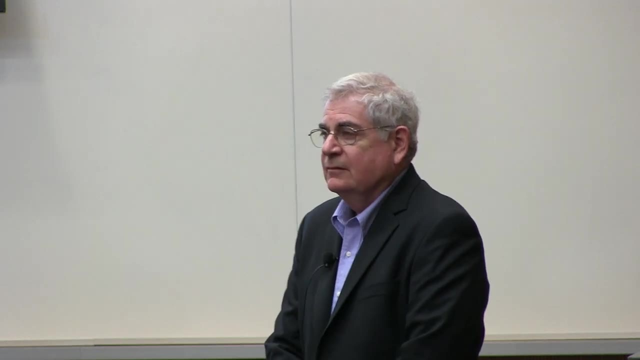 Those are all amphipathic sequences. Yeah, If you take the sequence of one of your best ones, make the amphipathic. instead of making the amphipathic to a place of a positive one, it has a cluster. 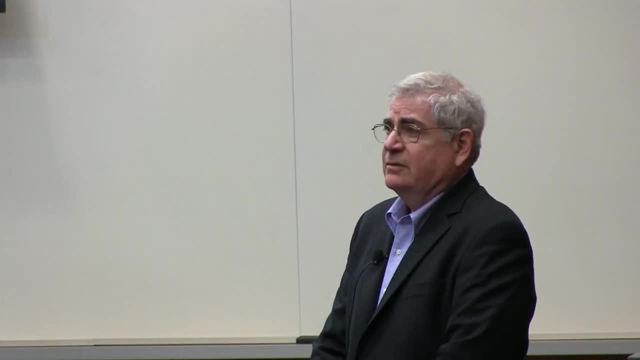 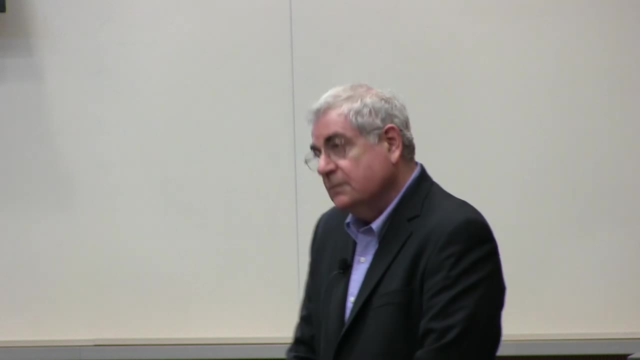 No, I haven't done that. That would be a good control to see if the principle is right. Yeah, And then another technical question: When you use the DIC measurement, is there a difference? No, You mean in the combination therapy thing. 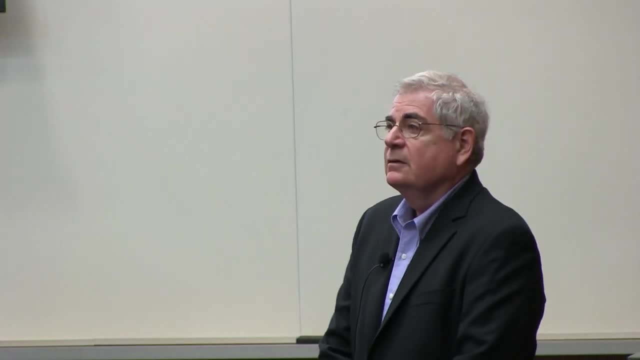 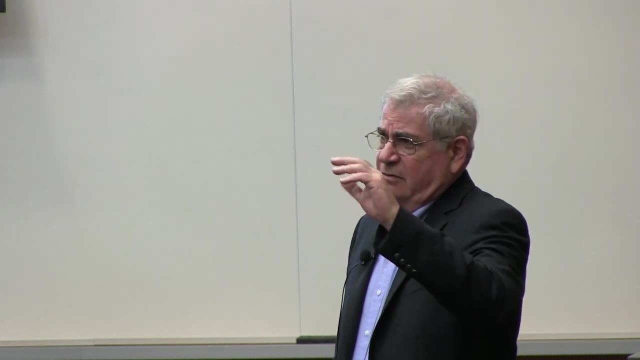 No, no, no, I'm just. There's a thing that's called the Calgary method. It's some sort of a thing with a little. it looks like a little Eppendorf tube with a cap where the bacteria are made to grow on the inside of the cap. 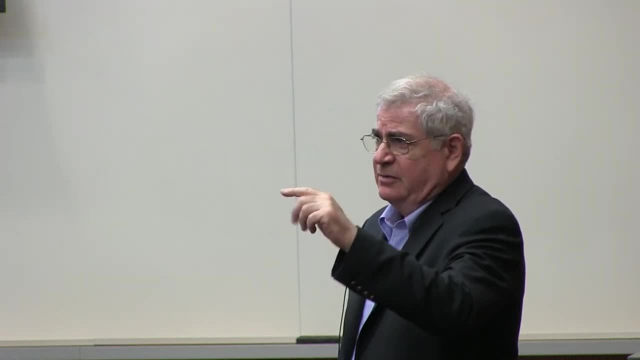 and then it's dipped into the fluids and it's some dynamic thing where the fluids can get into the cap and then it's dipped into the fluid and the peptides pass by this thing. You have to see it, It's a kind of a little mini apparatus. 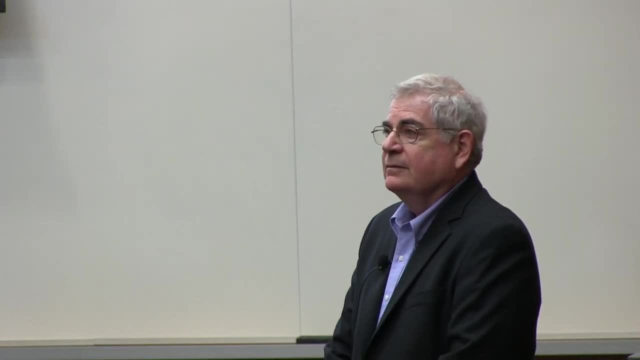 But my question is: are you testing to see whether the biofilm activities are important or are you starting with them? You're starting with them. You wait till it gets to the mucoid, To a biofilm, Yeah, And then what are you testing once you have the measurement? 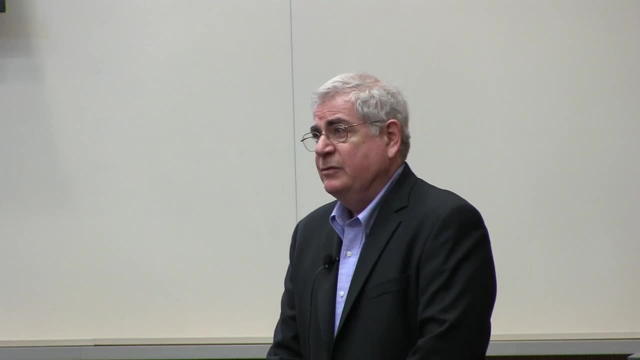 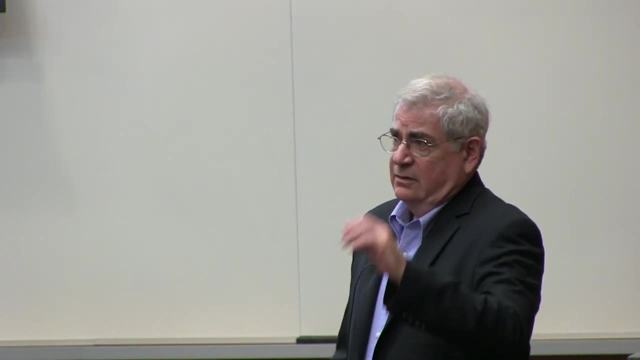 once you have the biofilm. I guess it might just be an OD, An OD measurement, or something of that sort. Or you could just visually read these caps. They're little things that look like little triangular. They can probably be read in OD form or something. 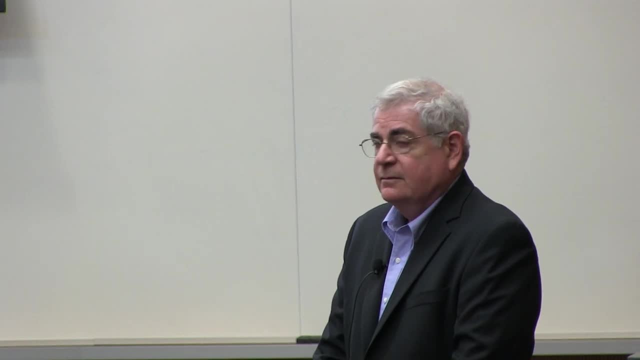 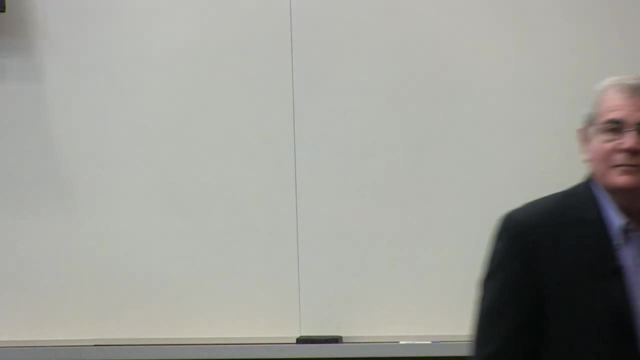 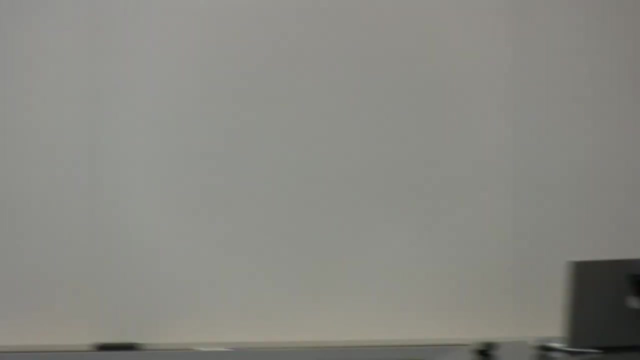 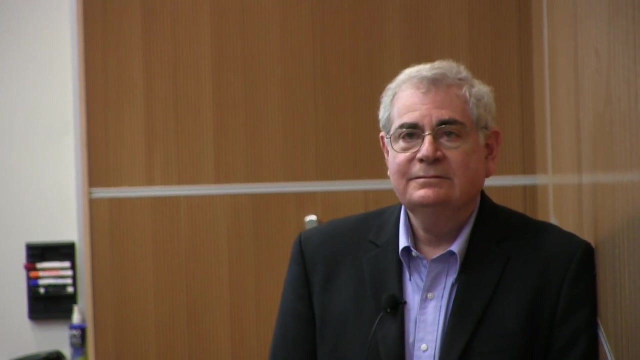 That's all right. Back there, I see someone. Yeah, Since everyone's asking two-part questions, Have you ever tested the caps against mitochondria or impacting them themselves to measure the equivalent of MIC? Nope, OK, I guess I. 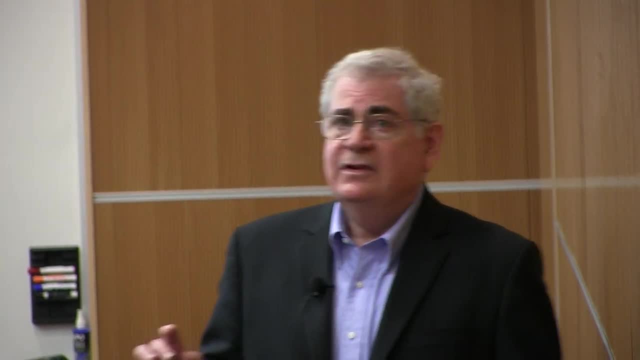 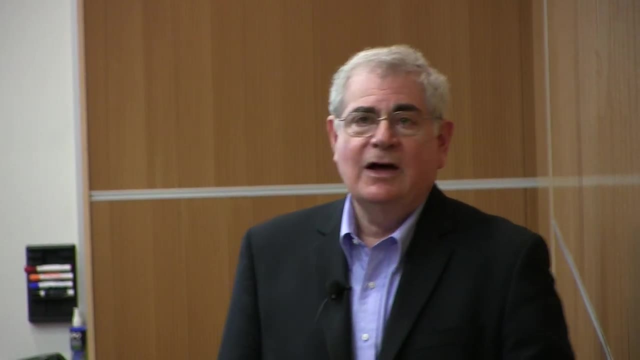 I must say, all of these types of questions, a lot of this work is in its infancy. when it comes to these Sure, You know, if these things get, if these things are tough on mitochondria, we're all we're cooked, you know. 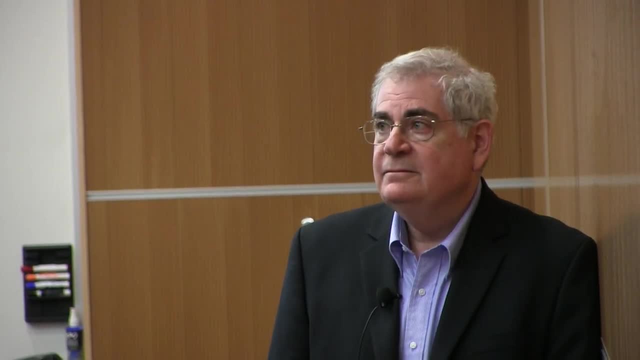 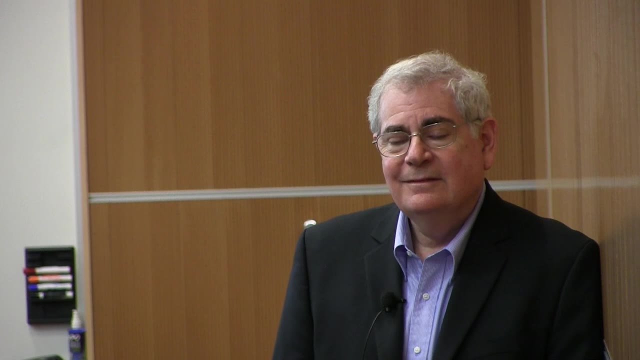 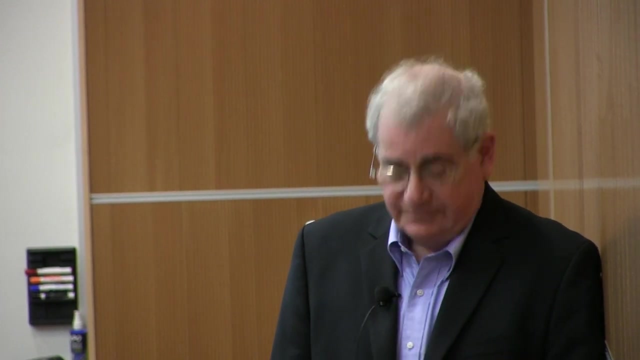 Yeah, And the other question was, I think, kind of related to Barry's question, which is when we test- and we do this ourselves in the lab- We test, you know, small molecules in vitro, but right, it doesn't really replicate the situation. 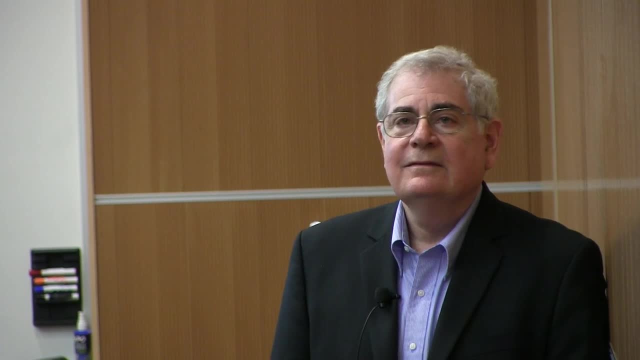 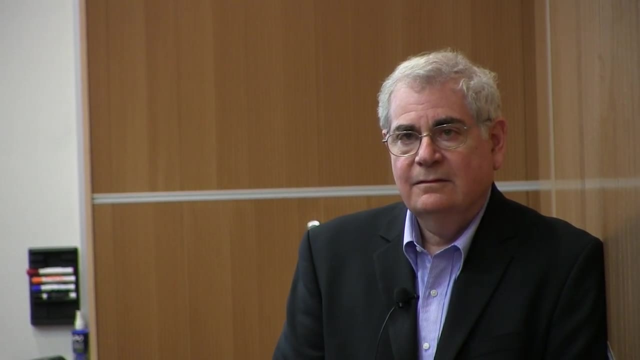 And I think the one, really the one case that really showed that nicely is a lot of them positive- is that you know you grow them in vitro like staph aureus and you know they just look like normal kind of coccyx. 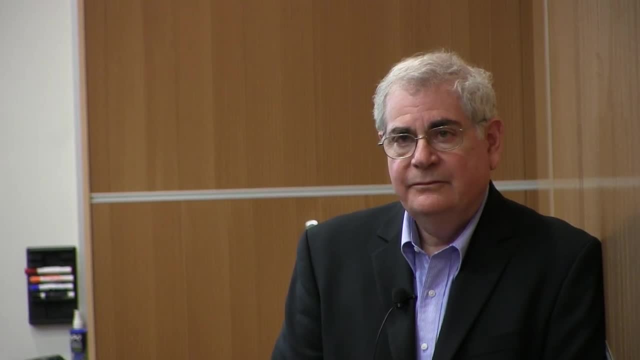 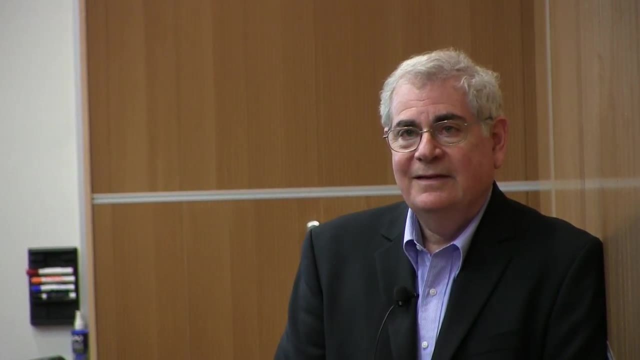 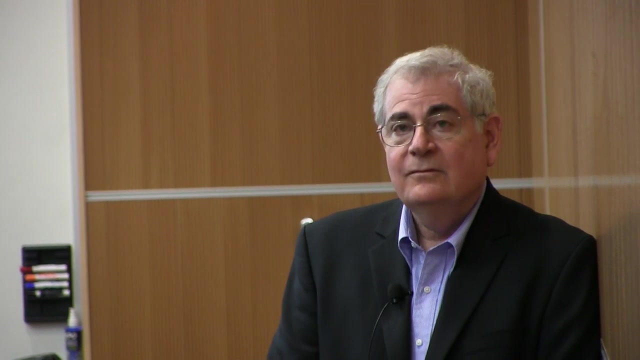 So when you grow them, like in an infection model, they grow this like incredible lipoteic acid and luteic acid structure, and it's hard to imagine anything penetrating through there, And so I'm just curious. 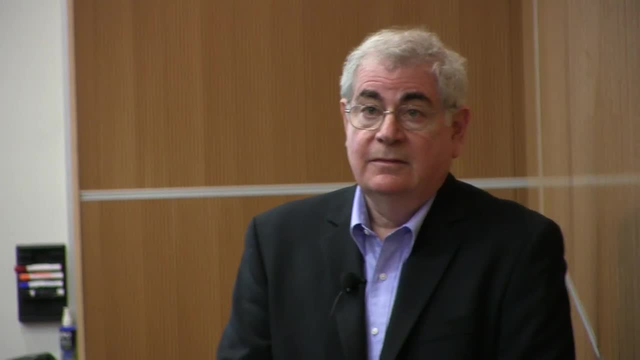 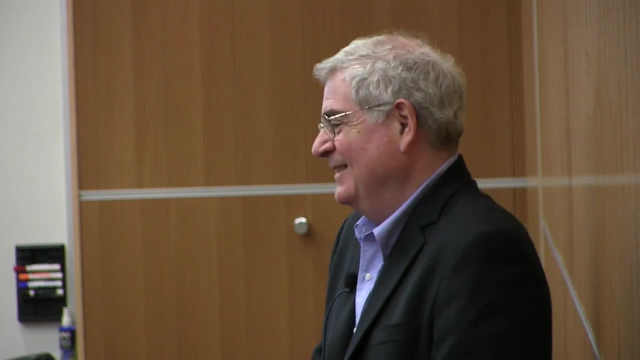 Yeah, we haven't tried that. That's something to move toward. Yeah, Yep, exactly. Well, we're the same. I mean, we don't, we never do Yeah, Okay, there was a question here. 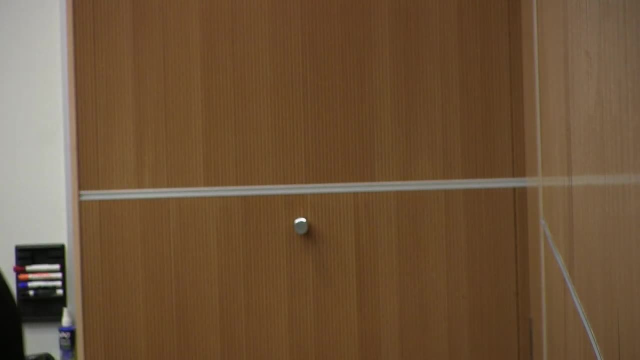 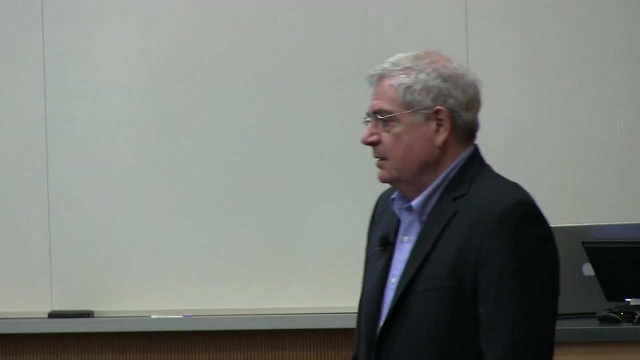 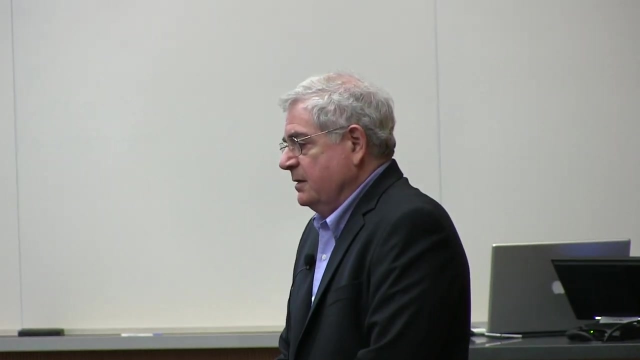 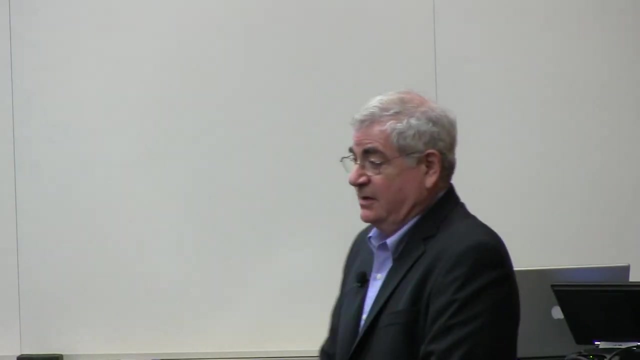 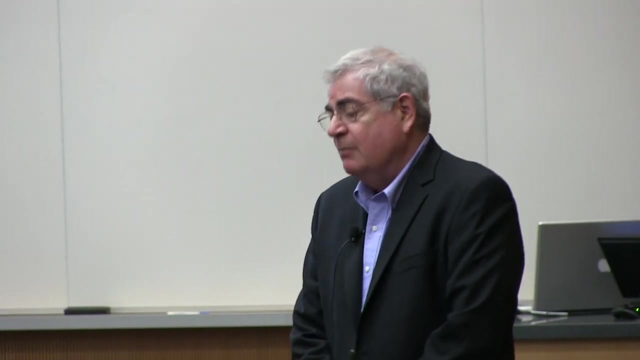 Yes, Never actually did the NMR on it, simply because, like you said, the CD is helical and all peptides like this over the years are always helical. So what we wanted to do is make a one-to-one complex. 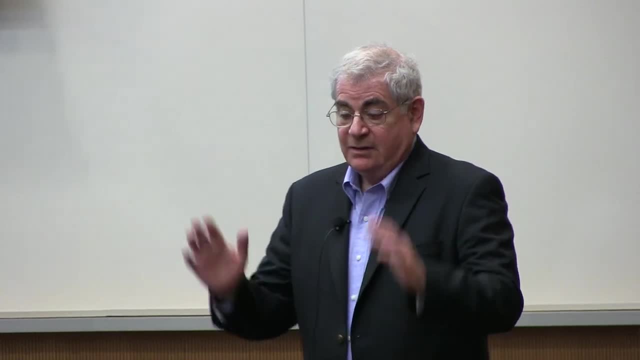 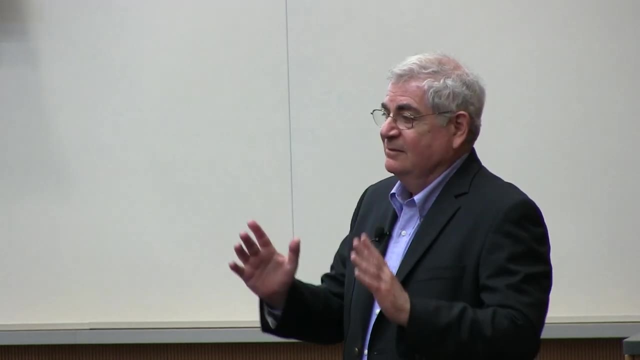 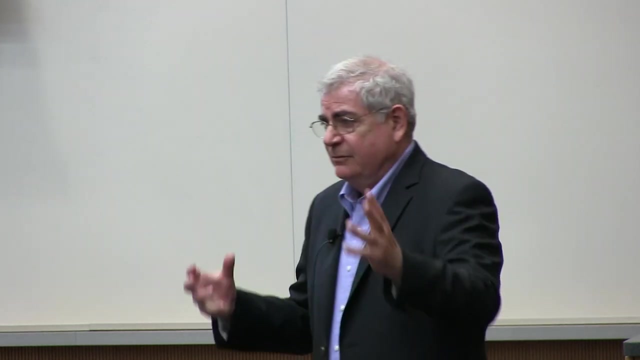 let's say, of one of the peptides with a defined segment of the alginate. like you know, five sugars and one peptide and see, you know, try to get some idea from the NMR about how that, you know, forms a specific complex. 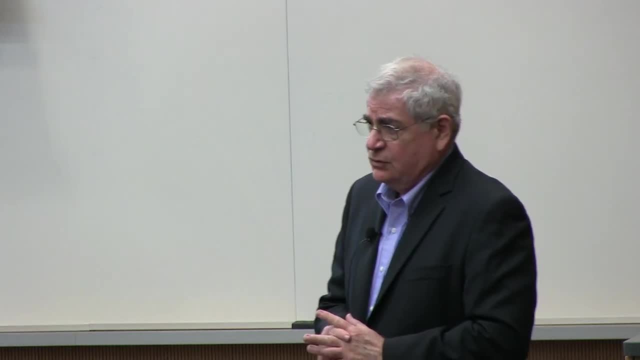 and how it might aggregate the the sugars. That is something that's it's not that easy to get the defined segments of the sugar. And about the antigen: the antigen, like you've been trying to study the effect on the meat. 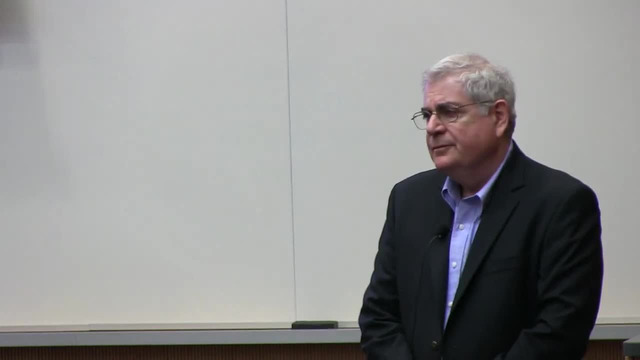 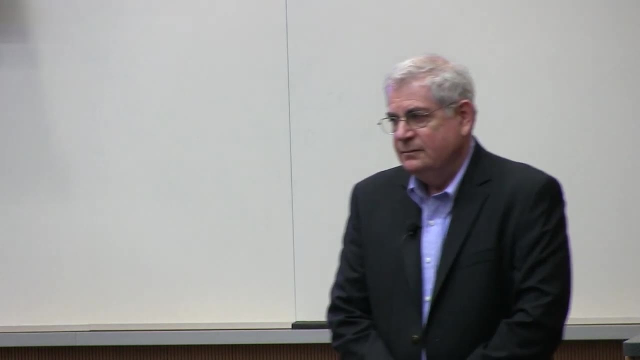 like increasing concentration of the oligosaccharide and how it affects the ability of growth and starting to inhibit the growth of the bacteria. No, didn't do that specifically. Didn't do that specifically, And that's, And that's.